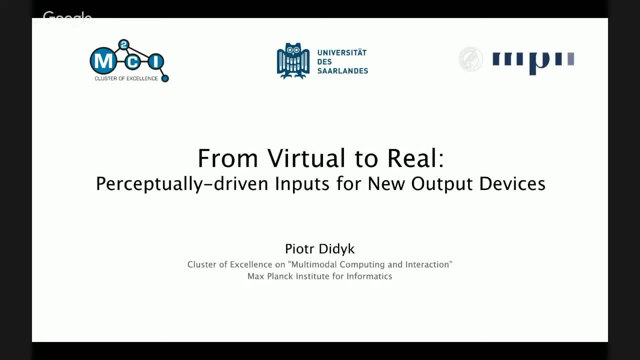 I think organizing this kind of talks is a really great idea, So it's really my pleasure to be here with you guys and whoever is watching this. So yeah, today I will talk a bit about my research. This talk will be more like overview of my approach to what I want to do, rather than specific projects and details. 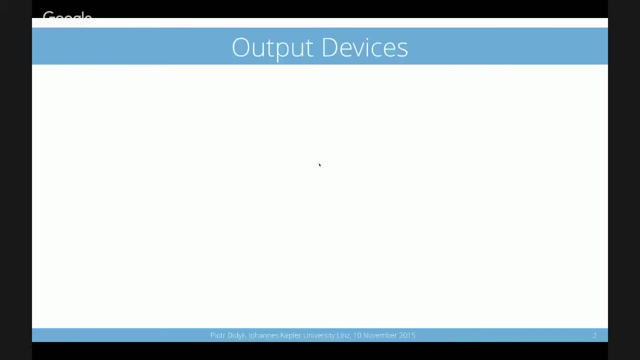 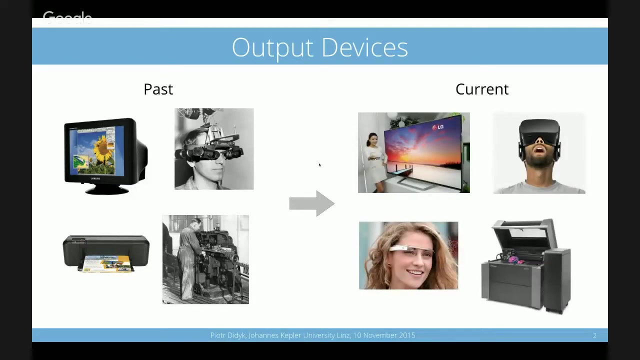 So, but yeah, anyway. so my research is essentially motivated by the recent development in many different kinds of output devices. So, as we can see, we, you know, currently we get a much bigger variety of those output devices. They are different in many ways. 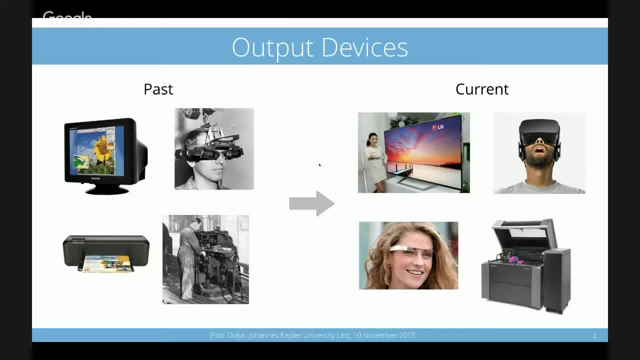 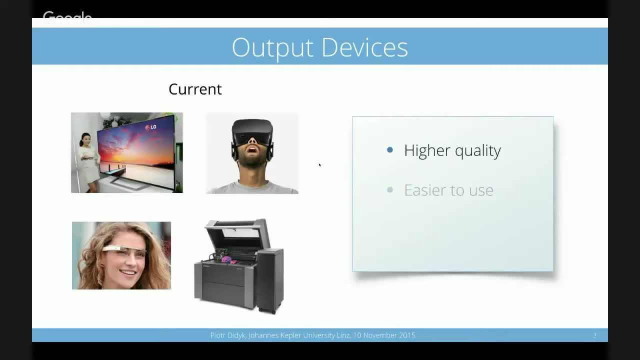 They have many aspects, But what is interesting is that there is really many of them and there are many differences in terms of capabilities. So if you look at them, we can, of course, reproduce much higher quality with current devices. They are much easier to use, but they also offer those new possibilities. 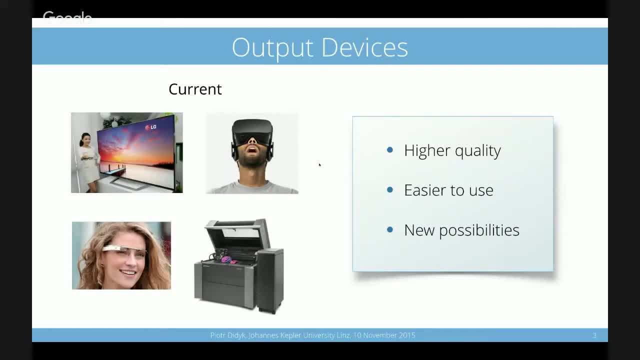 So, for example, this recently emerging market of 3D printers shows that we quickly move from 2D printing to 3D printing, And this really gives people, and even naive users, a great opportunity to create stuff and to bring this digital world into real world. 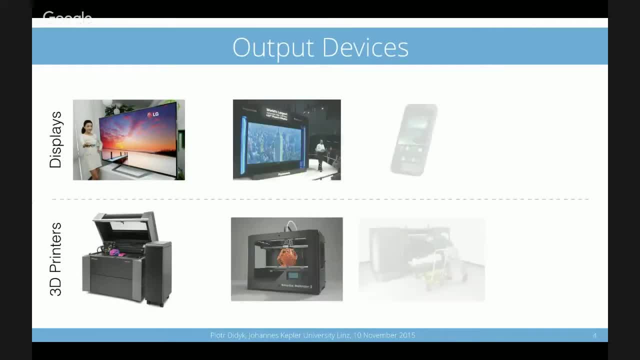 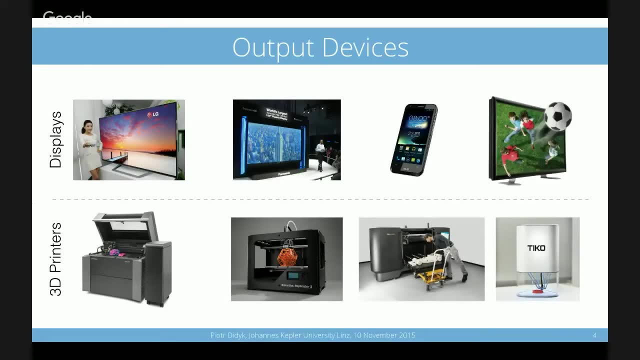 And even if we look at the specific kinds of devices, we'll see that within each class of this device there are many different subcategories or those devices different in different aspects. So, for example, in the context of this place, we have this place. 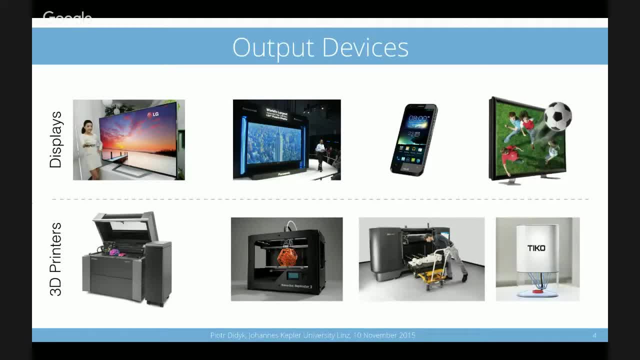 We have this place with different sizes, but also with different capabilities. For example, we have those multi-view screens, stereoscopic screens. In terms of 3D printers, we have printers that are customized for needs, also for the budget that we have. 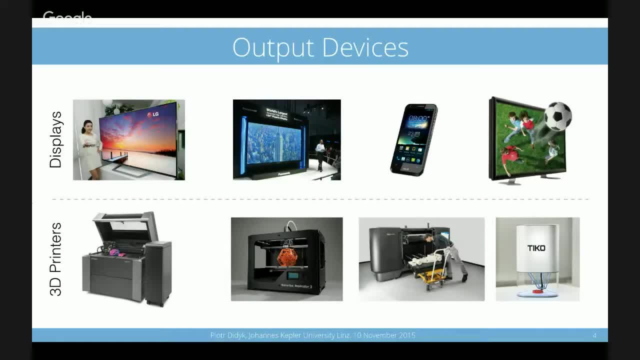 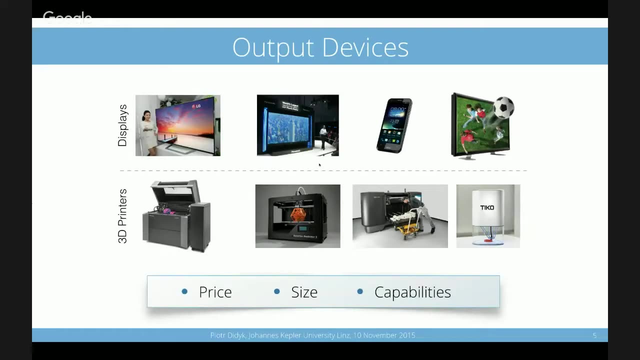 So we can buy low-price printers and print relatively simple things, But we can also buy those high-end, huge 3D printers that are able to do much more. Yeah, So those devices, they are different with different capabilities. So this is, I think, also different from what we observed in the past, that now we not only get better devices, but also the customization of those devices is pushed to much larger extent. 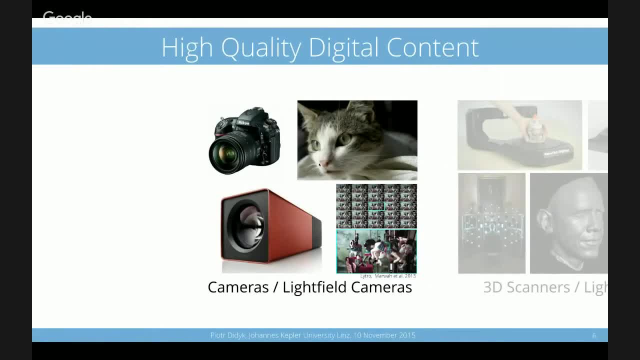 And, on the other hand, if you look from computer graphics side- not only computer graphics side, but in general- we learn how to capture real world. So, starting from images, we can take high resolution 2D images. But we also, for example, learn how to capture more complex data, for example light field. 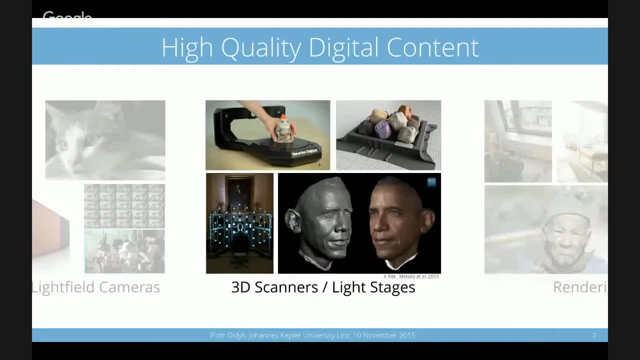 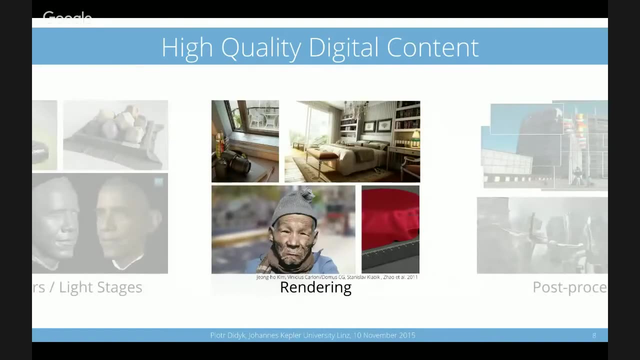 Besides this, we also learn how to capture 3D information of surrounding thus world, including also reflectance properties, And those two sources they let us we actually use in computer graphics And those let us render, for example, super realistic images like those ones here. 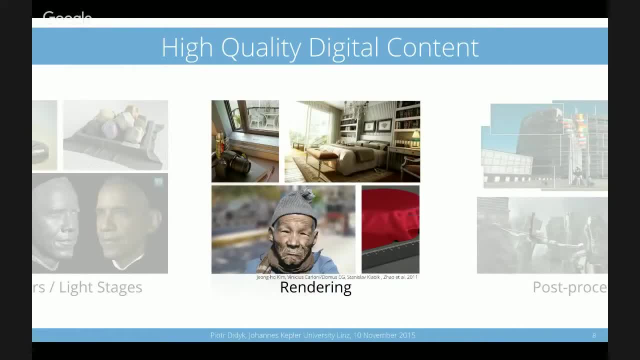 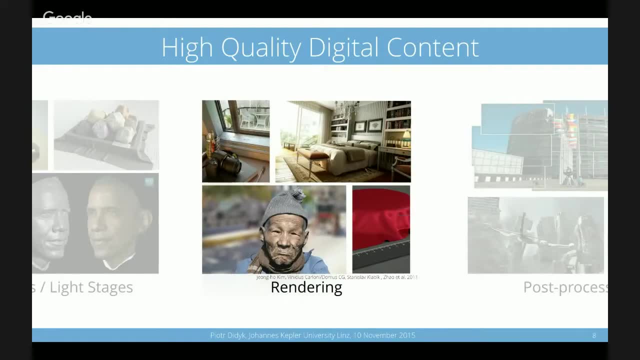 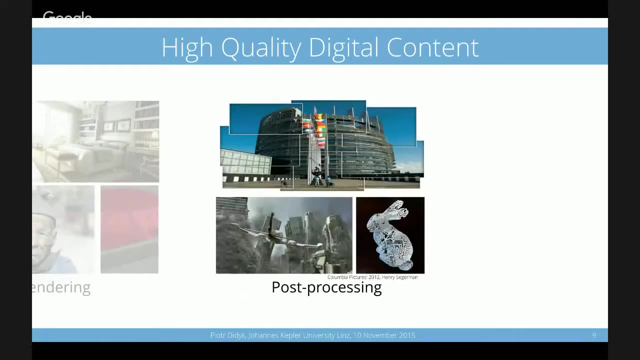 Where we cannot really distinguish- Yeah, Those renderings from regular images, And later, with this huge amount of content that we can capture, we also can process this content and create even more complex images and combinations, where we can go to gigapixels. photography. 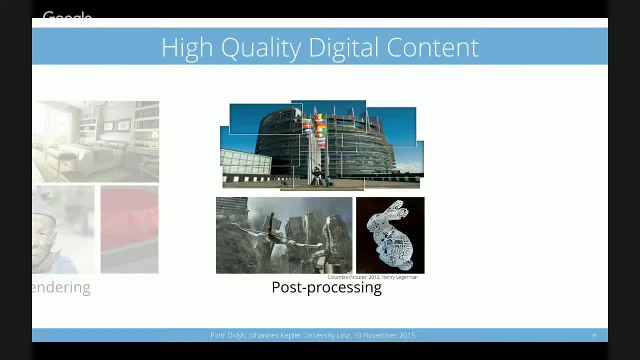 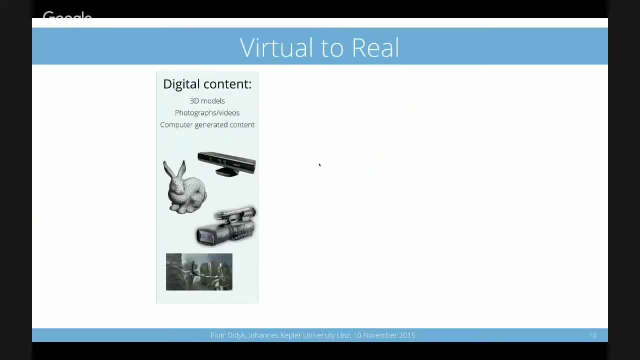 We can combine CG content with real content captured with cameras in the post-production tools for movie industry, Or we can create very complex geometries. So on one hand, we have those huge capabilities in terms of how we can capture the data from real world. 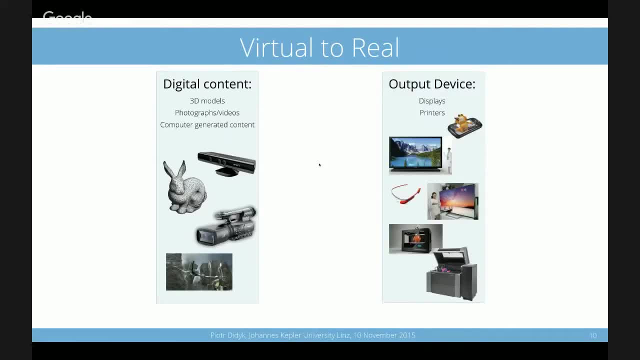 And, on the other hand, we have a number of those output devices. As I said, they are different in many aspects, And what is really interesting for me is how to actually take this digital content that we capture, we post-process And we organize it. 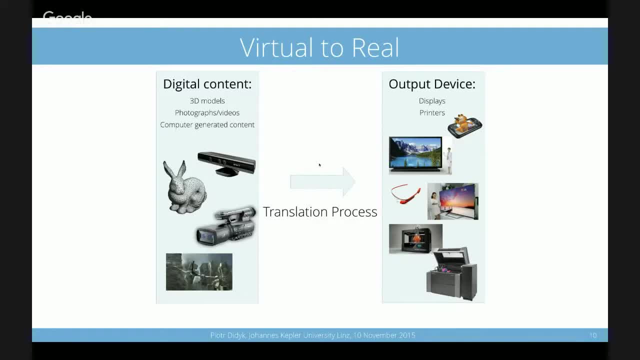 And we obtain via different processes, And we use this to show this information on those different kinds of output devices, such as displays or maybe 3D printers. So in my research this is maybe not really super accurate, But for me I usually assume that we have an almost unlimited capabilities in terms of what we can capture. 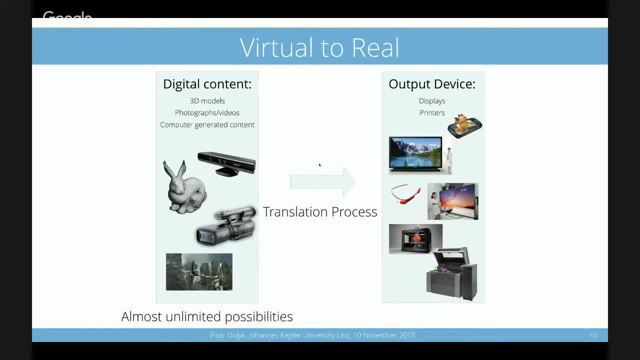 Of course this is not true if we talk to people that do rendering. Of course there are time constraints. We cannot render everything, But in theory, when we let those processes take long time, we can really currently capture really a lot of data. 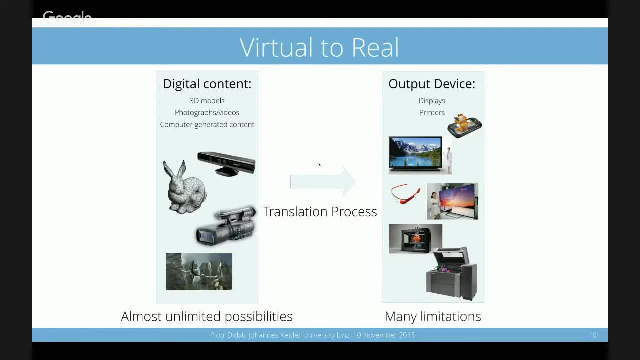 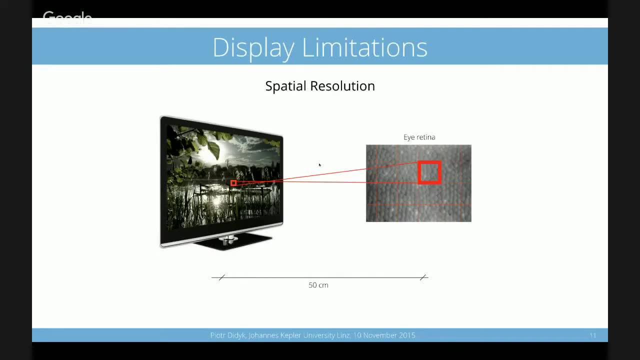 But on the other hand, on the output devices side, we have many different limitations, And what I mean by those limitations is, for example, the limitation in the display resolution. So if we think about it and we take a closer look, if we look, for example, at one pixel, 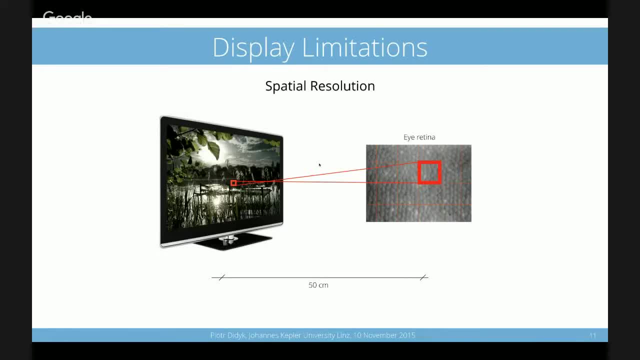 that those displays are composed of and we look how this display patch projects on our retina, we'll quickly realize that the area that one pixel is covering on our retina is actually containing more than one photoreceptor. So there is approximately 9 to 12 photoreceptors. that corresponds to high-definition screen. 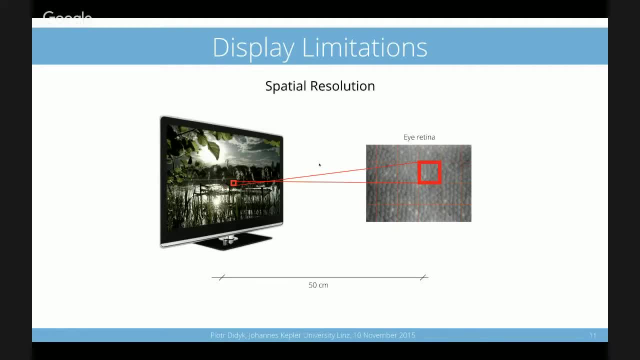 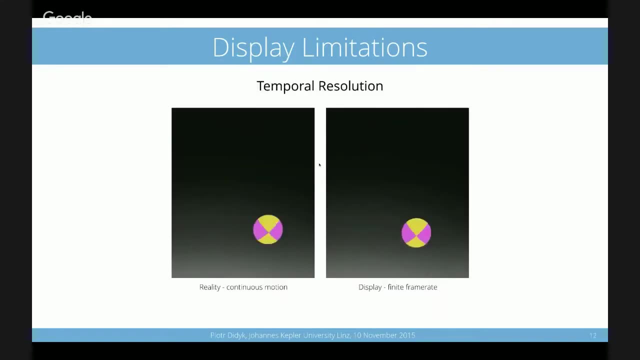 which is less 50 centimeters. So this kind of gives us the idea that, although we can capture those high-resolution images, when it comes to display, those displays are really limited and they cannot really address individual photoreceptors. Another example of the display limitation is, for example, the temporal resolution. 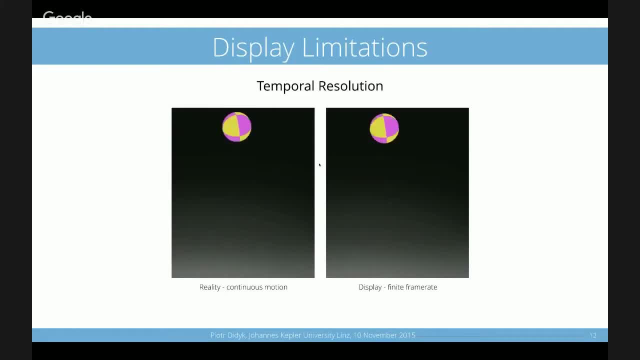 So in real world we are used to observing continuous motion and we observe it in continuous ways so we can track those objects and make this object steady with respect to our retina When our fovea, so we see those objects sharp. 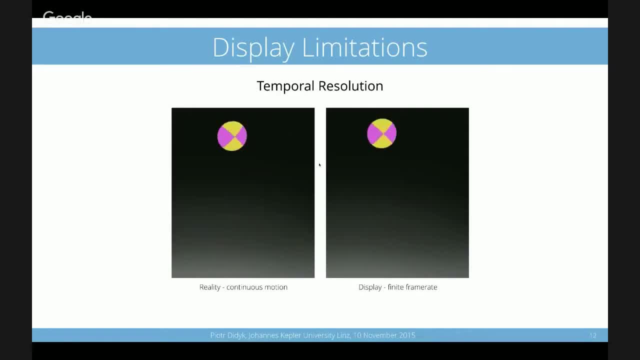 However, in the context of display, those devices have rather limited temporal resolution and this leads to many effects such as whole tabular or jagginess of the motion and so on. So again, we have currently high frame rate cameras or we can render high frame rate content. 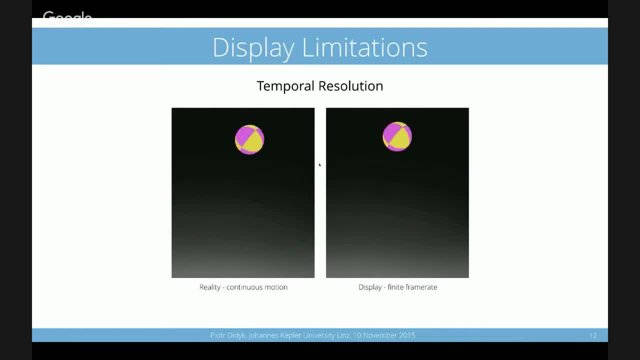 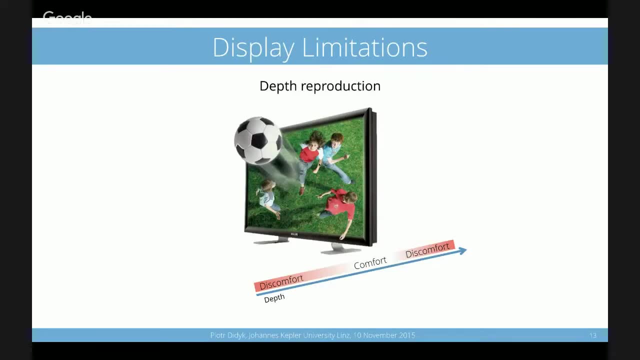 but we cannot really display those things on current devices. In the context of 3D screens, there is this known limitation that we cannot reproduce a huge depth range that we might want to capture, but we usually have to squeeze the 3D scene. 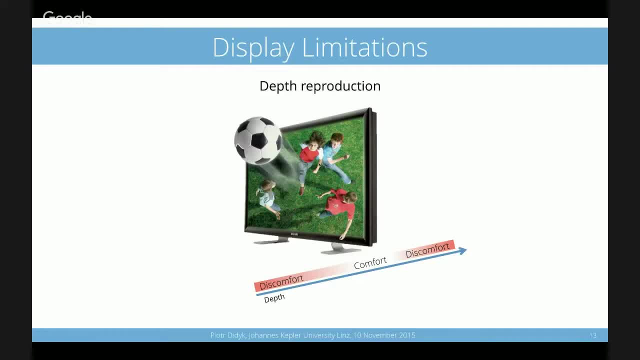 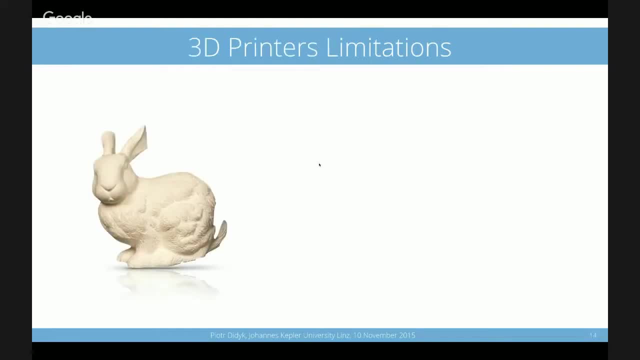 or the stereoscopic content that we show on the screen to some smaller depth range in order to make the content comfortable. And, last but not least, in context of the 3D printers, if we want to print some object- almost never if we use current printers- we get what we want- 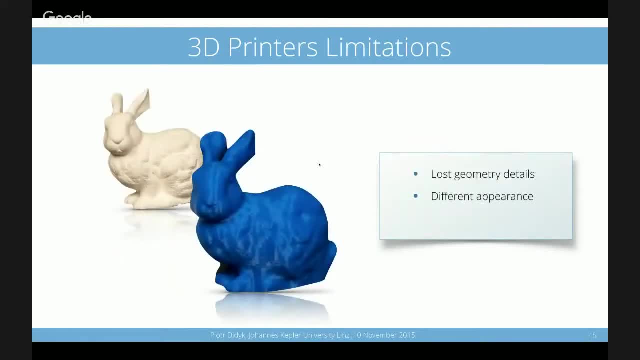 And those differences are. there's a lot of differences in appearance, so the resolution of current printers is not high, so we have lost geometry. We have slightly different appearance because the number of materials that we can use is currently limited. But there is also something more that we maybe cannot see, and this is beyond what perception in computer graphics. 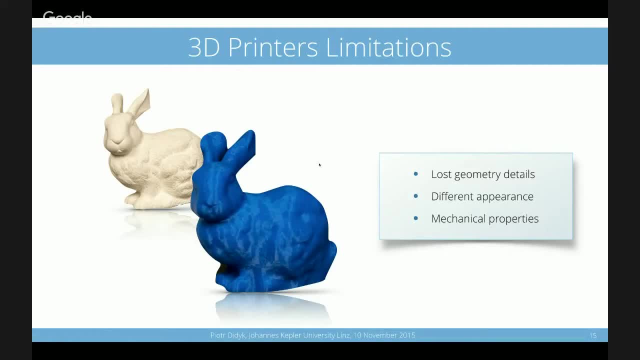 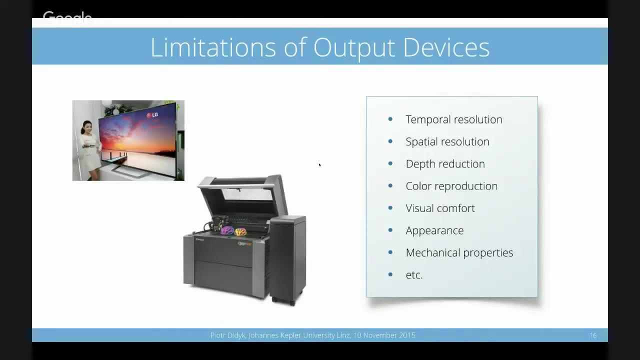 has considered so far, those are mechanical properties. So because we have a limited number of materials, we cannot really reproduce all mechanical properties that we might want to convey. So, in summary, no matter what kind of device or the output device we are using, 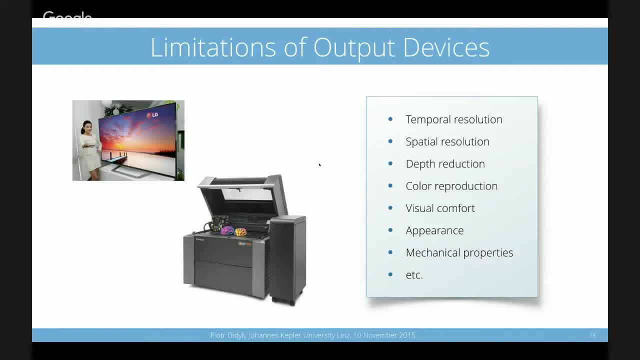 and no matter how much better they will get, I believe that there will be always this gap between the content that we can create and content that we can reproduce, And there is a really extensive list of limitations that those devices have, starting from spatial temporal resolution, depth reproduction- as I said for 3D- and auto-multiscopic screen. 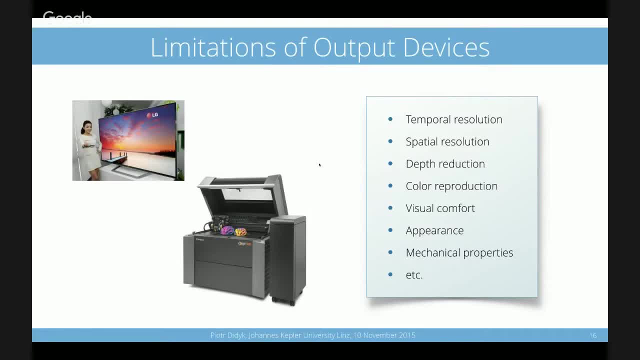 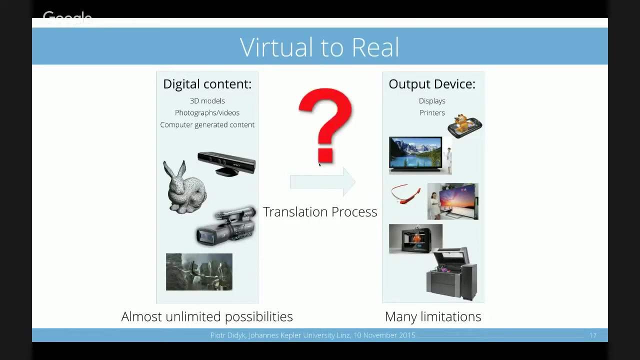 And there is a lot of things that is now coming up due to the 3D printing technology and how it actually reproduces the complex three-dimensional objects so they actually look and feel plausible. So really, the question is how to do this translation process. 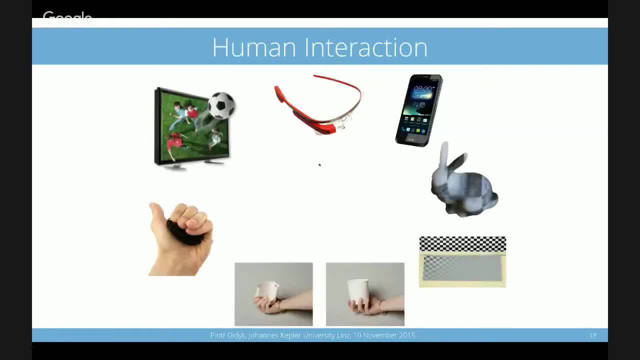 But there is this one more thing that I talked about already and mentioned a bit. There is no matter what kind of objects we are going to reproduce, most of them- not all of them, but most of them- will include some- will involve some human interaction. 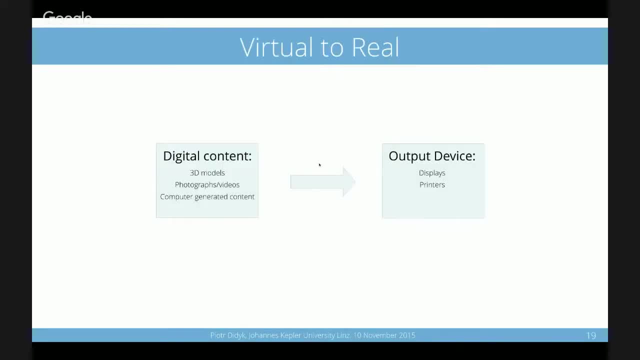 So what I tried to address also in my research, is to take this into account. So I try to remember that whenever we do this translation process from digital content to output devices, there is at the end a human observer and a human sensory system that is involved in the perception. 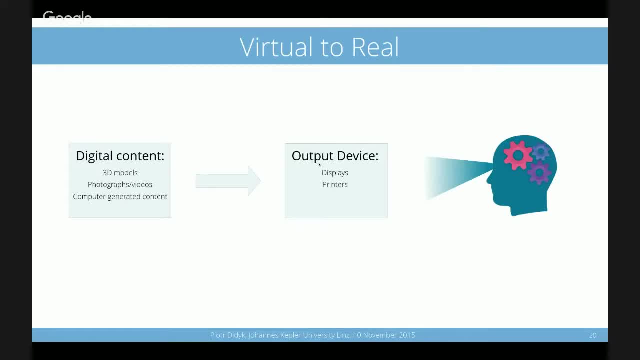 of those objects, of this content that we are creating And, as I mentioned, there are those limitations on the output devices side, but there are also many limitations on the side of human sensory system. And just again to give you an example, 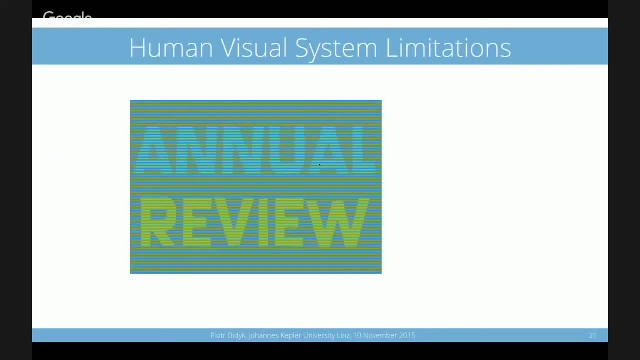 if you just brief idea what those are is, for example, here there is a limitation of the human visual system to the color perception. So if you look at this image and I ask you what kind of colors I use for reproducing those two words, 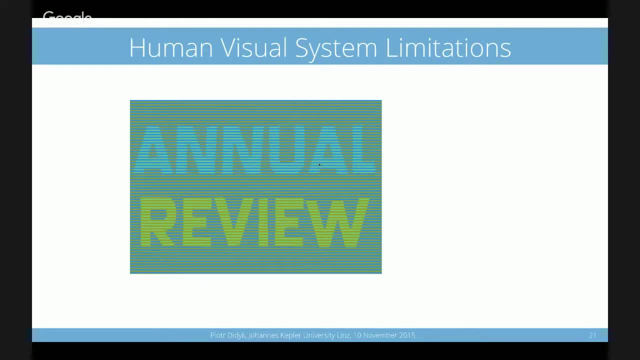 you will likely say that the one on the top is blue and the other is on the bottom is green, But in fact, if you look closely, those two colors that I use for actually creating those two words- they're exactly the same. 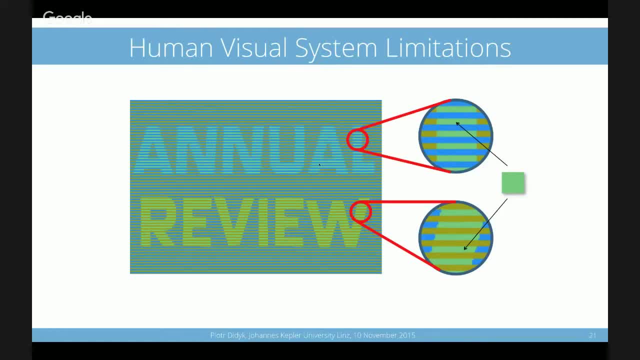 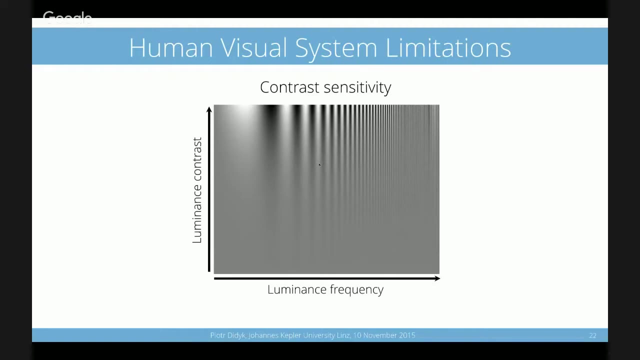 So this kind of shows that we are often fooled by our perception and very often what we actually see is not what we actually get in the real world. The other very frequently used properties of the human visual system is so-called contrast sensitivity function, which essentially characterize which kind of patterns we see. 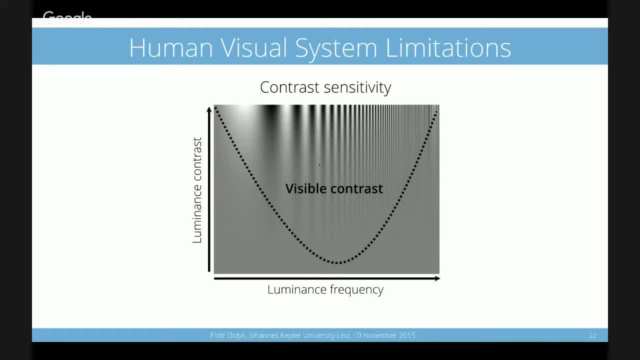 or which kind of patterns we don't see, And this is related to the contrast, to the magnitude of the contrast and frequencies of the contrast, And many of the techniques for preparing content for displays actually rely on those findings about the contrast sensitivity function. 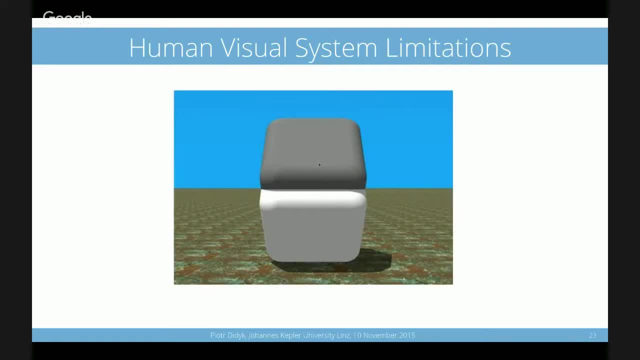 And on top of it there are also many illusions. So, for example- this is a standard illusion that's often shown- There are those two blocks on top of each other, And if I ask you what color are these or what gray value are these? 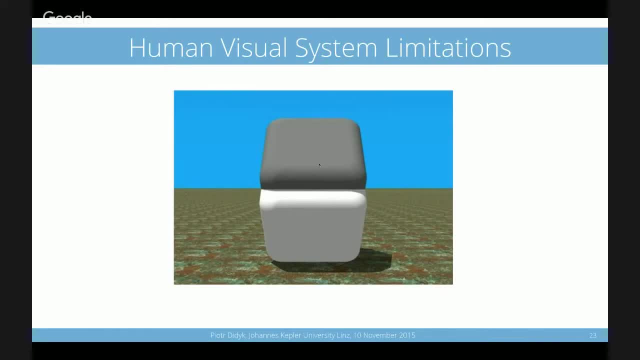 you will likely say the lower one is much brighter than the one in the top. In fact, however, when you cover the transition between those colors, you will quickly realize that those two colors are the same. So again, the main message here is that human visual system. 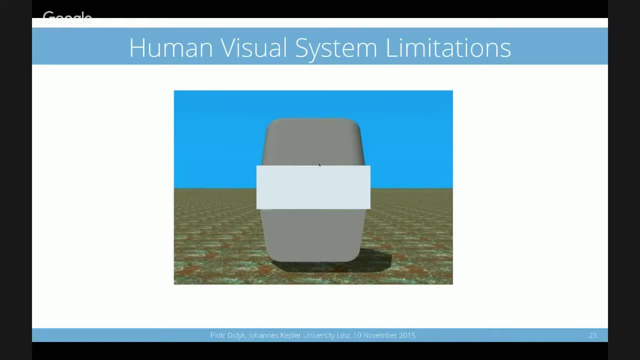 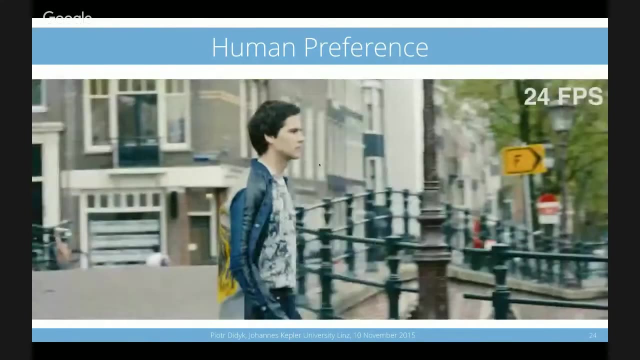 and not only human visual system, but in general sensory system, has many limitations, And what we see, what we perceive, often is different from what actually is reproduced. There's also one more thing that I want to mention. There's a human preference, So in many aspects the human preference plays a big role. 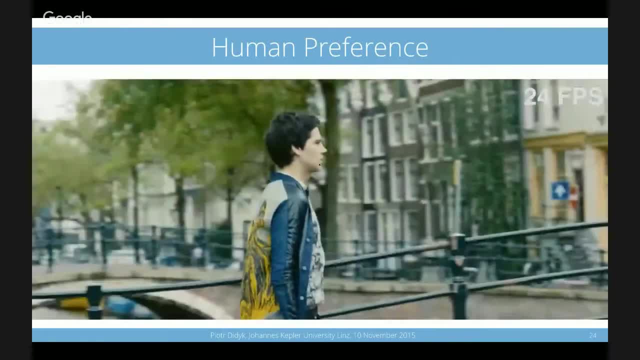 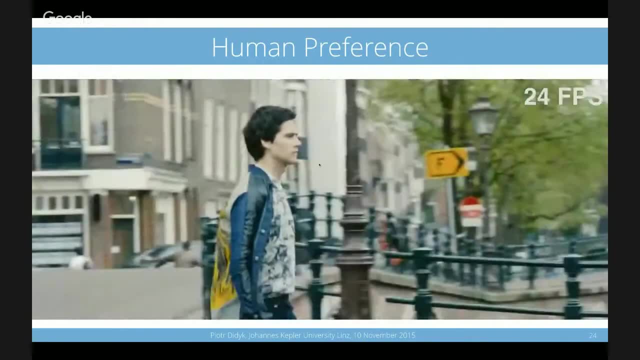 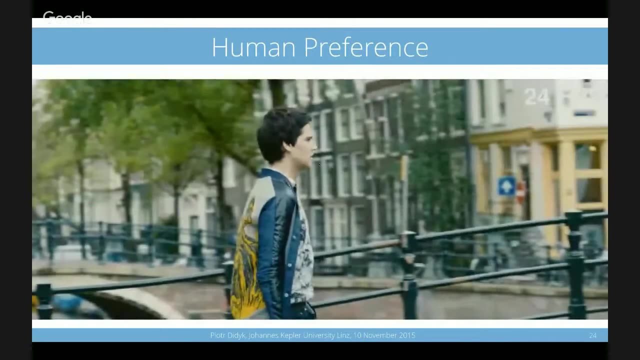 And recently- just recently- there was a huge debate- I mean there is still a huge debate- about the frame rate, because there were new movies released in high frame rate And you can create a movie in 20 frames for four frames per second. 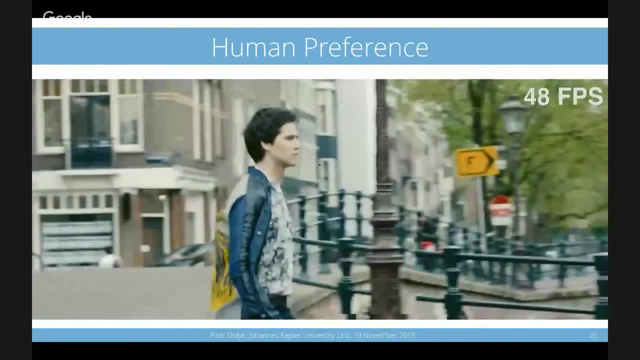 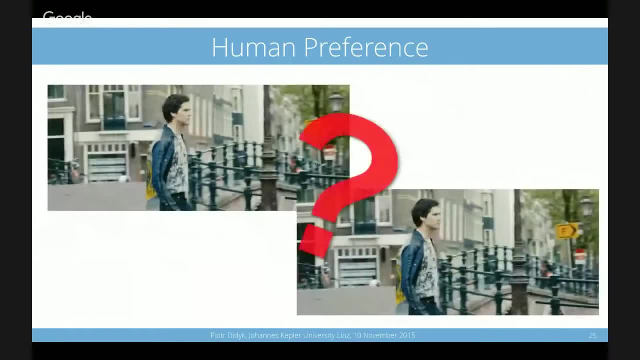 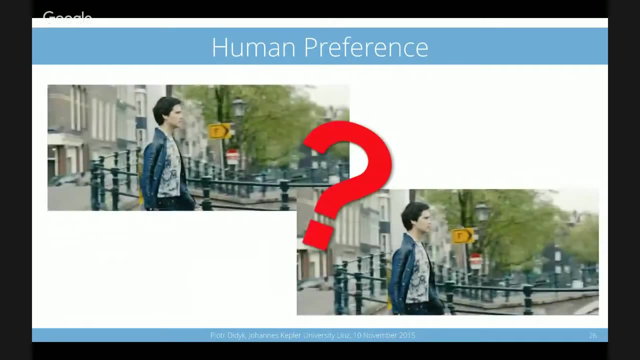 And you can. I'm not sure whether you see it. This is 48 frames per second. Probably you don't see it, But anyway, there is the debate. Of course 48 frames per second is closer to reality, But at the end, what people want to see, it's not really clear. 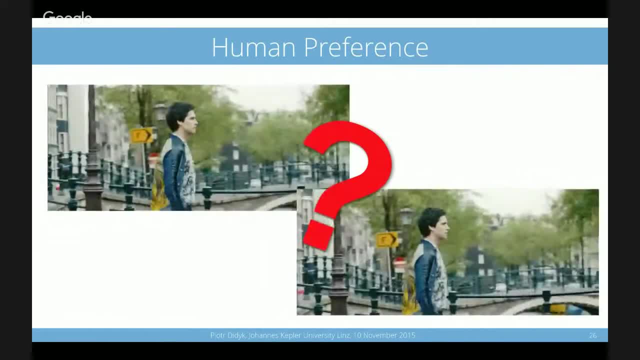 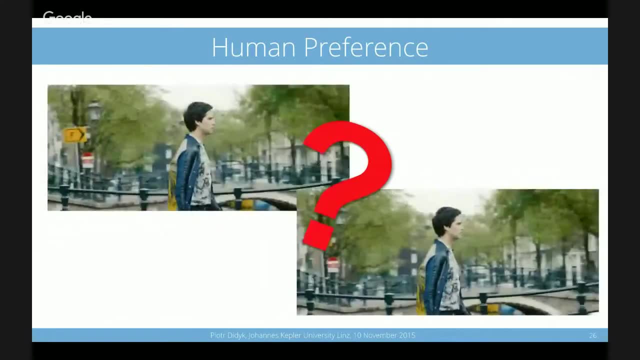 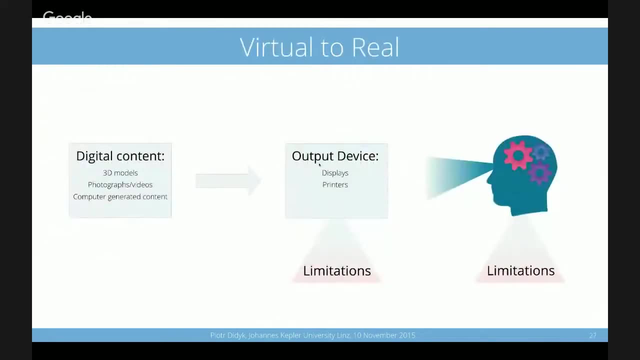 Some people want 24.. Some people want to 48. So really it's first thing is about the limitations of the human visual system, But then at the end you need to also take into consideration what actually people want to see. So yeah, so there are those limitations. 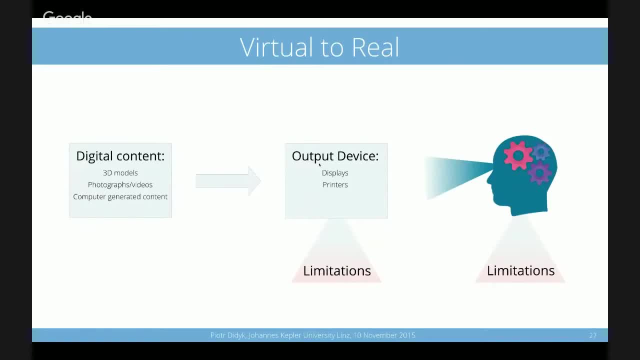 on the human sensory system, And what is interesting here is the limitations on the human sensory system and the limitations on the output devices side. they are usually not the same, And there is the place where we can play a game and try to trade those limitations. 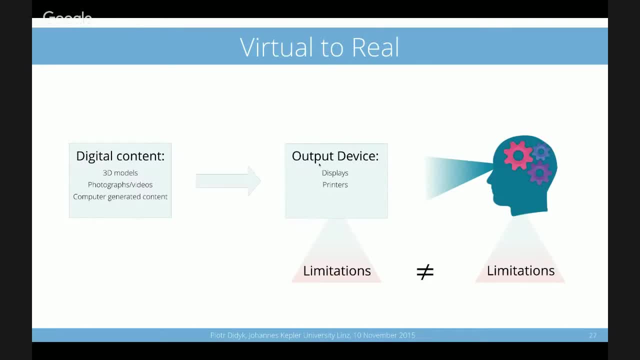 so we can use certain limitations on the human sensory system and use them in a favor to improve the perceived quality on the output devices. And this is essentially what I would like to show you now, And the standard way of doing this, and the approach that we are trying to do, is to learn something. 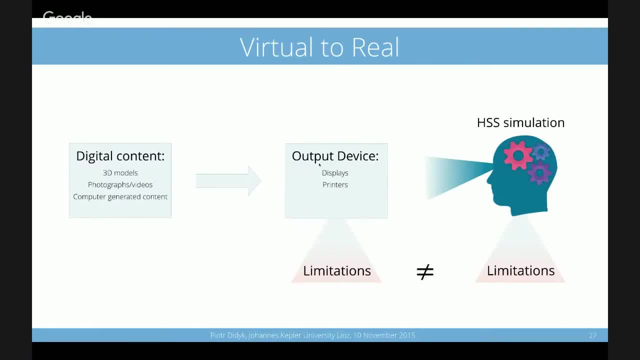 about the human sensory system. Simply speaking, we may say that we want to, to some extent, simulate it. We want to simulate the human sensory system, build models of them to understand how it works, And then we want to include those models into. 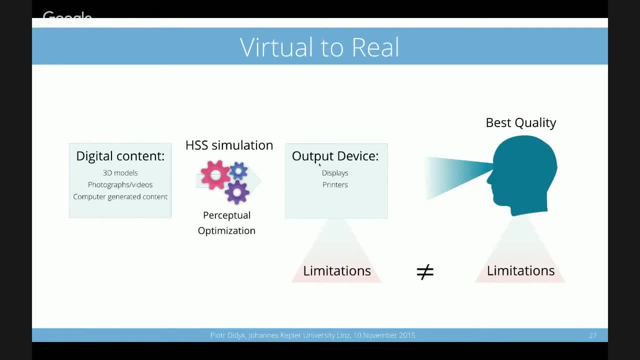 so what we call perceptual optimization, which essentially is translating this digital content into output devices, and try to optimize for the best quality, but not for the best quality as can be measured on output devices, for example on screen, but as measured as a perceived quality observed. 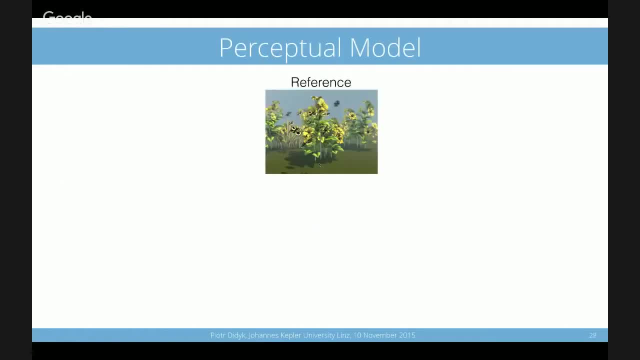 by the human observer And the standard, the way such a perceptual model works and how what can be a simple task that such a model should be able to do is essentially if we have, for example, in context of displays, if we have a reference image that we want to show. 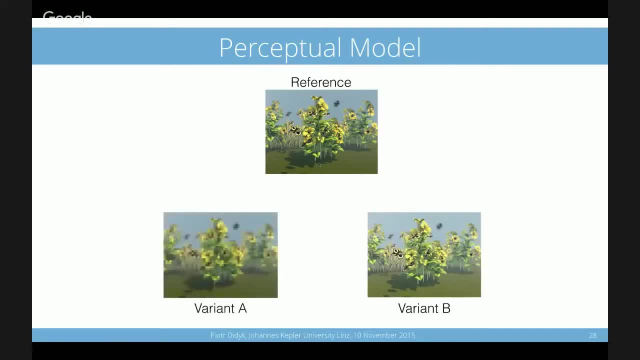 on the screen and we have certain display limitations that cannot really, which doesn't allow, which do not allow us to show this image on the screen, And we have two, two instances, so to say, of this image that can be actually presented on the screen. 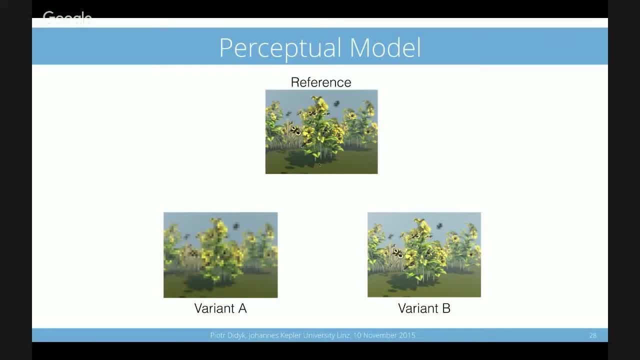 We want to essentially be able to judge which one, which one, will be closer to the reference, And of course we can use a standard numerical differences. but it turns out that those numerical differences very often do not meet the values, The values that are actually reported from the people. 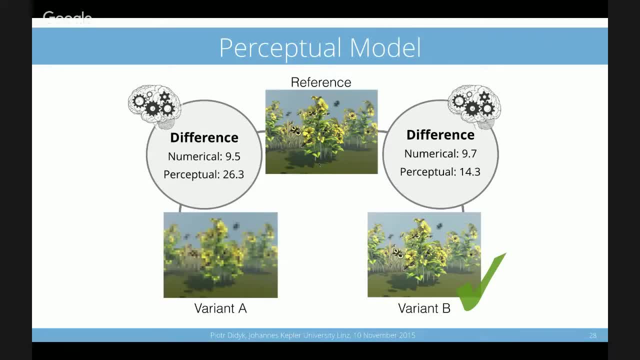 So here, maybe if in the variant B we just reduce brightness slightly, increase the brightness slightly in the terms of numerical difference, it can have a very similar impact as, for example, reducing the resolution. But in fact people are not that sensitive. 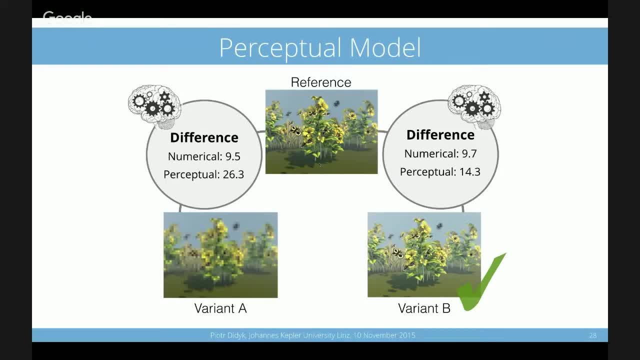 to the luminance changes. Therefore, this numerical difference here doesn't really doesn't really simulate the perceived difference really well. So in this case we would just like to tell which variant, A and B, is better, And this is one of the tasks that such perceptual modeling. 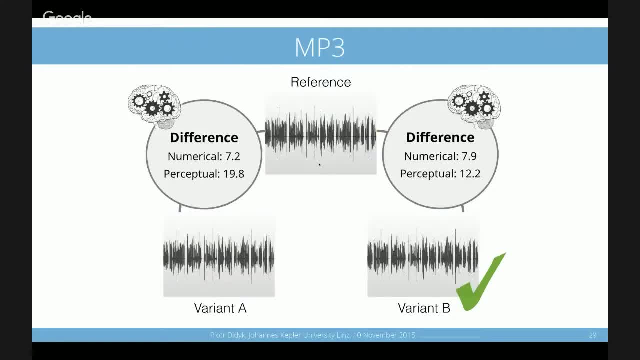 should be able to do And, if we think about it, such models are really in the heart of many things that we are using currently. So, for example, MP3 codec. what really has insights, it's some model that essentially tells which of the signal will be heard by a person. 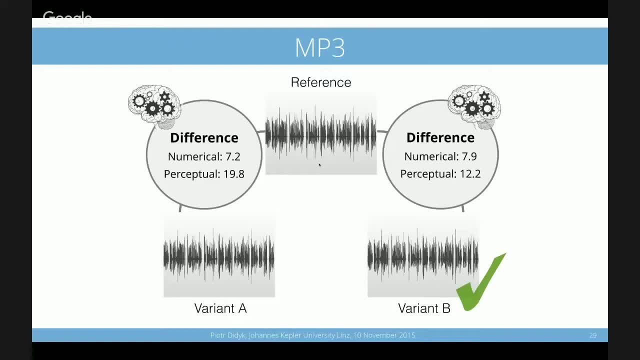 and which will be not heard, And then, based on this, we can remove the information that will be not relevant for human sensory system And therefore we can compress this information and make use of such things. And yet, just to mention this again, 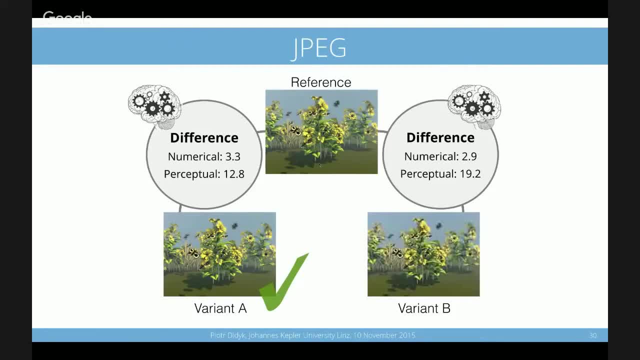 the same things happen in JPEG. Deep down in the JPEG, the JPEG compression, we have a model that can tell which things we will see and which will be not perceived. So it's really about telling the differences between two images and saying yes. 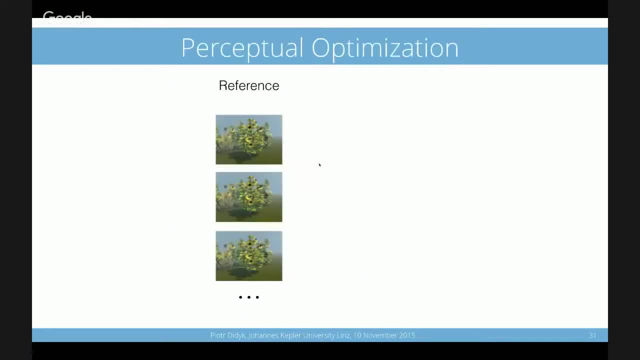 what will be visible or not. And then, if we have such a model and we want to do this perceptual optimization, we can do it very naively. So we have a reference image that we want to display, and then we have a number. 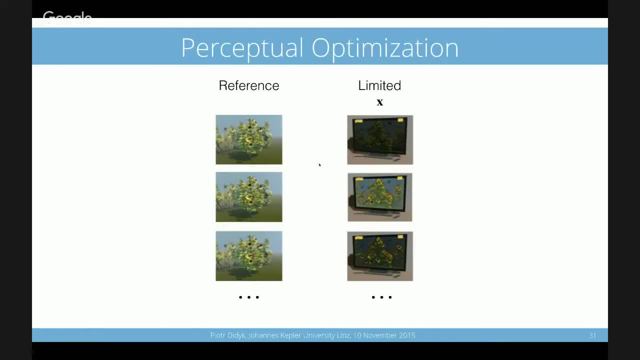 of different variants of images that we are able actually to display on the screens And if we have this model that can predict those differences, we can simply compute those differences and run some optimization method which can choose the image that best reproduces the reference image. 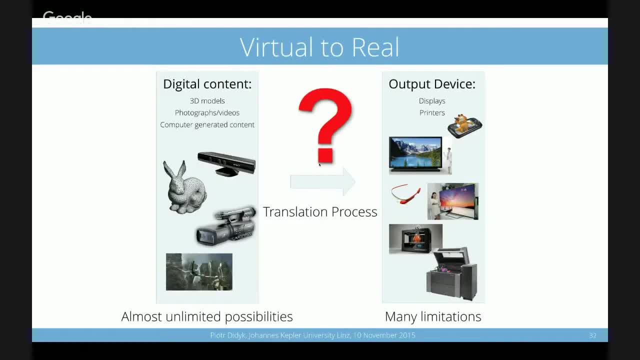 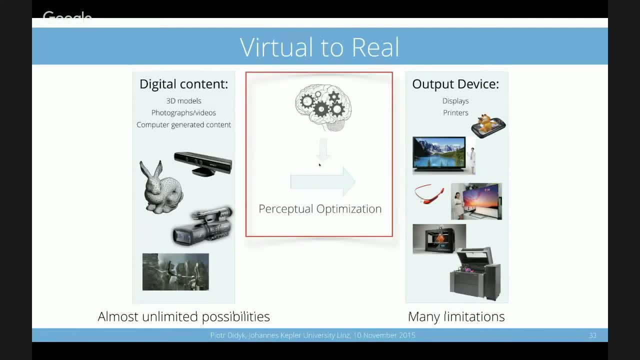 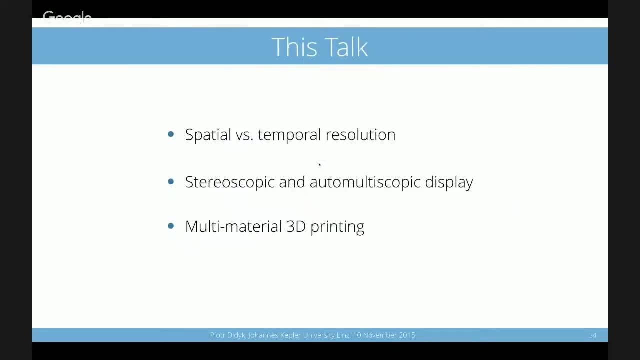 in the perceptual sense. So really, what we are talking here is this translation process, which is governed by this process of perceptual optimization and by the knowledge of the human visual system. So now I will just give you, I would like to give you- a quick overview. 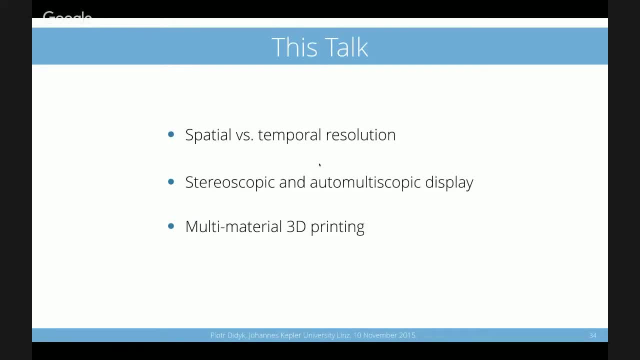 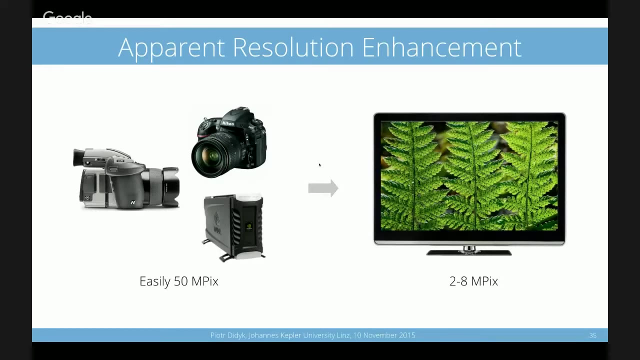 of three examples where we use actually such approach and it was successful in doing so. So first I will talk about the spatial and temporal resolution And in this context we had a project where we wanted to address the problem of limited resolution of display devices. 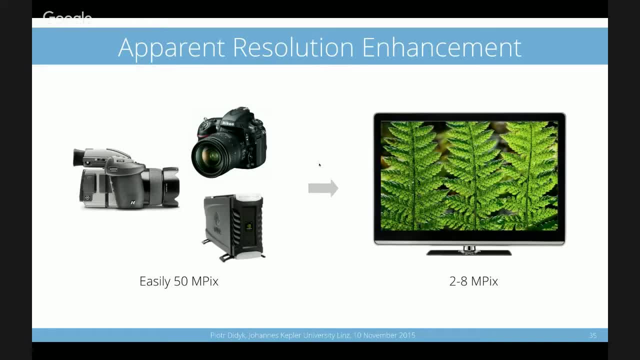 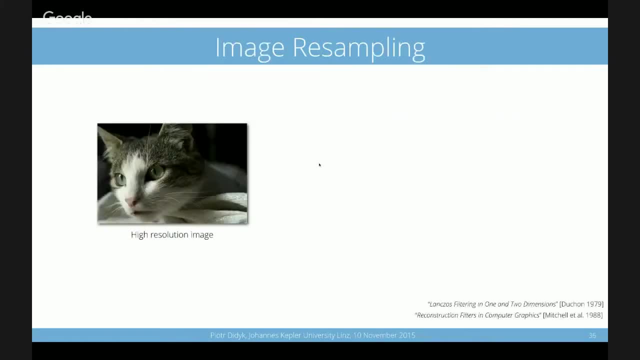 So, as I said before, we can capture high resolution content but we cannot really display it well on the screen. So usually what we do, we take high resolution image, then we have to filter out the information, meaning here high frequency information that we cannot reproduce on the screen. 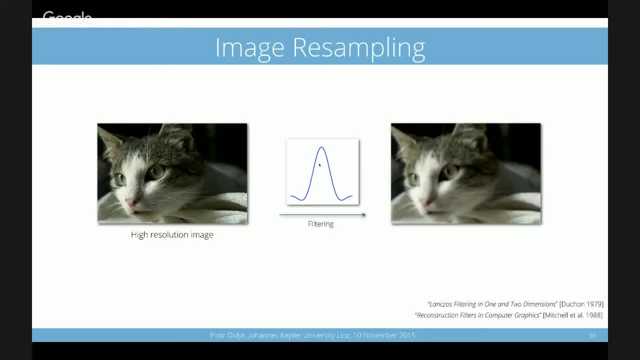 So we get kind of blurry image, blurry version of this image, and then we down sample this image And then now we are able to show this image on the screen. But, as I was already mentioned before, this is a pity, because if we look at the screen, 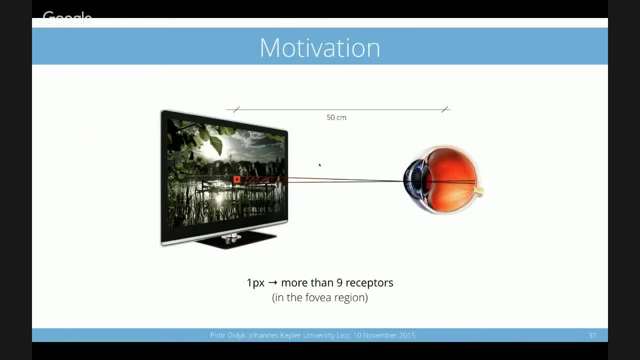 there are really many receptors that are looking at the same pixels in standard setup, So there could be really a hope that if we have high resolution displays, there would be a way to convey more information and to address individually larger number of photoreceptors. 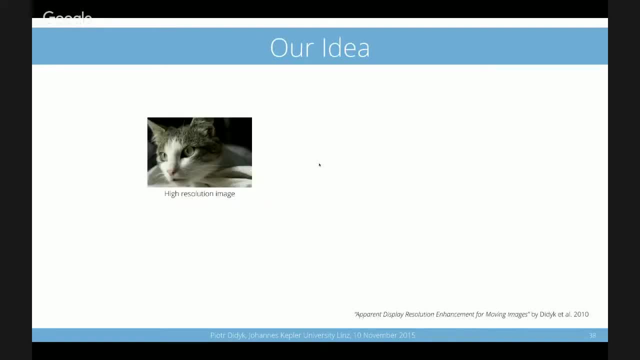 So what we wanted to do in this project is essentially to take high resolution image and then do something to it that, when we show it on the screen, it actually creates this impression of high resolution image. So we cannot really show the high resolution image on the screen. 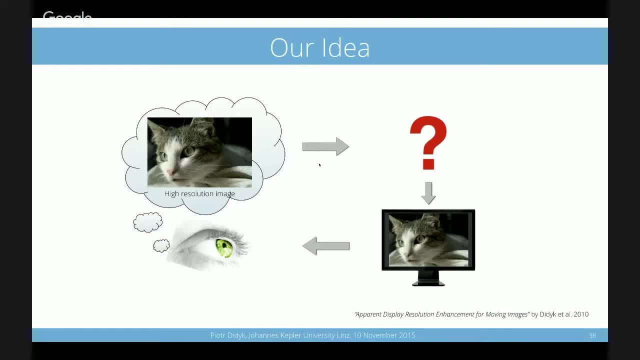 because it's low resolution device. But what we aim for is really this impression of high resolution image which is created at the end in our human visual system. And, in this context, what we did, we came up with this idea of decomposing the image. 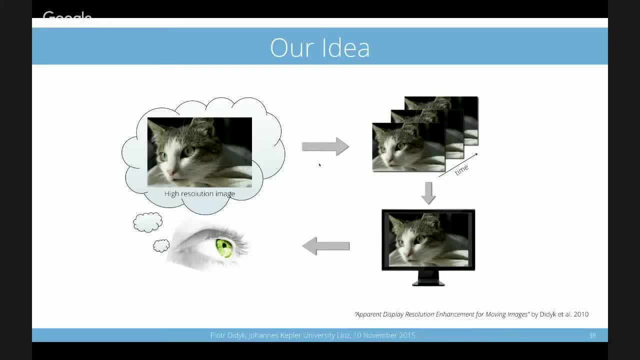 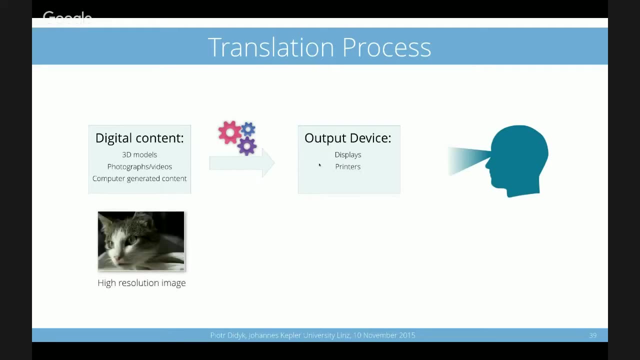 into multiple lower resolution images that are shown over time And we wanted to use here the temporal averaging that is done by the human visual system. So if we go back to the scheme of the translation process, essentially the input to our method is high resolution image. 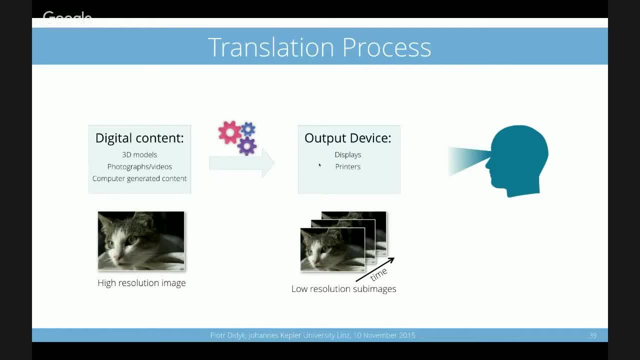 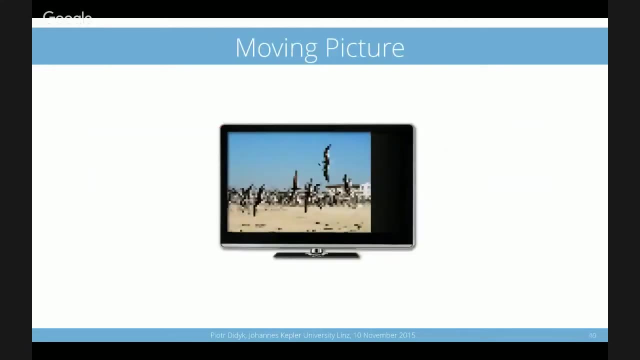 And then we want to, as an output, we want to have a number of low resolution sub images that we show on the screen, And what we want to account for is temporal integration done by the human visual system. So this method I would just here mention. 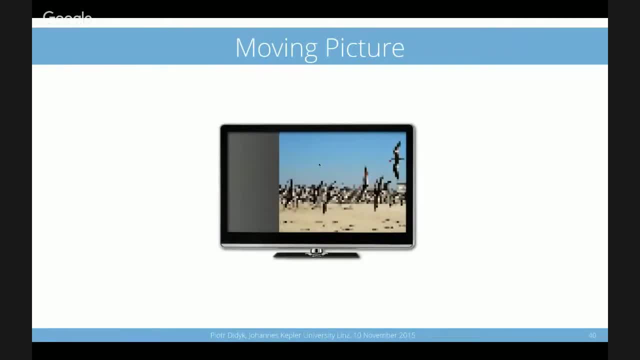 that this method works only when we deal with moving pictures. So if we consider only static images, this doesn't work. I will not go into details here, but yeah, it works only for moving images, because only then you can play such tricks as we do. 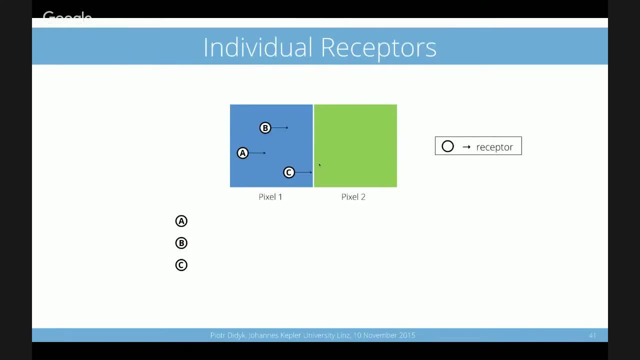 So just to explain you how it works it's, let us consider those two pixels and three photoreceptors that are looking at those pixels. So now, if we change the content, if we change the content that is displayed on the screen, but at the same time, 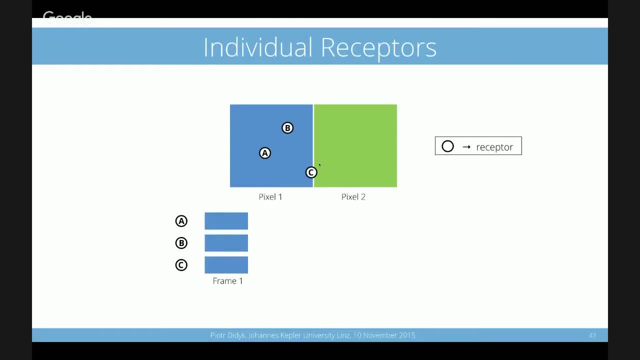 the content is moving on the screen, so we have some motion. our human visual system is well trained to track the object that is moving on the screen. So if we show a moving object, essentially what will happen is that the values of the pixels will change. 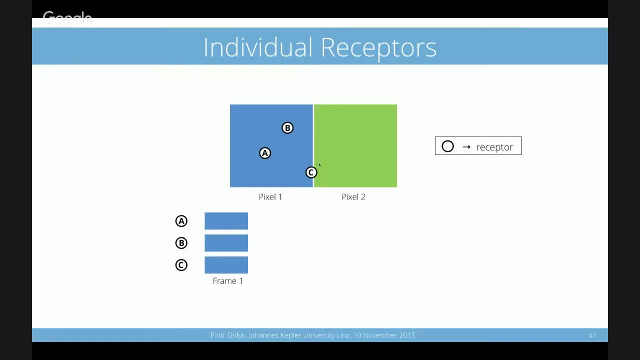 but also the positions of those receptors will change with respect to the initial position. So, as we can see here, if the object is moving I can change the signal that is shown on those pixels and at the same time I can move my photoreceptors. 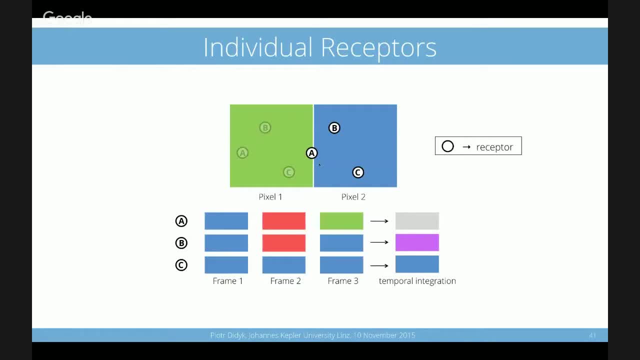 And now the interesting observation is that if those receptors were not moving, so if they were static, no matter what kind of signal I would show on the screen at the end, those three receptors that were falling in the same pixel, they would receive the same signal. 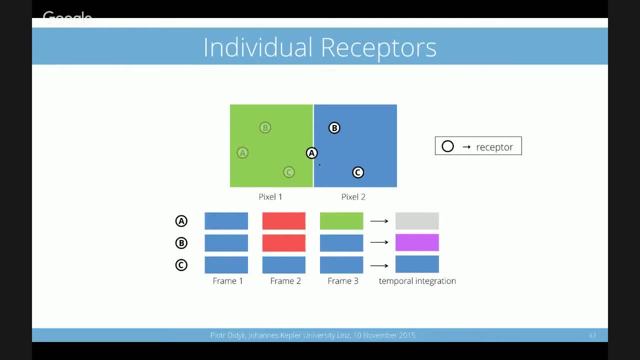 But here because they are moving and they cross the boundary of those pixels. actually we can address almost each receptor individually. So we can see that because those receptors see slightly different color over time, at the end of the cycle, what those color averages? 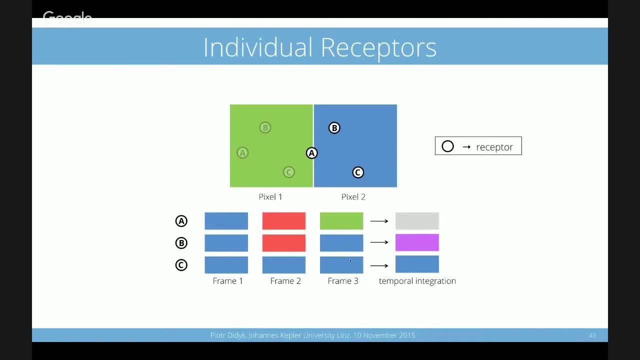 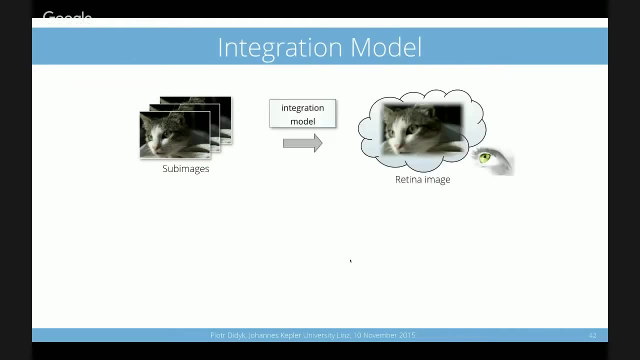 is slightly different. So this kind of shows that each of these photoreceptors can see something slightly different. And this was the motivation to our project and we formulated the problem as an optimization problem And first we created a model that essentially takes those sub-images. 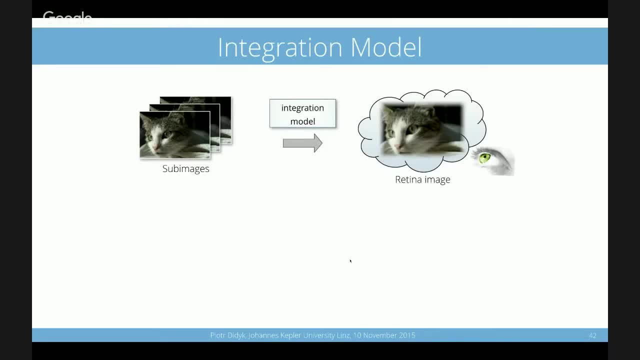 and the motion that we perform and builds an integration model that can predict the images actually perceived on the retina. So it takes into account the motion, it takes into account the sub-images and it predicts what we see after this temporal averaging of the human visual system is done. 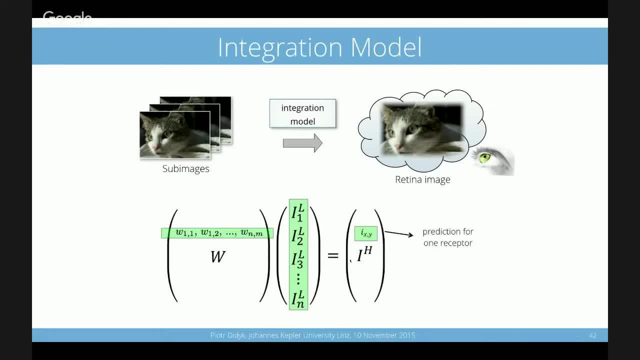 And now, if we have such a model, it turns out that this model can be easily written as a system of linear equation. So now, if we want to compute those sub-images that give us the impression of looking at high resolution, what we need to do? 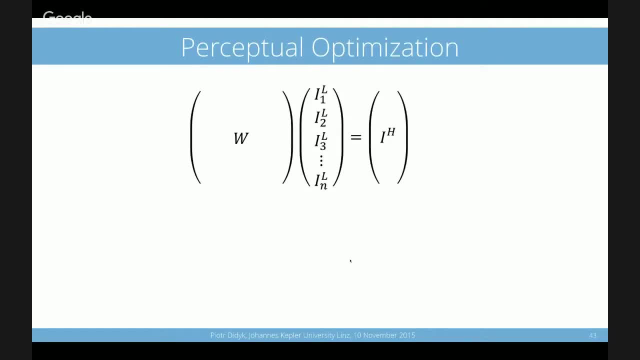 we have to turn this linear system of equation into optimization. So we give us as a matrix that describes this integration model. we essentially create this matrix using the information about the motion that we have in the scene To the right hand side. we just give this high resolution image. 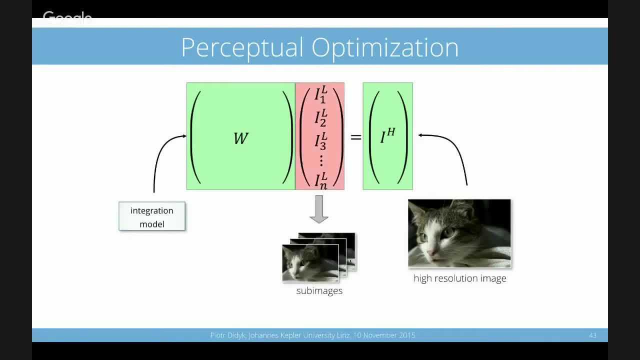 that we want to perceive and we simply optimize for those sub-images that we have to show that after the integration, they give us high resolution image And once we solve this we can, for example, obtain such a result. So those are three frames. 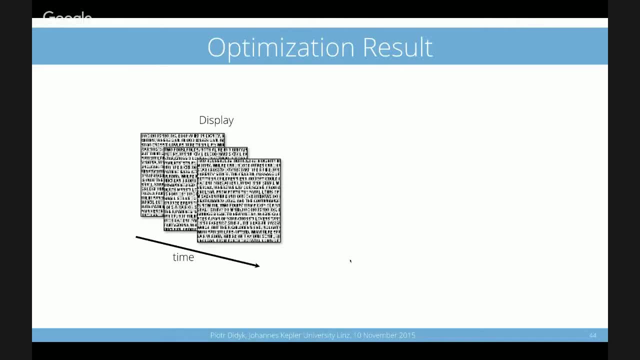 that we optimized, And you can see that each of this frame on its own doesn't convey any information. It's actually full of aliasing, but this is a good sign, because this aliasing actually is a source of high frequency information after this temporal averaging happens. 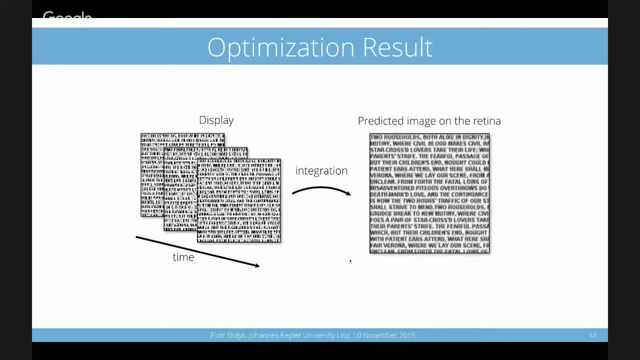 But what we simulate after showing those three frames on the screen, the rapid succession, what we actually can see is that those images average on our retina to something that actually we can read. So, although those three images don't convey any information, because the resolution 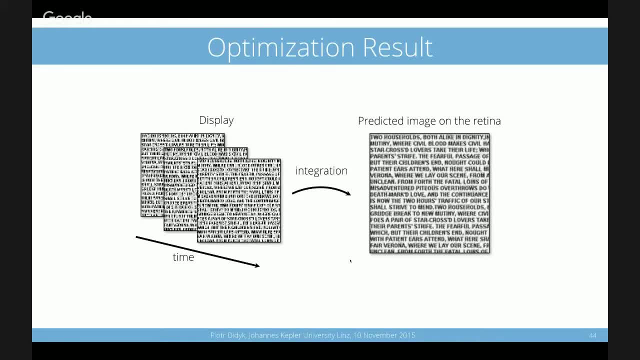 of those pictures is too low. after this temporal averaging, we actually can obtain high resolution that we perceive, actually high resolution image, that which we can perceive well, and we can actually read the text. And so this project was done some years ago and that there was some 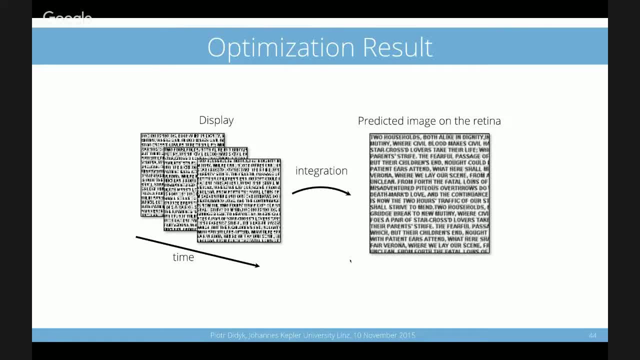 you know developments on the technology side And one can question: why do we need high resolution if we already such techniques, if we need, if we have already 8K display and we don't even have content for this? Well, the thing is that 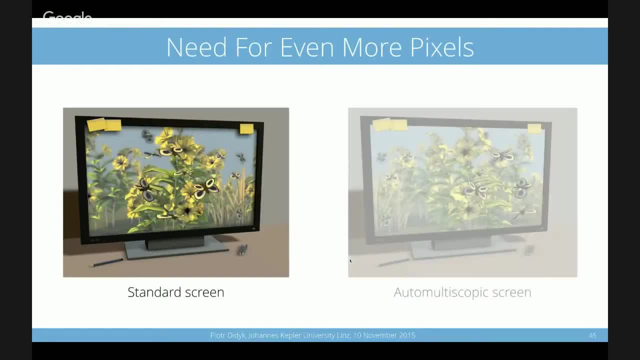 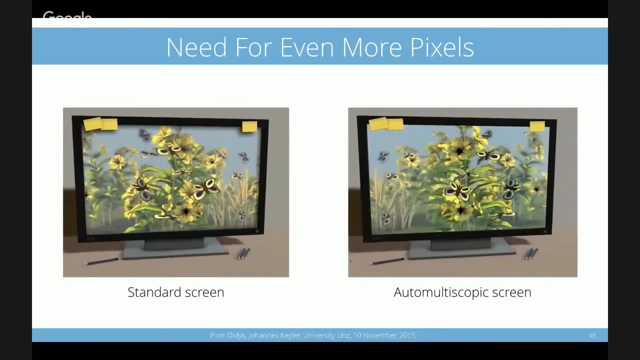 as soon as we will start moving from standard screen to something which is more light field screen. So, for example, nowadays we have those maybe not very common, but there are those auto-multiscopic screens which can show actually multiple views. Then we still 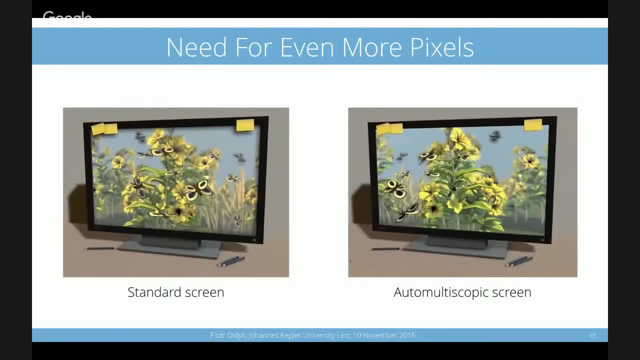 we are still lacking number for pixels to actually build those screens. So I believe, although maybe for the standard application, maybe one is right. It says that further improving the resolution is maybe not that important, because we have high resolution devices already and maybe 8K is ways too much. 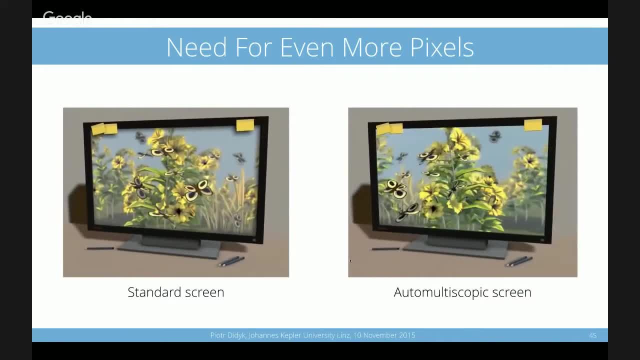 comparing to what we need. But if you think of those light field display, multi-view displays, those people that work on those displays, they still struggle with the fact that everything is low resolution, Even if you had, if you take head mounted displays. 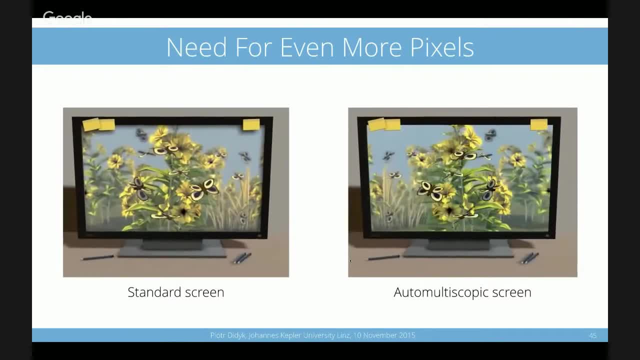 like Oculus Rift. if you put this high resolution screen in front of eyes, you quickly realize that the resolution that you need is not two times, it's not three times higher, but it's maybe 10 times higher that you actually need. So the such techniques. 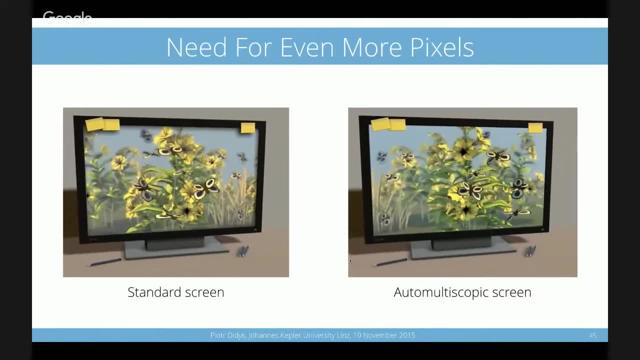 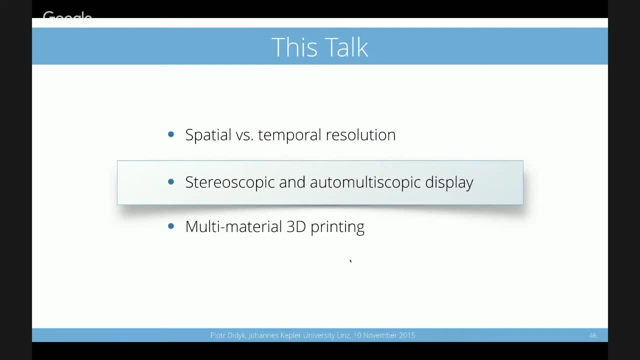 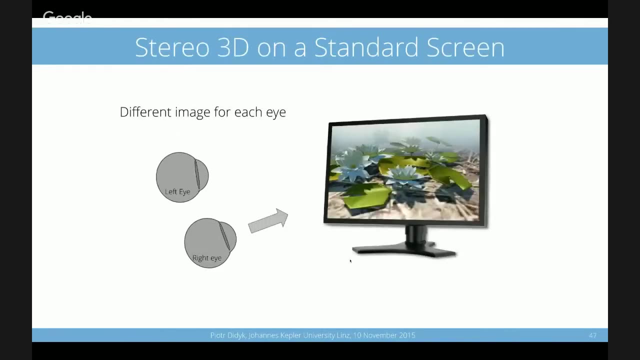 I believe will still find use in such context. Okay, so this brings us to the topic of stereoscopic and autostereoscopic displays, which I will talk about now. So, in the context of stereo, we show the stereoscopic images by showing two different images. 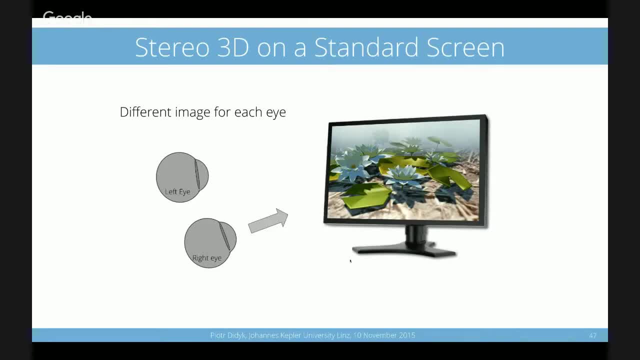 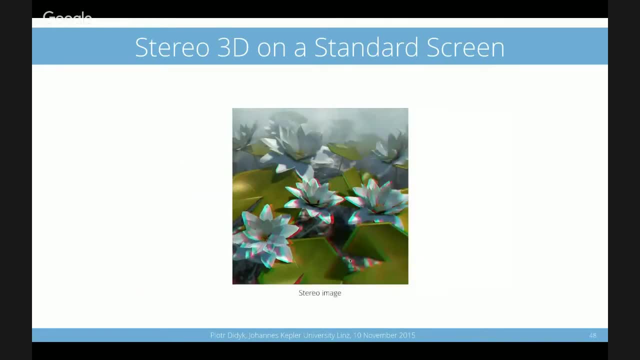 that are taken from two different viewing positions and we show them to left and right eye And the stereoscopic image is a symbol of the perspective that we have on the other side of the screen And the stereoscopic images are the same as the larger picture. 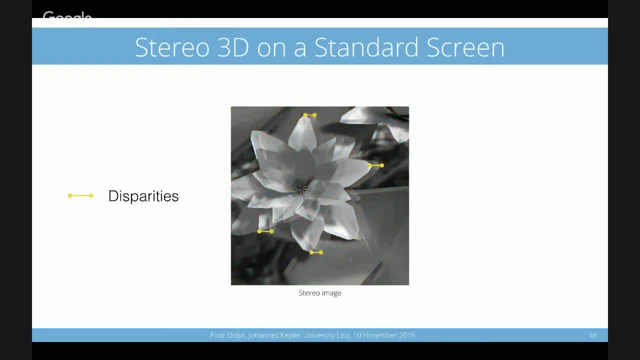 that we have on the other side of the screen, but they have a smaller representation, And the stereoscopic image is called the binocular disparity. So it's the binocular disparity that we have in both eyes. Now, the thing is that this is not the only source. 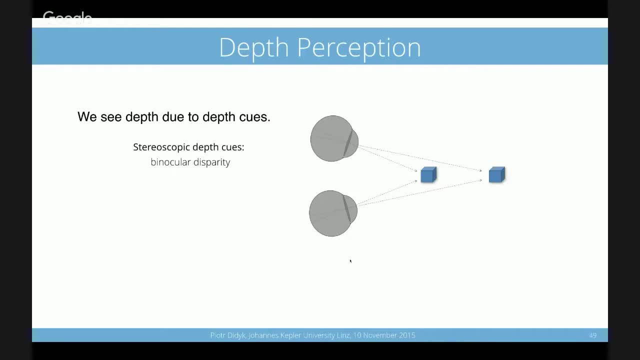 of the 3D effect that we get. That's not the only cue that contributes to depth perception. So those small disparities is essentially called binocular disparity and accounts for how different objects and different depths project on our retina and where they end up with respect to each other. 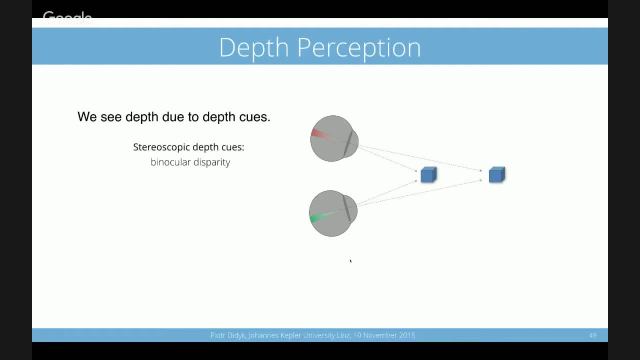 But there is a number of other cues, like the binocular disparity and the retina, which is a symbol with respect to each other. but there is number of other cues that also give us a good perception of depth, And those are those ocular depth cues. 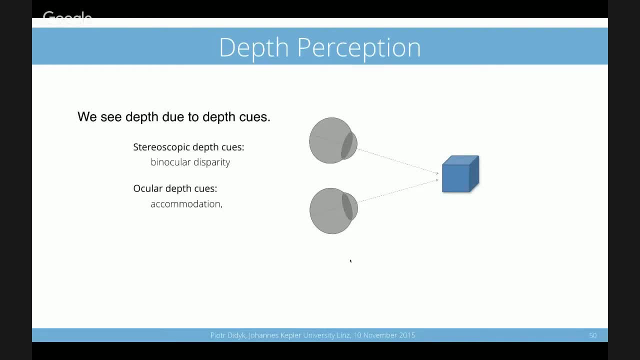 Maybe some of you have heard about accommodation, which is essentially the shape of the lens which set the picture that we see in focus, And the other is vergence, which is essentially the angle between our optical axis And those two. they are also very strong depth cues. 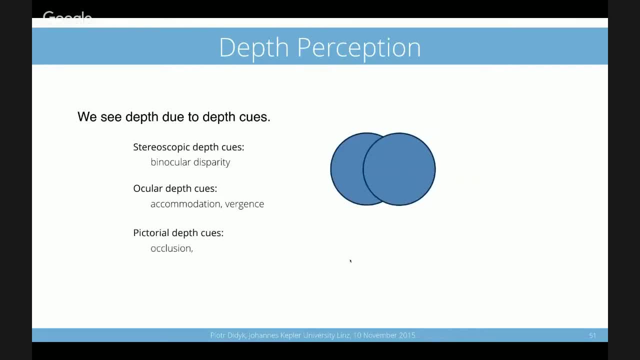 And there are also those pictorial depth cues that we have in 2D images, like occlusion size or shadows. Now, the thing is that in order to provide good stereoscopic content, we have those cues, have to be in agreement, However, on 2D screens. 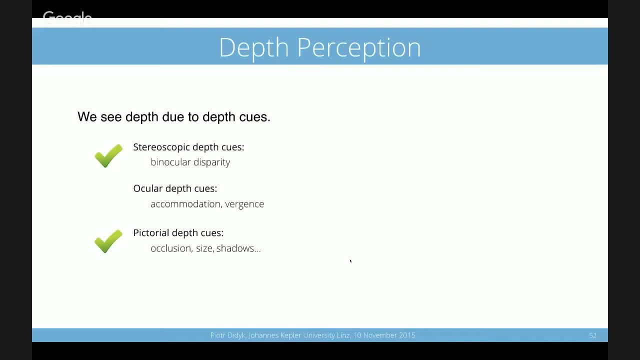 we can only reproduce those binocular disparities and pictorial depth cues, The ocular depth cues, accommodation vergence. they really require 3D space. We cannot really reproduce them on the standard 2D screen. And to just give you a more insight, why is it so? 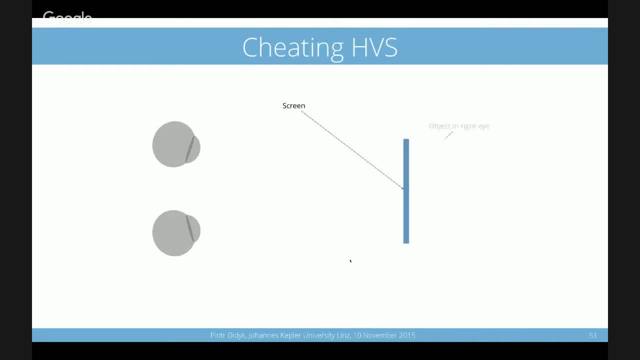 Let me just show you the simple example: when we have eyes looking at the screen and there is one object that we show in different position of the screen for both eyes to create an impression, in this case, of image floating in front of the screen. Now the problem is that if we look, 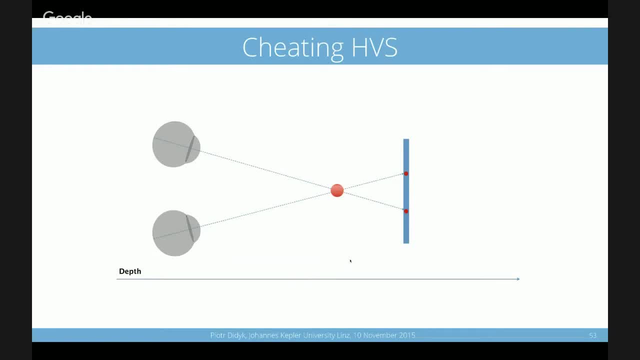 so this is what binocular disparity will tell us: that this object is floating in front of the screen. If we look at the vergence cue, it will stay in with agreement because the angle between the optical access will be correct. But if you look the accommodation, 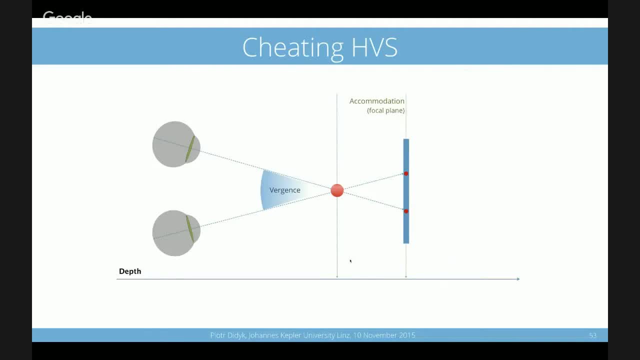 so where we actually accommodate, where our eyes set focus. this is actually the plane of the, this is the depth of the screen And this discrepancy between those cues, mainly accommodation and vergence. this creates a view, a viewing discomfort, because they remain in disagreement. 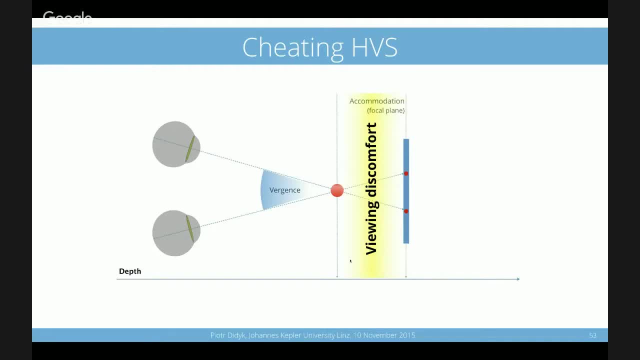 in the stereoscopic setup And they're actually coupled in nature. This discrepancy between them creates a viewing discomfort which, fortunately, can be tolerated in some region around the screen, but this range is very limited. So, in fact, what you have to do, 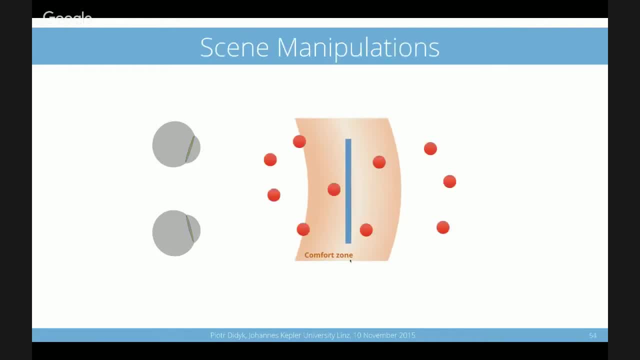 if you prepare the stereoscopic content and you have some objects that are further from the screen that discomfort zone allows, you actually have to. you have to bring those objects into the comfort zone to make sure that people will not experience viewing discomfort. So here, if you think again about the translation process, 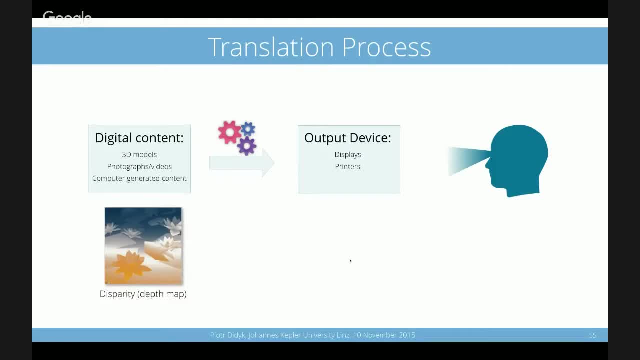 what you have as an input is some representation of the stereoscopic content, can be depth map together with images of disparity, And as an output, you have to reduce the depth map. this depth map reduce the range of depth that you show on the screen. 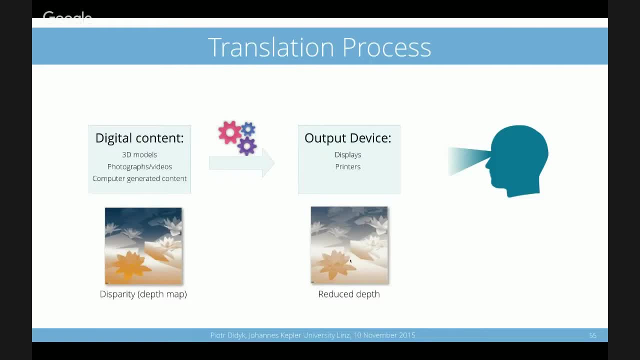 because you usually cannot reproduce and the depth range that you capture in real world. And to do this, we essentially want to account for sensitivity to disparity of the human visual system and to limits of the comfort. So how much people can tolerate of this depth range? 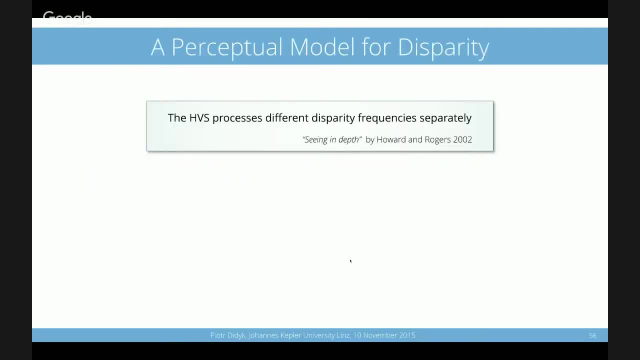 And so we address this in one of our work on modeling disparity, And the one thing that this and other models for human perception rely on is the fact that, deep in the brain, what we are doing, we are doing very simple image processing. 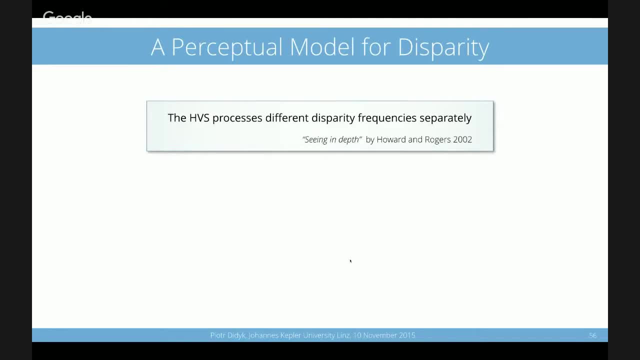 And it turns out that, similar to luminance perception, also disparity perception, what human brain does is essentially it has a different receptive fields that are tuned for patterns with different frequencies. And this essentially, this essentially, you know, this essentially gives us a hint that what the human brain does is actually some kind. 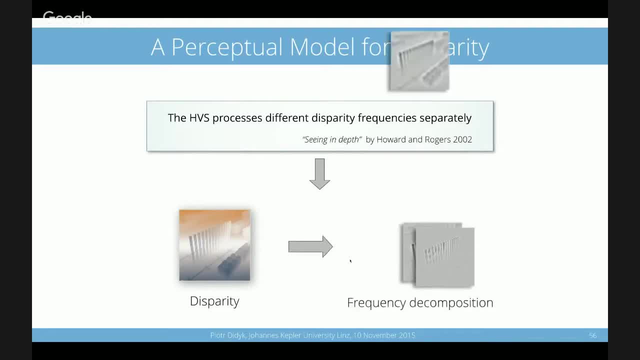 of the composition of complex images into different frequency bands, and then the brain kind of processes each of these bands separately. So now, if we want to simulate how such a processing works, it turns out to be sufficient to do experiments on simple patterns, because here the brain decomposes this image into different. 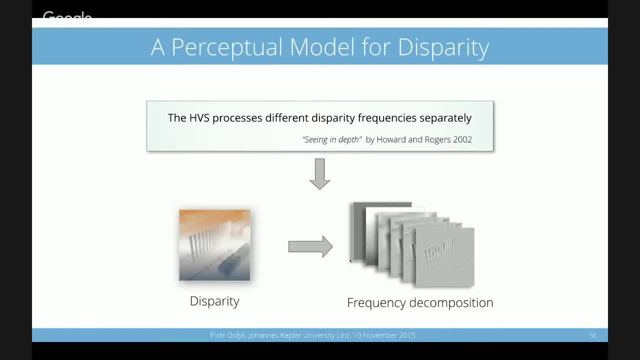 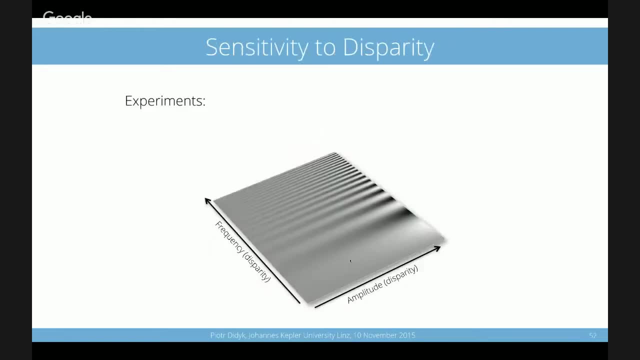 frequencies, What we did, what we can do. we can measure the performance of the human visual system, for example on sinusoidal patterns. So this is easy to do, because the space of different sinusoids, or sinusoidal depth corrugations in this case, is not that large, because this is controlled by, essentially, the amplitude. 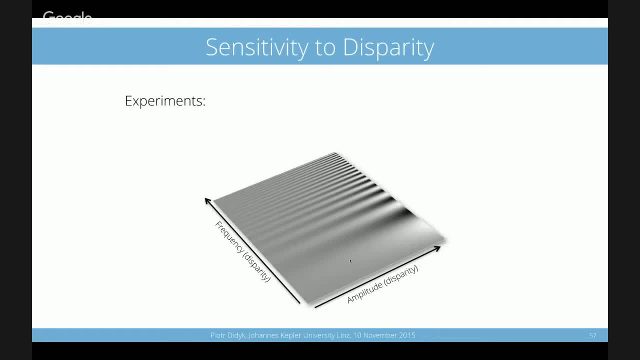 of disparity and the frequencies of the disparity, And then we can explore such a space and we can essentially measure how the human visual system responds to different signals, And in this case we can measure thresholds. so what's the smallest amplitude that is visible by the observer? or what's the minimum, the delta of the amplitude that people would perceive? 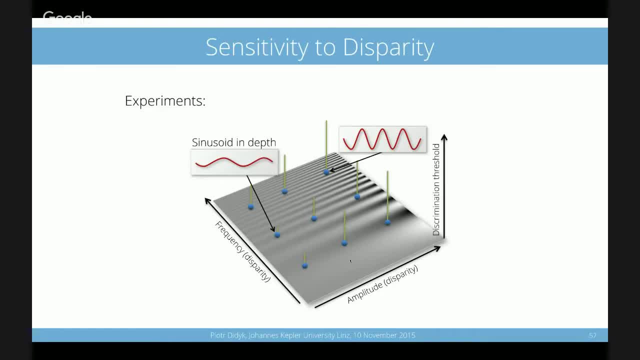 would see, And based on such measurements of sinusoids, we can apply them directly in this simulation. So here we have a sample of the human visual system so far, but in fact we can see that there are some differences in this, in this frequency decomposition. 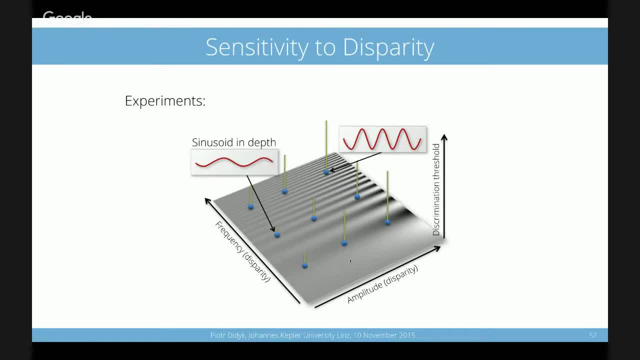 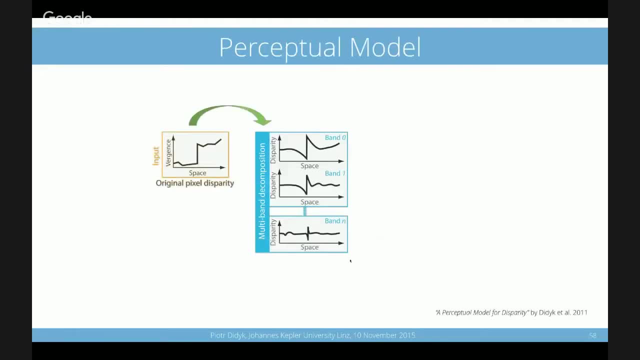 So, in fact, what we did? we did some experiments. I will not go into details, but we did some experiments on the sinusoidal patterns. And then, because we know that human visual system performs this kind of processing, we can follow it. and at the end, what we do? we take the depth information we similarly 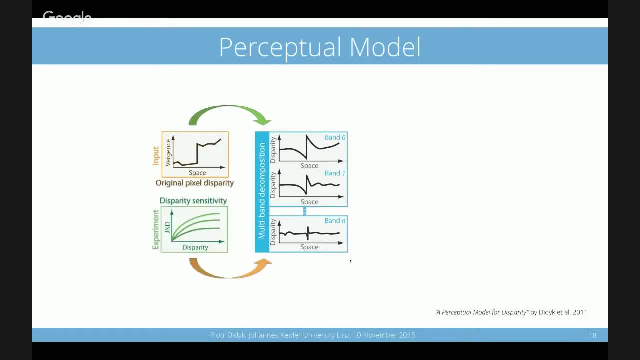 where we can actually apply this knowledge that we gain in the experiments done for sinusoidal depth corrugations, And then we can compute so-called perceptual space of the depth, where the depth is essentially at each band, at each frequency band is measured in some perceptual units. 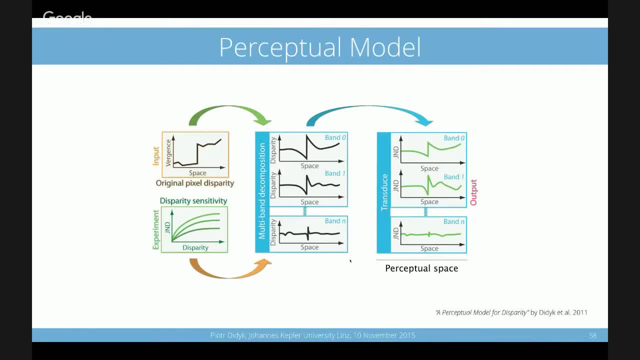 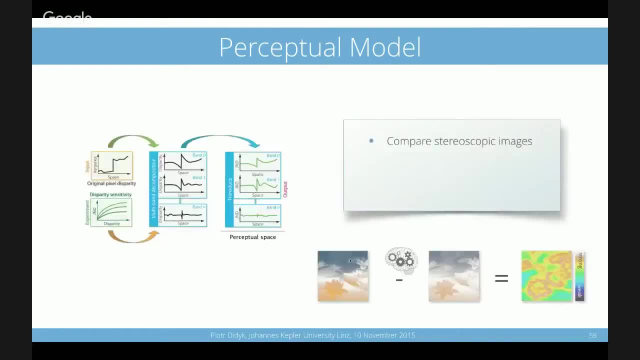 We call them just noticeable differences, where one JND would mean something that's barely visible. And then, if we have such model, we can essentially do many different things. For example, we can compare stereoscopic images because we can perform such a decomposition for two images. 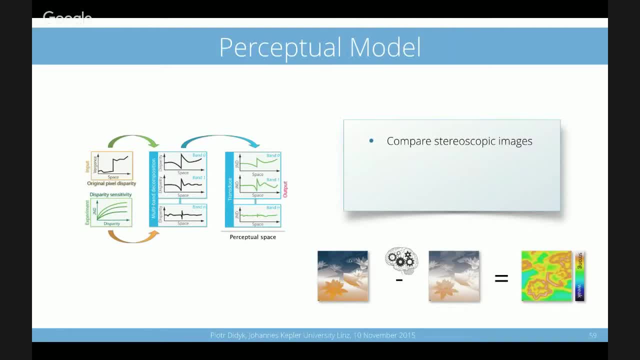 and we can compare them. We can compare those JNDs and know what's visible. We can also remove the signal that's invisible, because we know that everything that would be below this one just noticeable difference is invisible. So, for example, we can remove it for a compression purpose. 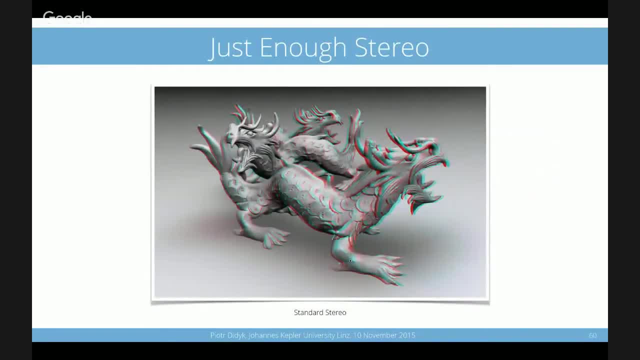 Wow, One interesting thing that we did with this model is something which we called backward-compatible stereo or just enough stereo, And essentially the observation was that not everybody likes the stereo, And if you have two people, one of them likes stereoscopic images. 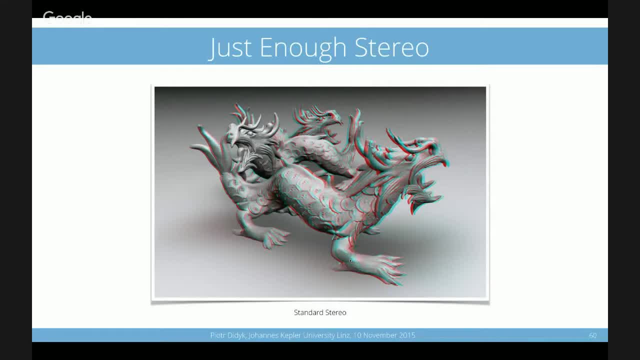 and the other doesn't. it's usually. you have two choices, Either in both cases: either the person that doesn't like the stereoscopic image will see those color artifacts while the other person will enjoy the stereoscopic impression, or the person that likes stereoscopic impression will not see stereo. 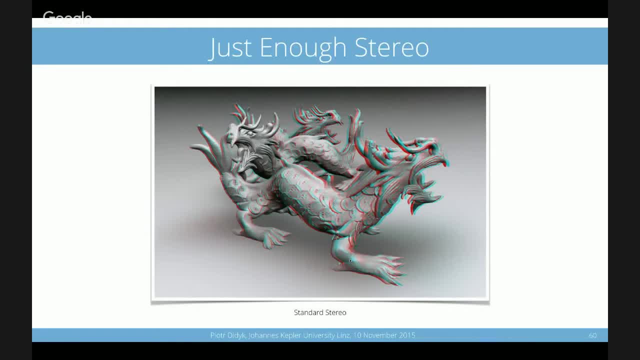 because the other person wants to see a clear image. What we propose is something which is just enough stereo. I'm not sure how much you will see on the video that you see there, but essentially we are able, according to our prediction, done by our model. 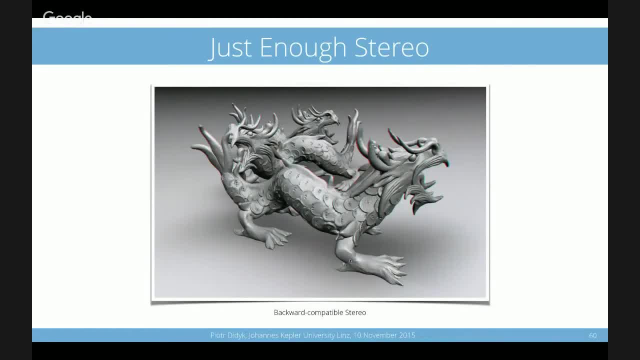 we can limit the disparities that we use in this, in this image, to minimum, just to make sure that the stereoscopic effect is visible, And this allows us to apply as little stereo as is necessary to see. So that's good for the person that likes stereo. 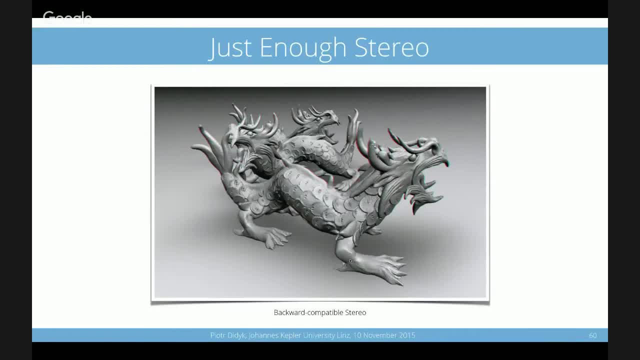 But on the other hand, the person that doesn't like the stereo and, for example, doesn't want the, doesn't wear the glasses- necessary glasses. that person doesn't see that much artifacts. So if you compare this and this, this is again, this is very tiny artifacts here. 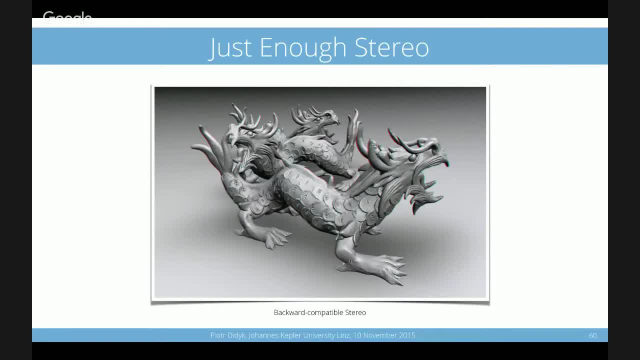 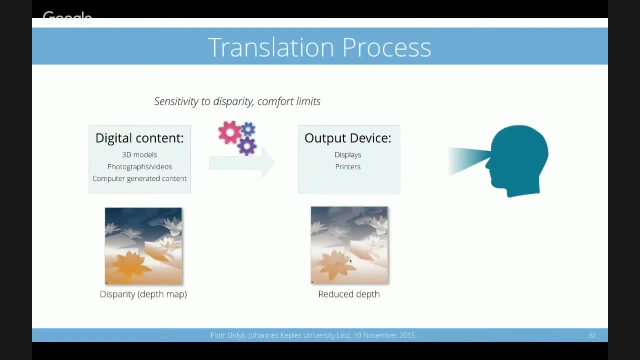 But if you wear glasses, you actually have a good, quite good impression of of of stereo. We also did some work concerning the temporal domain, as those are only static images where the input is the the image sequence and the output is optimized image sequence. 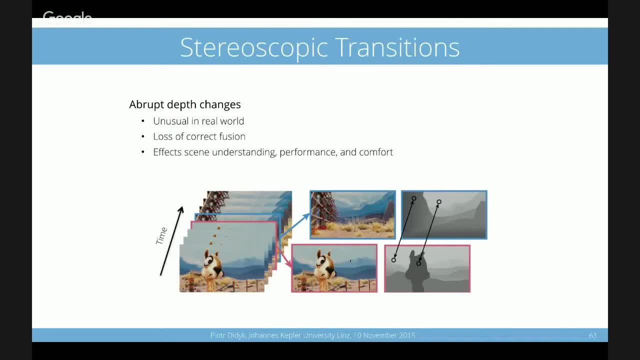 that you show over time. Here, the problem that we consider was stereoscopic cuts. that can be very disturbing because you're exposed, because you're exposed to very rapid changes of depth, So something that you cannot really observe in reality, because when you we look around. 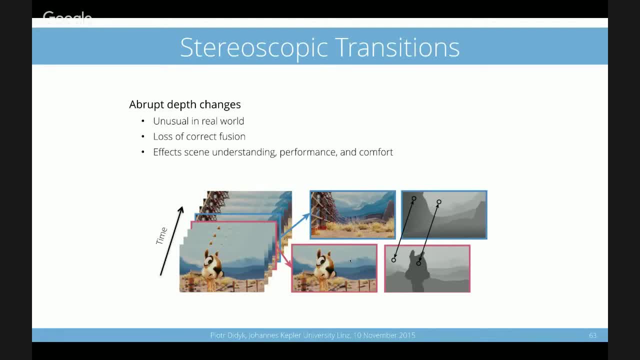 we can control what we see and we kind of predict on what kind of depth we are verging at every moment in time. When we watch the movie we don't have, we don't know actually what is the intention of director, So we can be exposed in very rapid depth changes. 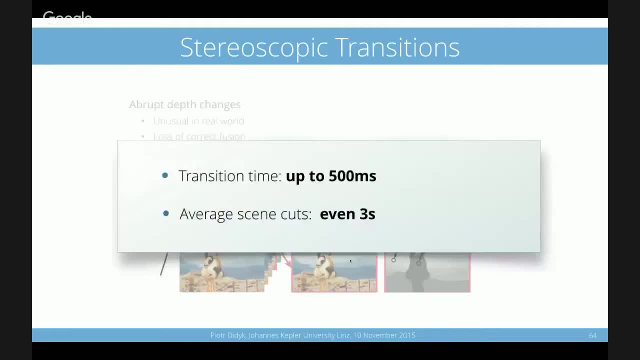 which can be very annoying. And just to give you some statistics, such a transition time between one depth to another can take up to 500 milliseconds, And it turns out that the average scene cut in the action movies around three seconds. So this just give you an idea how much time you lose. 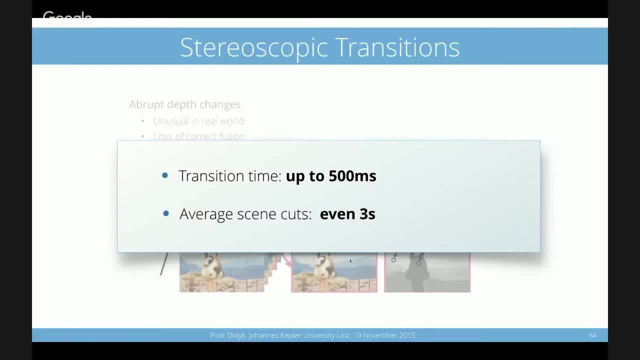 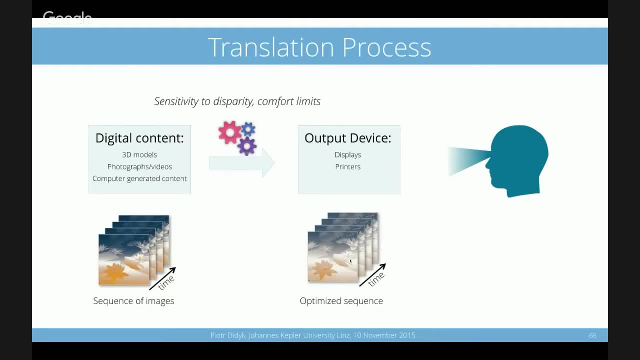 on just changing the depth at which you're focusing, And in this project we were investigating and optimizing the sequence depending of the performance of people, on focusing on different depth levels in the context of so here we accounted for the human interaction and performance. 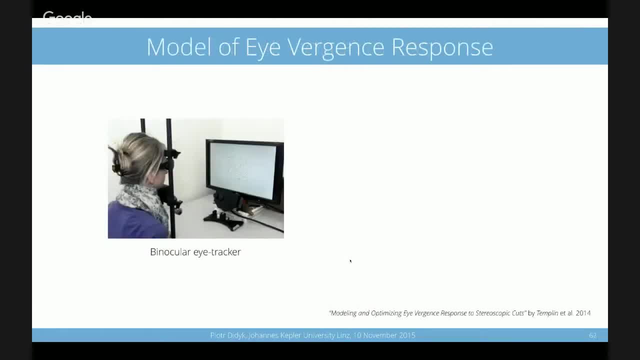 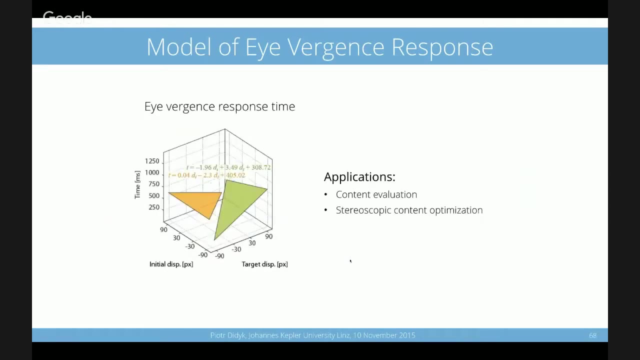 And what we essentially did. we run again bunch of experiment where we exposed people to stimuli shown and different depths. So that was more or less the experiment that we run And then from that we could derive the model that essentially predicts how long it takes for people to change the divergence. 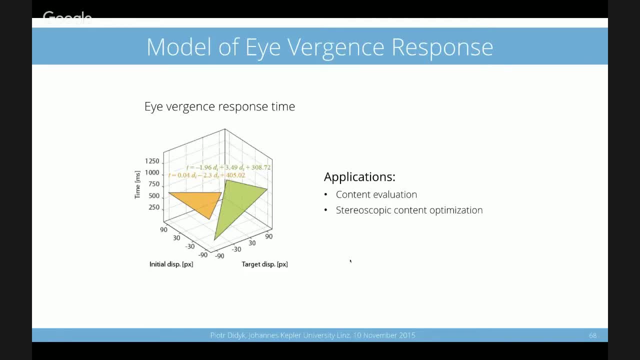 from one depth level to the other level And based on this we can work out, we can evaluate the content so we can, for example, tell how much time people will lose for this reverging, or we can also advise the techniques for actually optimizing stereoscopic. 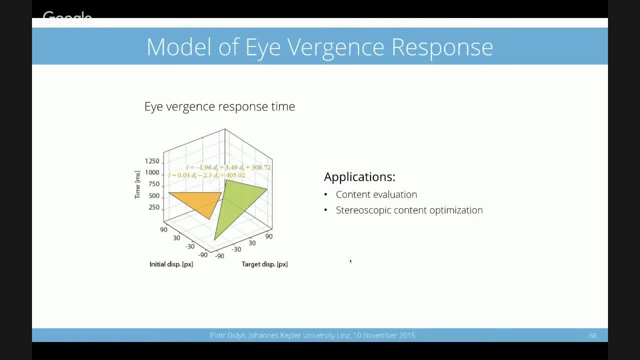 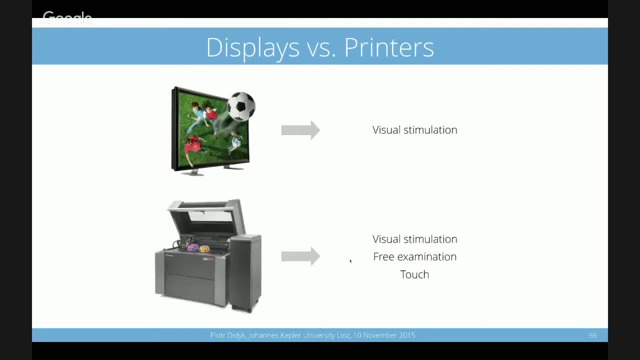 content to minimize the time and efforts that people need to put into watching this content. So far, I talk only about the visual stimulation, so I talk about the displays. Now I want to briefly talk about the 3D printing, which doesn't only provide us with visual stimulation, but also 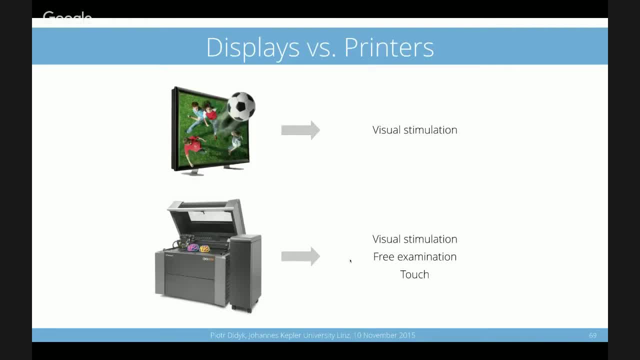 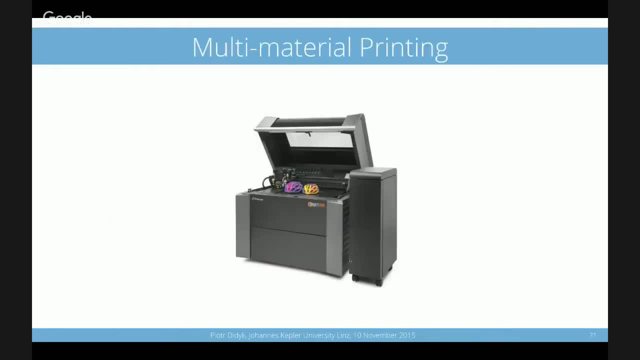 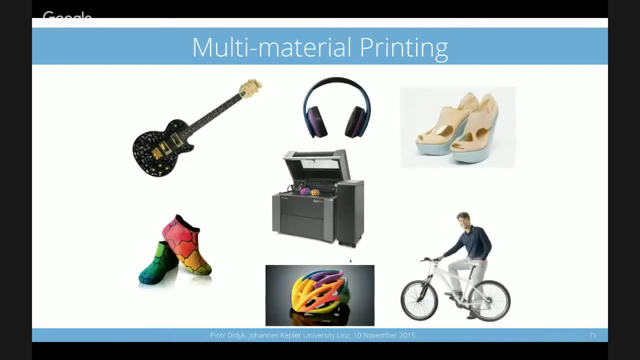 we can touch those objects and we can examine those objects, as those are real 3D objects. So I will now talk a bit about the multi-material printing and the work that we've done here. So currently, with such printer as this Object 500, we can print a big variety of different objects. The problem is that we don't have a lot of time to do that, So we can't do that. So we can't do that, So we can't. So currently, with such printer as this Object 500, we can print a big variety of different objects. The problem is that 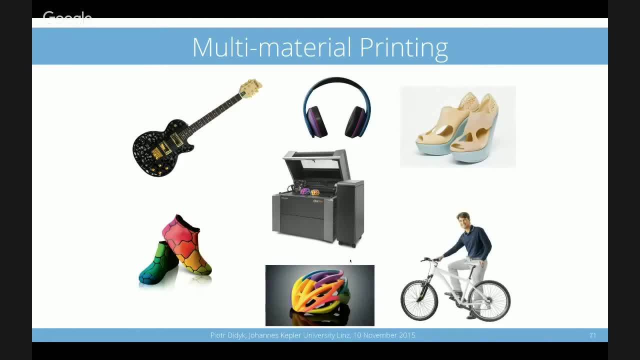 whenever you want to print such objects, it's almost you really require an artist who will do this design for you. This is not really those objects that are here. They're not really produced by naive users, And the problem with this is that. 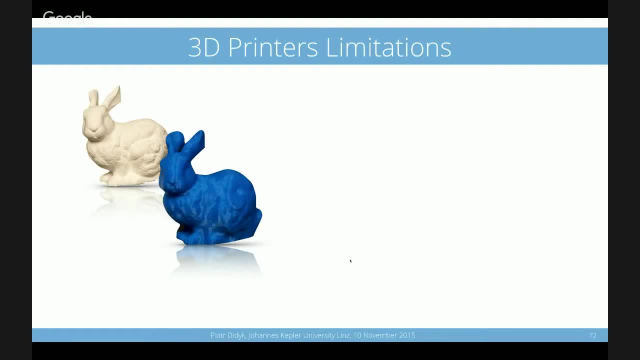 if you look at the multi-material printing and you want to print your objects, the first thing that you realize is the printer doesn't see your object. It doesn't know what you want to really achieve, but it only sees, by a bunch of pixels, that it will be filled by different materials. 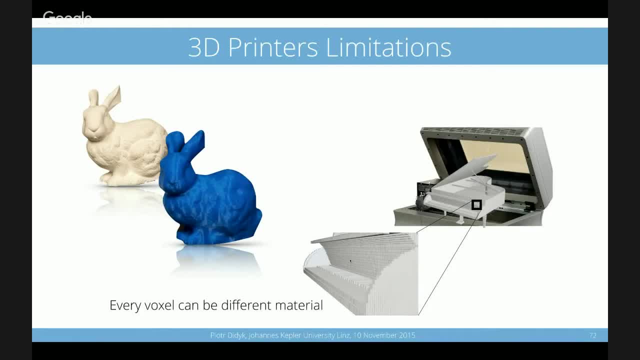 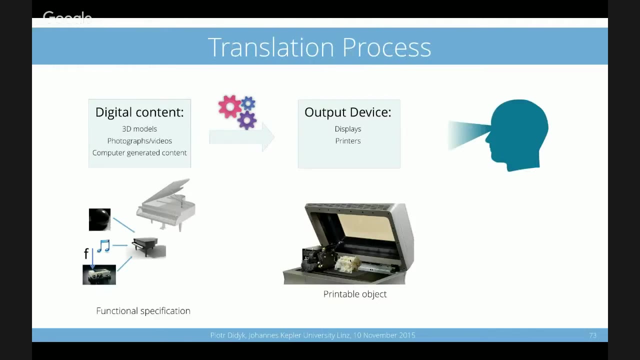 So essentially, what you have to solve is you have to solve for the assignment of multiple materials that you have on your printer to those voxels that will be at the end printed And, in this context, the translation process. we consider this functional specification. 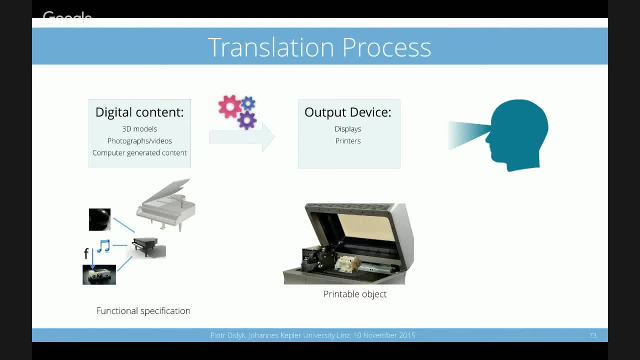 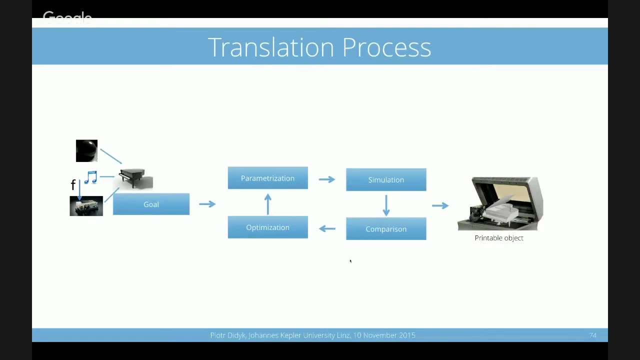 So the user has to specify the geometry and some high-level properties like reflectance, mechanical properties, and you want to translate this data into something which is understandable by the printer. So this is usually done in this, as it's shown here, in kind of optimization loop. 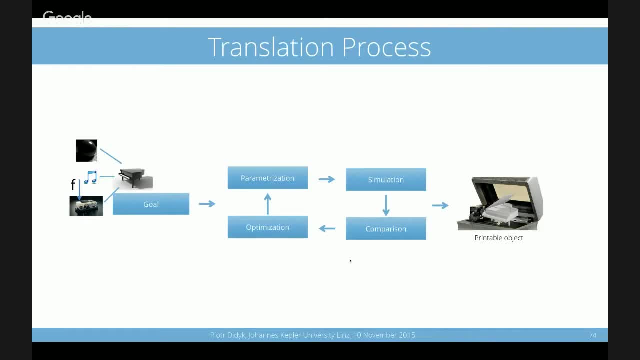 When you have the goal that you specify, then you have a parameterization of your geometry over which you optimize for different materials. then you usually have to be able to simulate this assignment, how this object would look in real world And how people would interact with this object. 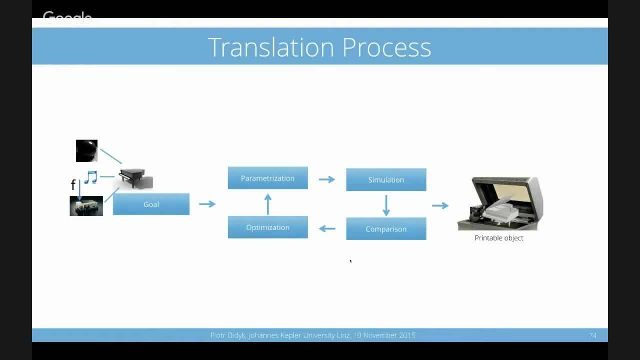 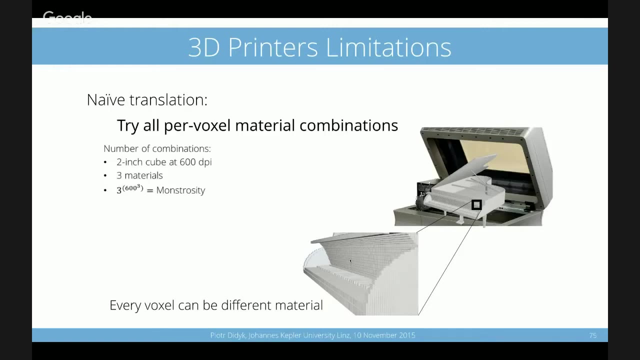 And then you have to on top of it, you have to have optimization that essentially optimizes for this material assignment. So the brute force approach is to have this per-voxel material assignment. but you quickly realize that if you try to optimize the material assignment on per-voxel basis, this will explode. 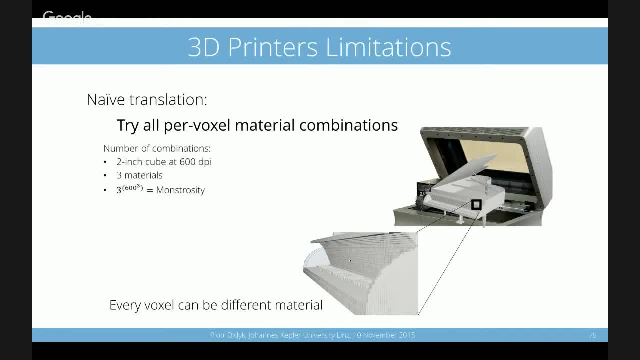 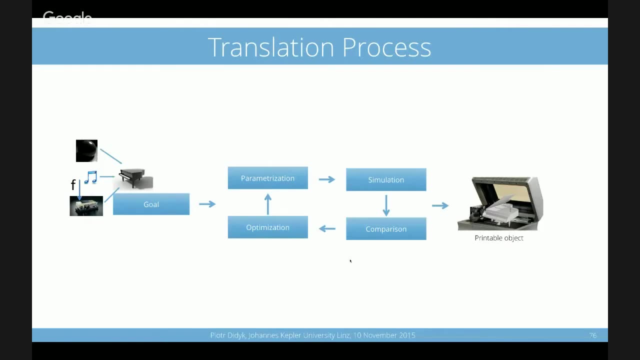 This will have a There's really humongous amount of possibilities. There's a lot of possibilities that you can consider. So the work that we did two years ago is about parameterization of those 3D objects for such kind of specifications. 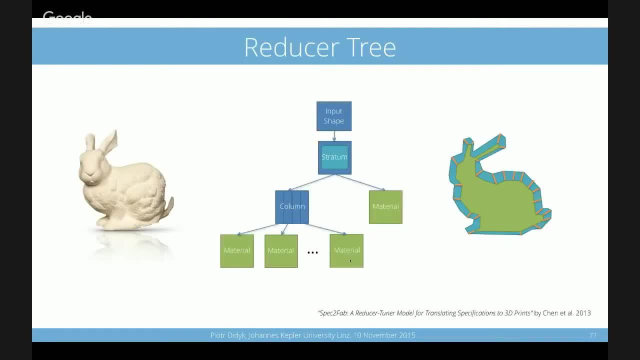 So, instead of having per-voxel parameterization, we created a so-called transducer tree which in fact is nothing else than a hierarchical space subdivision, but it's really tailored to the applications in the application. So, whatever it is you need, you need to have permission for. 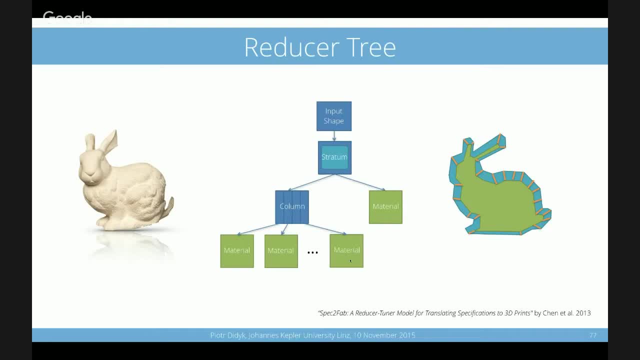 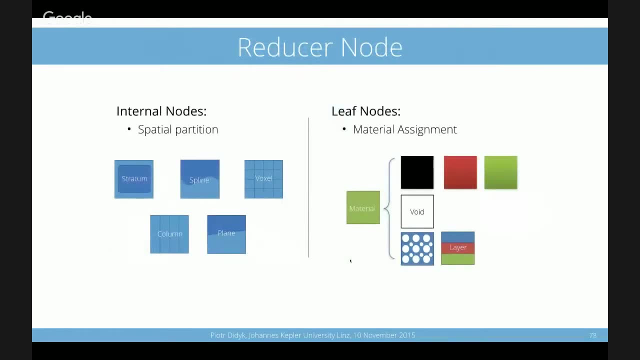 in 3D printing. So in this case the object can be broke down into several pieces by those internal nodes, And those internal nodes they consist of, in this case five different techniques for splitting the volume, And then the leaf nodes. 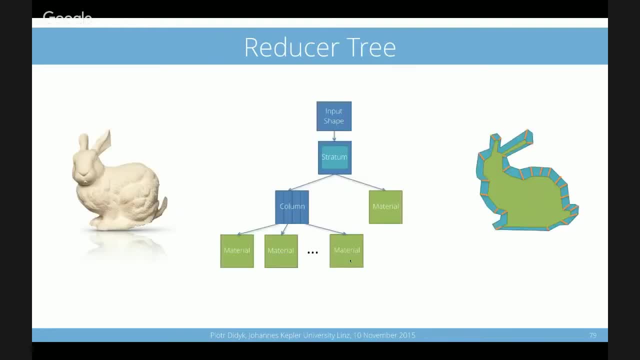 they encode the material assignment. So this is the example how you can break this bunny into such representation. And now the thing is that, instead of optimizing for the individual voxels, you only optimize for those material in those bigger chunks of the volume that are at the end of this tree. 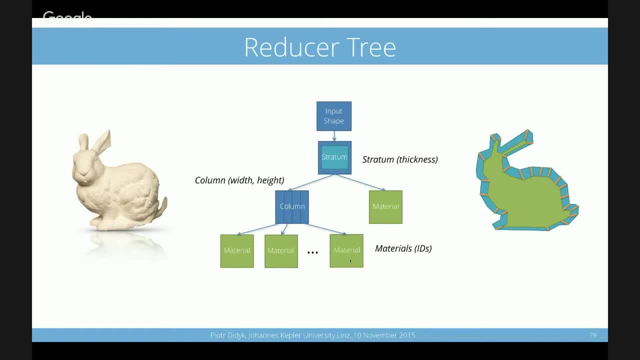 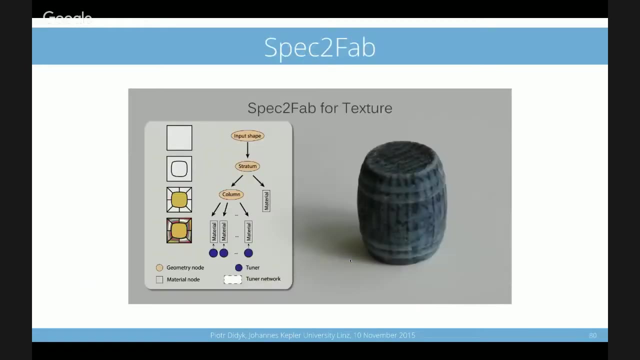 And you also optimize for those parameters of those subdivision components. So, for example, if you have the stratum which divides the object into outer shell and the inner part, you may optimize for the thickness that the shell has And with this reparameterization. 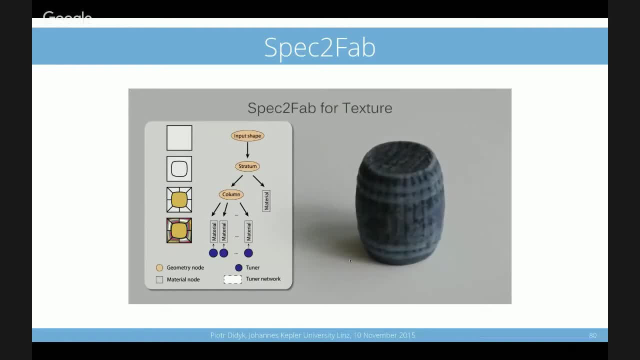 we were able to, in a pretty easy way, come up with different fabrication techniques. So here, for example, our results for texturing. but we can also combine those things and do, for example, texturing and subsurface scattering. So this is again texturing. 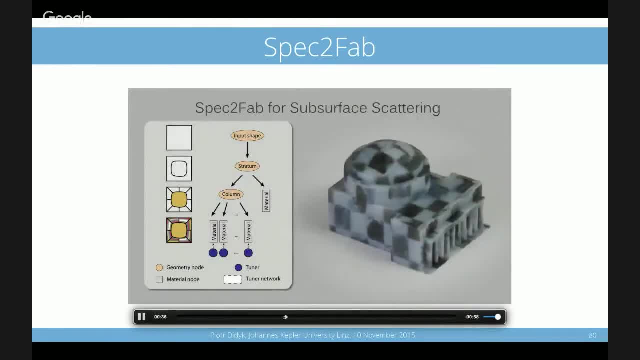 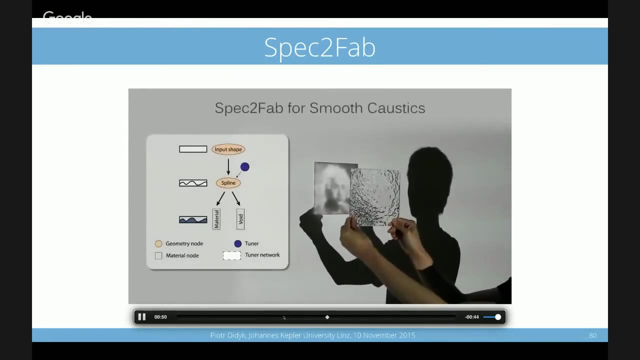 I will just browse it. maybe This is for subsurface scattering, And the nice thing here about this parametrization and this framework for creating those fabrication techniques is that you can easily combine them. So this is, for example: here is the producing smooth caustics. 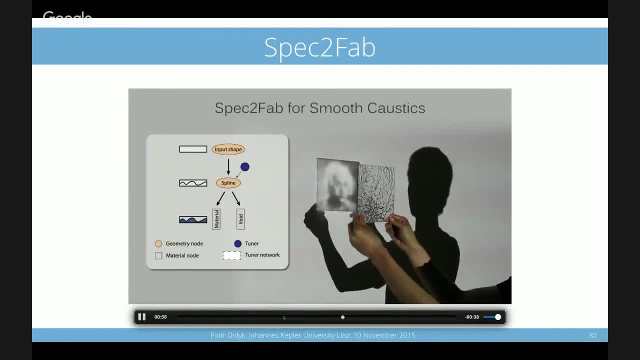 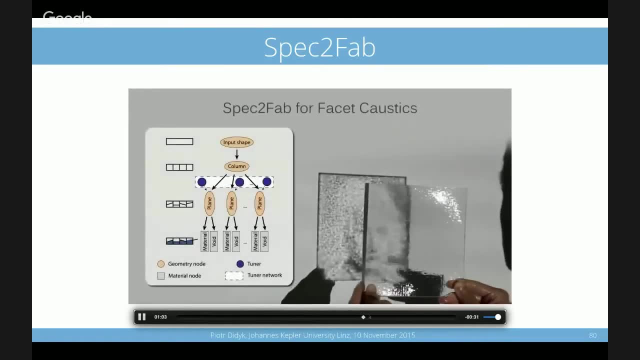 So this is the work that this is essentially. we show that we can, with such a simple approach and simple specification, we can reproduce the techniques that were already presented before. But, what is more interesting, we can actually combine those things. So, for example, texture and mechanical appropriation. 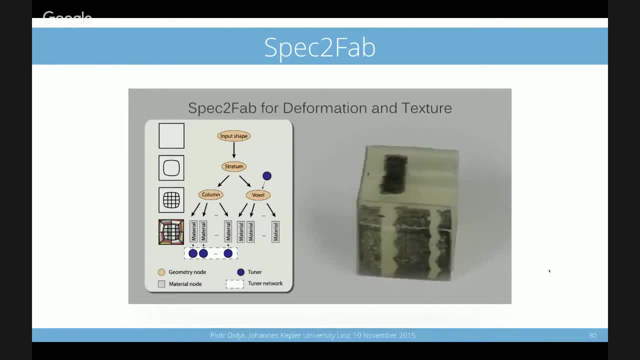 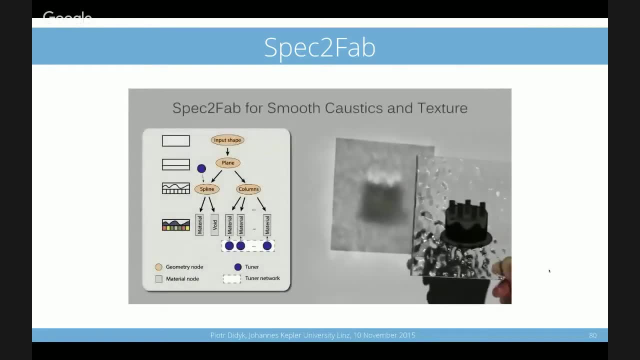 and so on. So we can combine those properties, we can combine them into one tree, We can take those trees and we can create a completely new fabrication techniques. So here is again texture and caustics. We can combine two and jointly optimize. 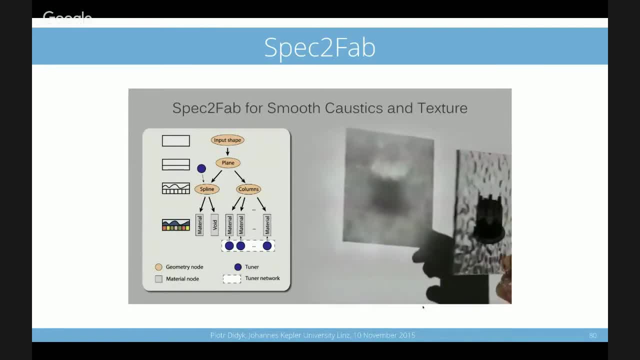 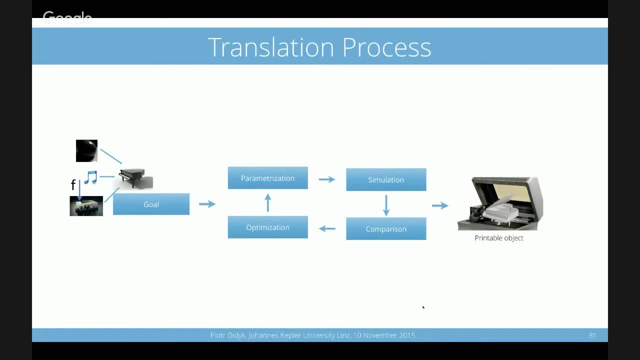 for the material assignment. Okay, there's just one more thing that I would like to mention that I'm maybe I'm currently working on, and that does the region. that's the field that I would like to expand to a bit. I think it's worth noting that this 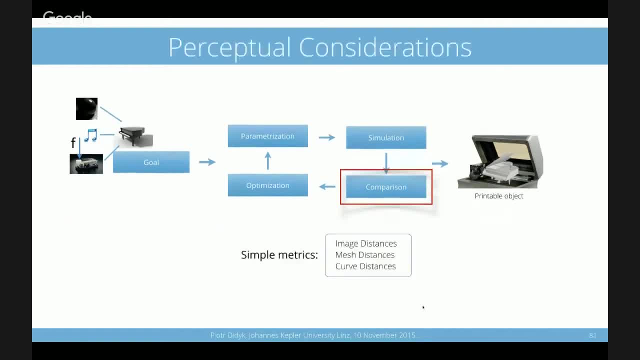 in the slope. we have this comparison and currently what is done in this box? those are very simple metrics like image distance, mesh distance, curve distances, But in fact, if you think what I said before, many of those objects are going to be handled by the humans. 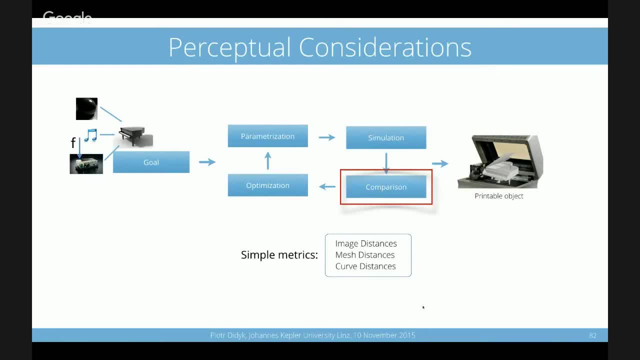 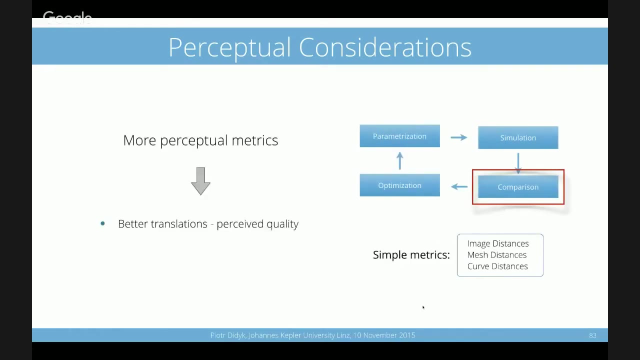 and humans will interact with them. It really there is really question whether we should not investigate those metrics and actually try to come up with some smarter metrics that will model the human perception in a better way, and possible benefits of designing those better metrics for fabrication is that we probably may get. 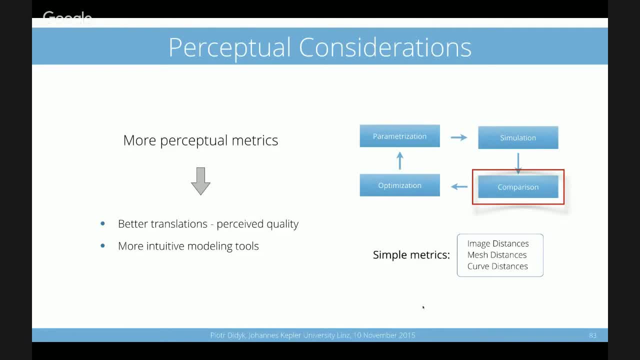 a better translations algorithm, So with the perceived quality will improve And in fact we also may get a more intuitive modeling tools, because if you think, for example, of tools that assign different materials with different mechanical properties, those tools are not really intuitive for knife. 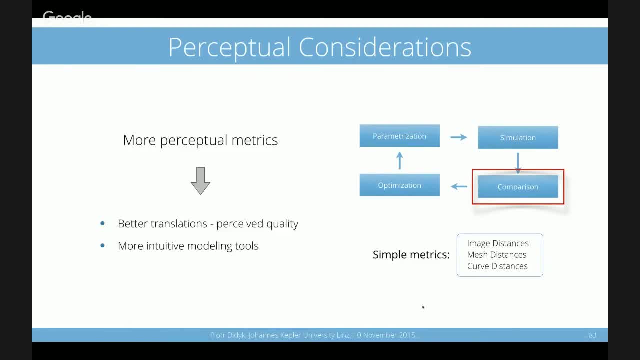 users. maybe they want to know which material is softer, which is stiffer, but they don't want to tune hundreds of parameters that those material have. So I think there is also interesting work to be done there. Okay, so to conclude, I hope I convinced you. 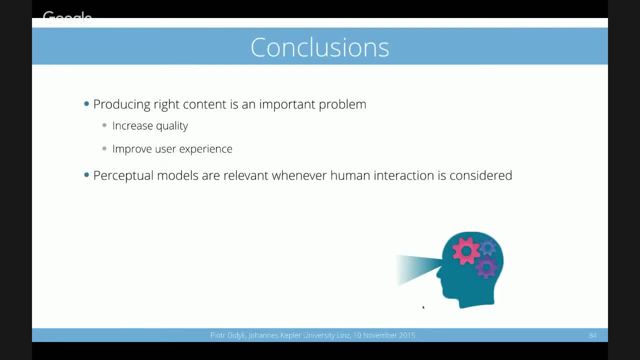 that producing the right content is an important problem And if you take into account, actually, the human observer that at the end interacts with this content, we can increase the quality, you can improve the user experience And in this context, the perception models are very relevant. 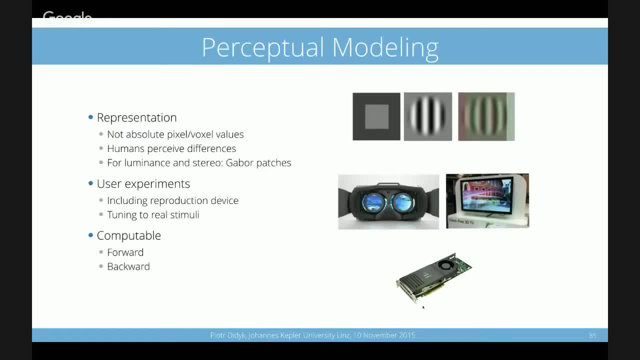 when you consider this human interaction And just to give you this overview on this perception, modeling that we try to do and what are important components is: first of all, if you want to do such stuff, it's important to pick up the right representation. 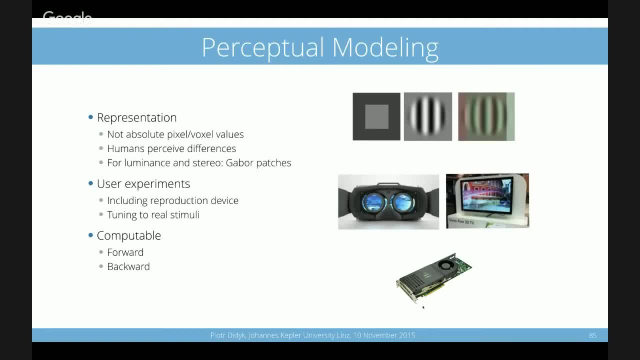 So we usually don't deal with complex images. We kind of try to represent those complex images or complex geometry. We try to do it in photos and pictures, we try to do it via images, so with some simple basic functions, so to say, someone can call it. 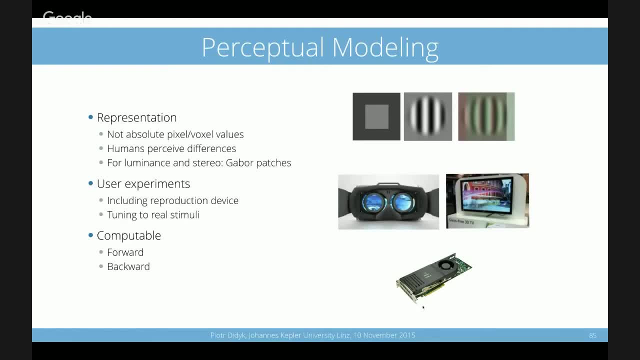 So, for example, it can be carbon patches. And then we have to run user experiments where we measure some phenomena, some thresholds, how people see different seasons, so on, And we really want those models to be computable forward and backwards. So we usually want to predict what people want to see. 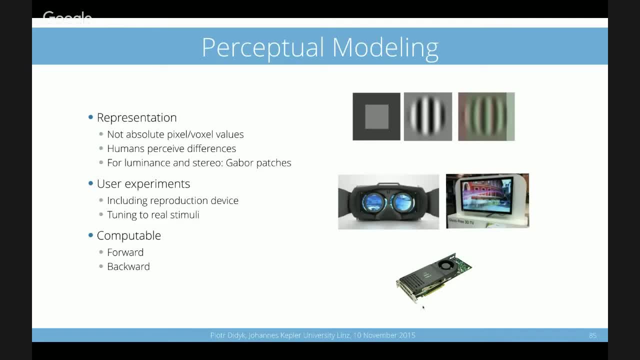 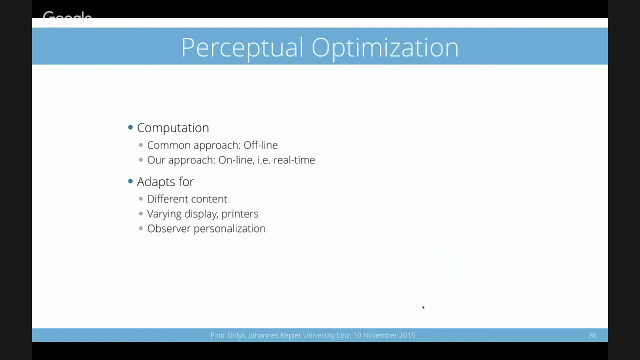 predict based on the content, based on the content that we show. what we see will see, but we also want to base on what we see. we want to predict what the content we would like to shown on the screen. and, yeah, in the context of 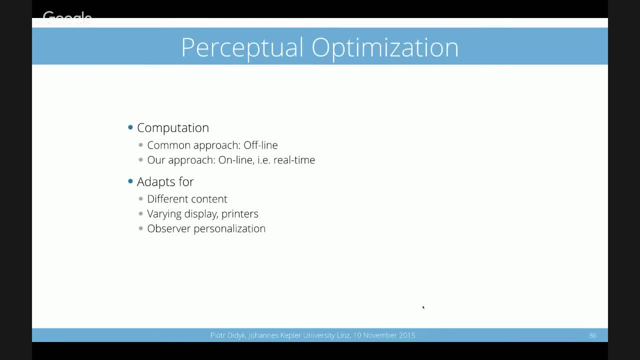 perceptual optimization. we usually try to design the online processes, so most of the techniques that I was showing they run in real time. this is important for us, for example, for graphics application, and we also care that those methods adapt to different content, different devices, and also we account. 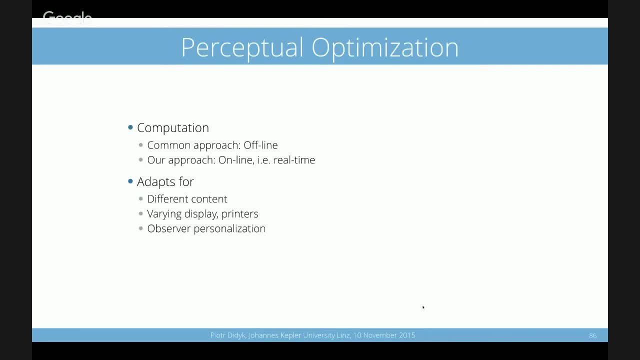 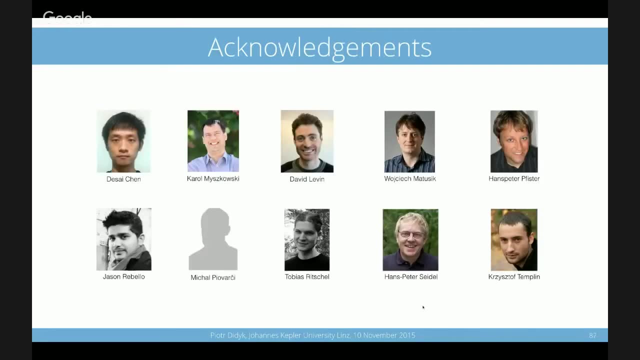 for observer personalization. so, for example of this, just enough stereo. this was kind of example of observer personalization, okay, so just I would like to mention people that work with me, and without them, I think this, this, I would be not presenting this work to you today. so, yeah, there were many people. 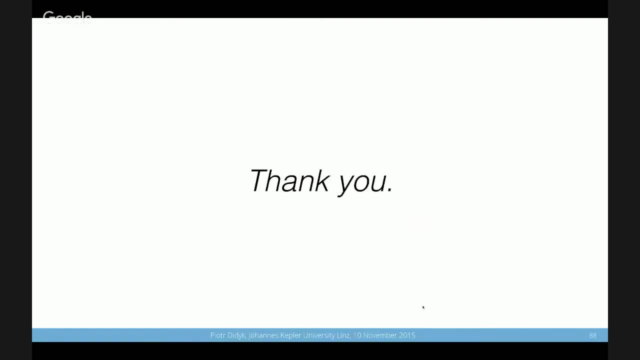 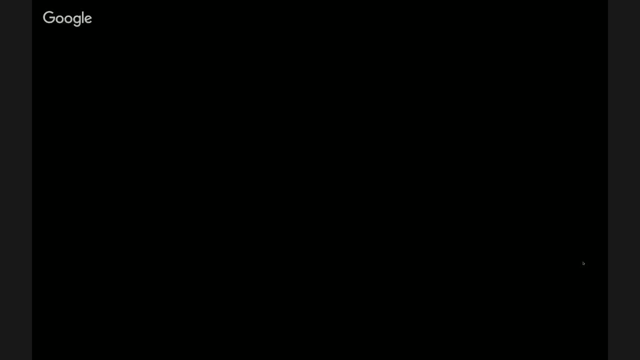 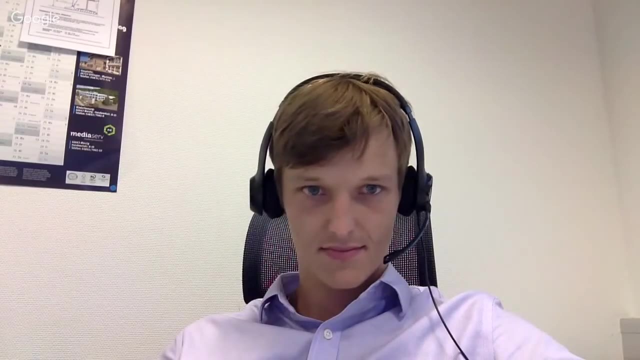 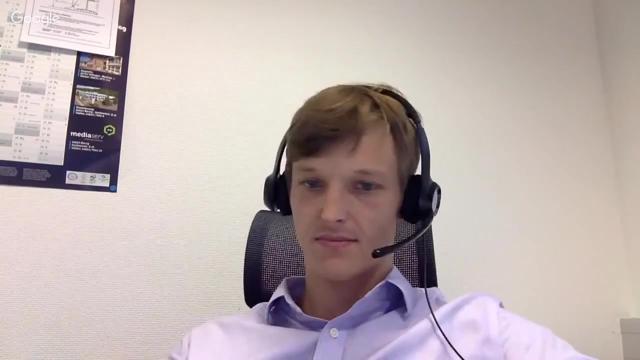 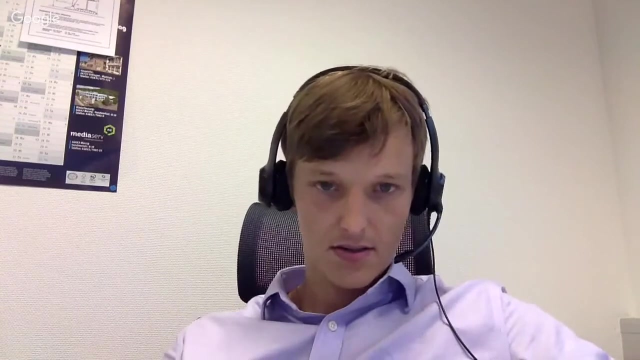 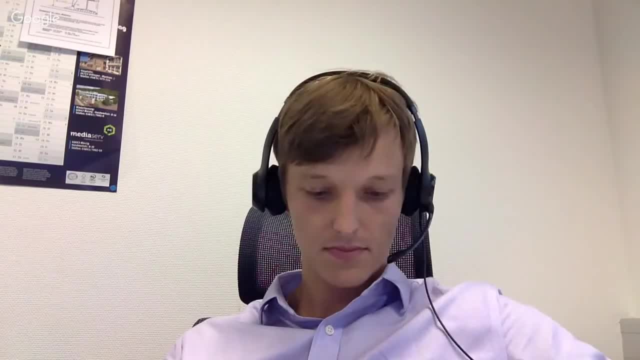 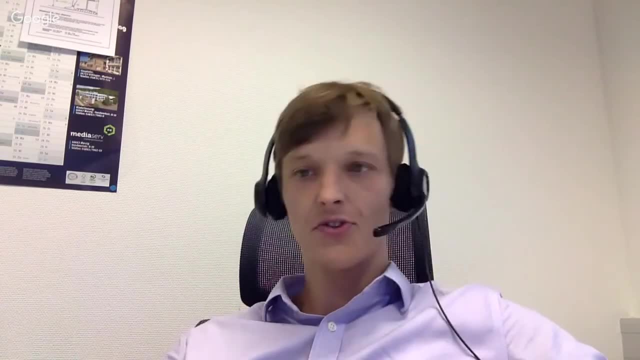 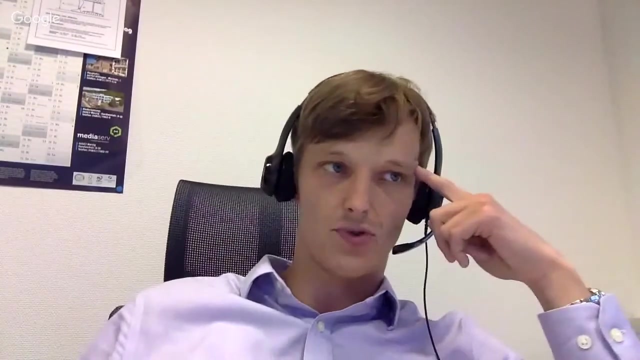 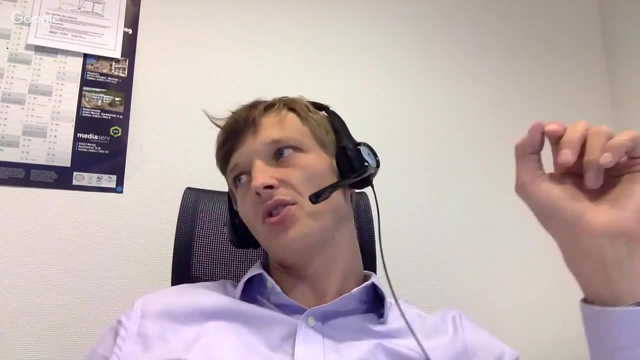 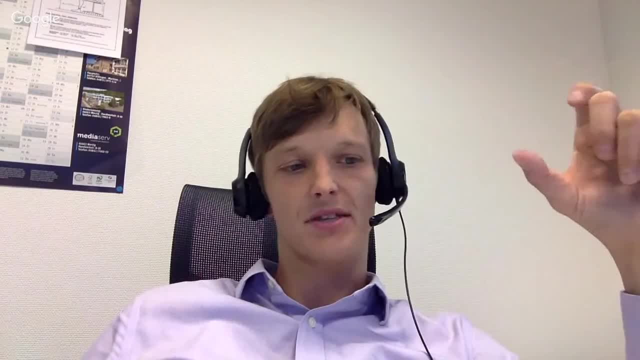 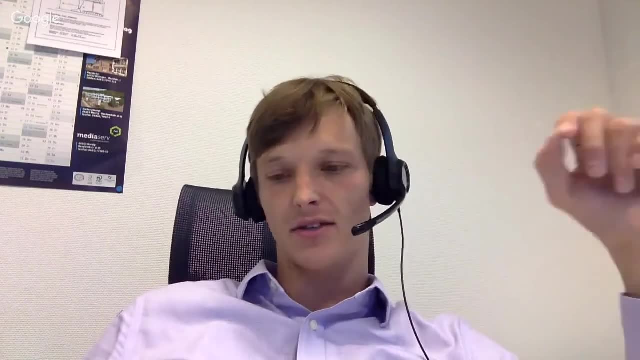 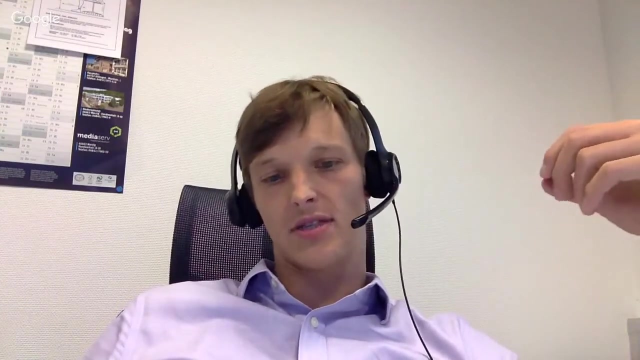 certain phenomena. So I'm happy that this is you know. so there are also those people like hardcore perception, people vision perception. they would run even more specific experiment just to show certain phenomena. We take them a bit step further to actually make them applicable. 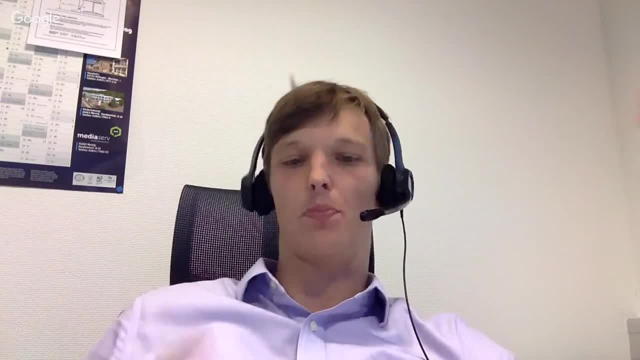 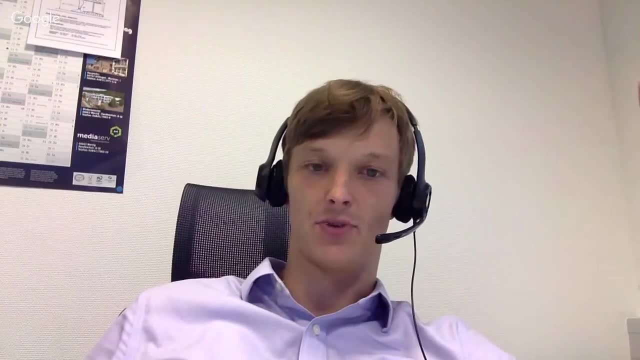 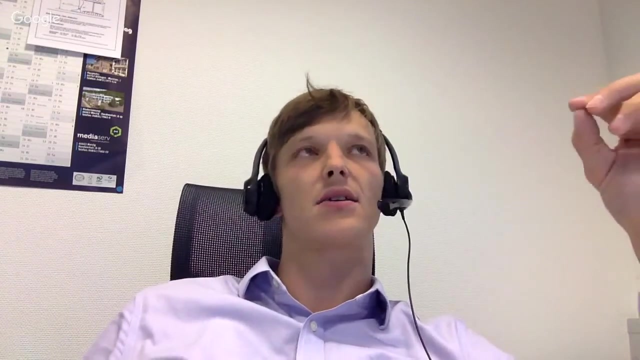 for complex images, But I don't think we have a complete model that would, for example, model completely the temporal aspect of the perception. So, for example, in the project that I shown here, this is really, this was really something that was saying, that was. 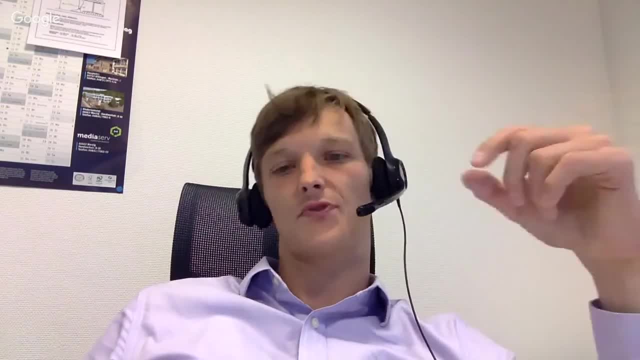 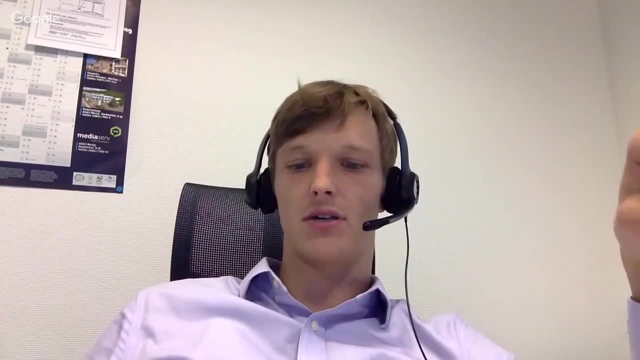 letting us know or was predicting what kind of signal, how much we can vary the signal over time, So we see the static content instead of instead of changing content over signal over time. Yes, So this was very specific And I think. 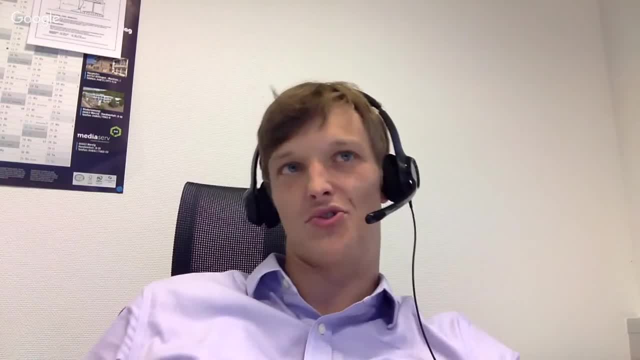 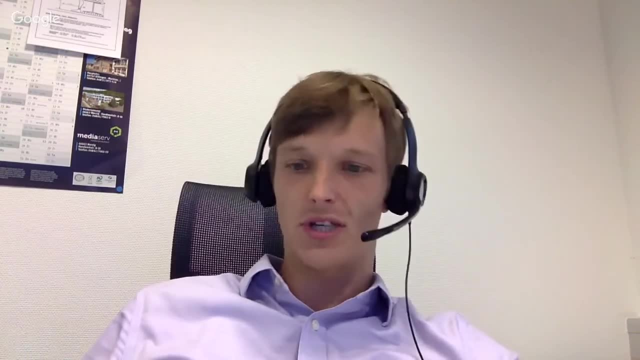 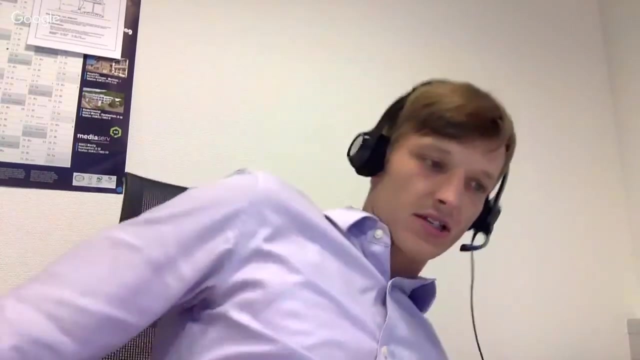 yeah. So, as I said, like in any of this project, the user- I think that's what we were asking about- plays an important role, in the sense that we almost always have to design new models. Yes, So we try to. we try to kind of bridge those things and try to build models that. 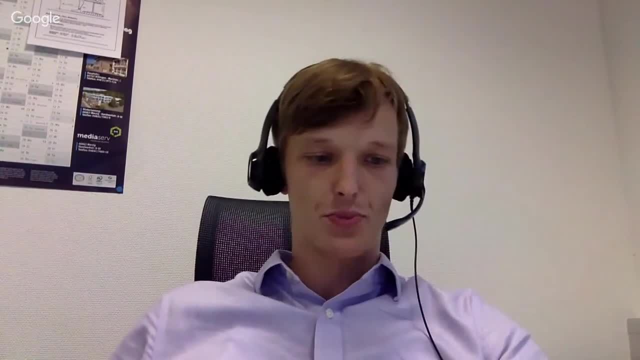 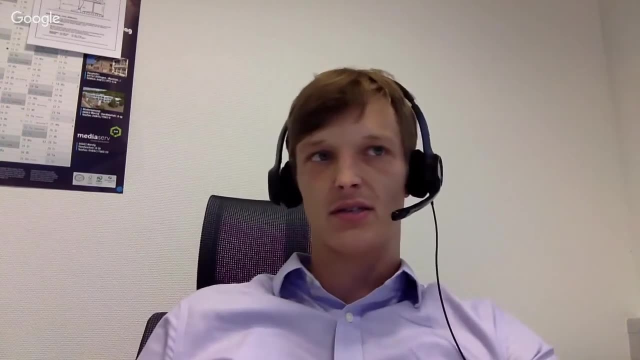 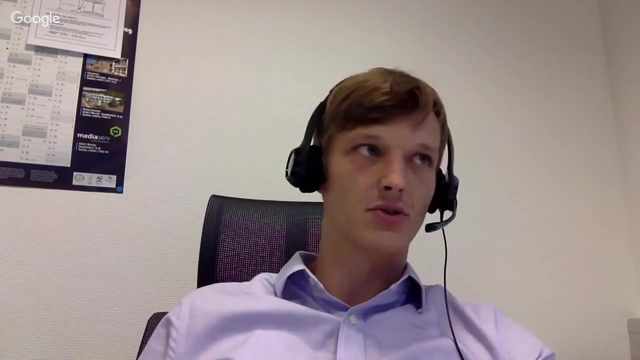 are more general, but the more general you want to build those models, the more difficult it gets. So we are rather considering like smaller assets, Yeah, So we're really looking at like the individual aspects and then taking advantage of them. Yes, It's also always the question how accurate you have to be in modeling those things, because 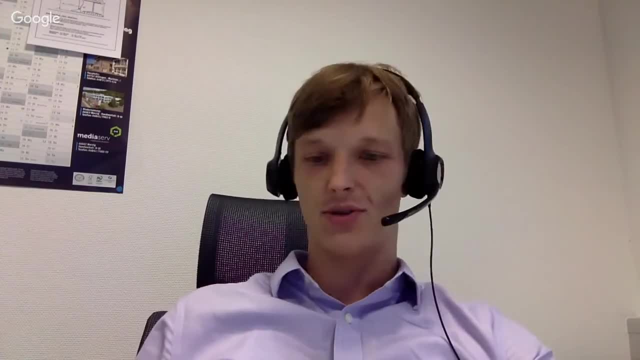 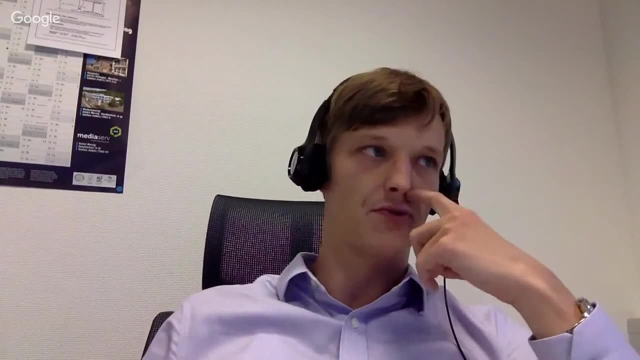 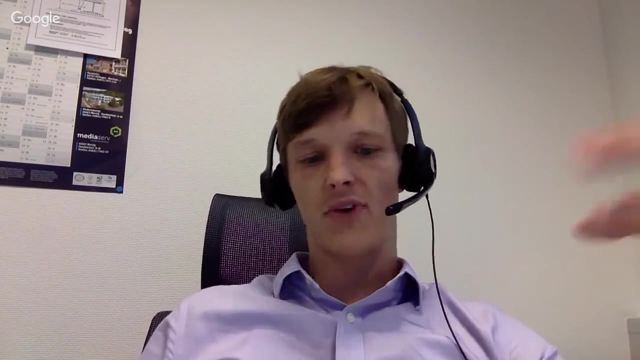 it's known that every model is incorrect. Yes, You cannot. you cannot probably be perfect. but also what we try to do, we try to show that, you know, even we make some assumptions and simplifications. at the end, We always- not the only- rely on those models that we 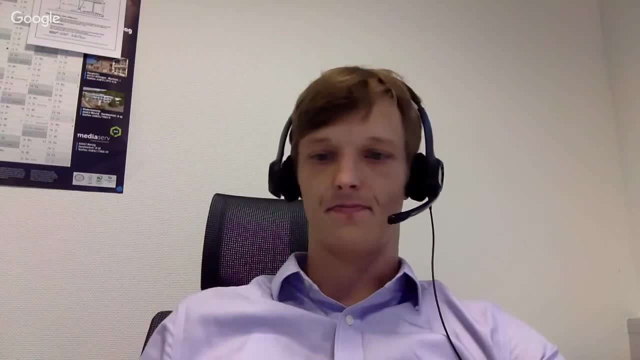 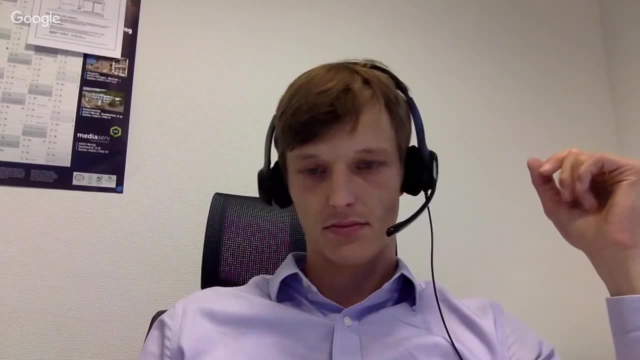 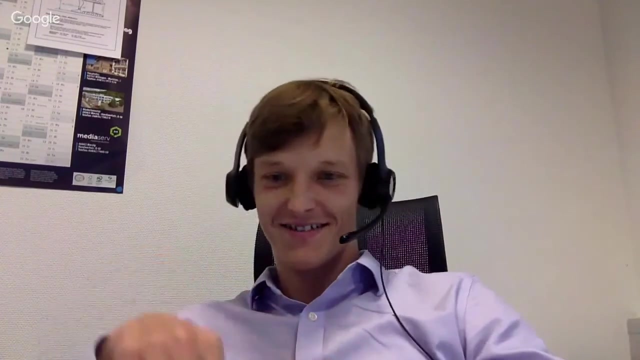 build, but we validate those things as well. Yeah, Okay, Yes them in the context of the application. yes, any more questions? I have a couple of specific questions and I think people warm up later on. you mentioned that you always, or often, use artificial stimuli, like our patches, to do your experiments. 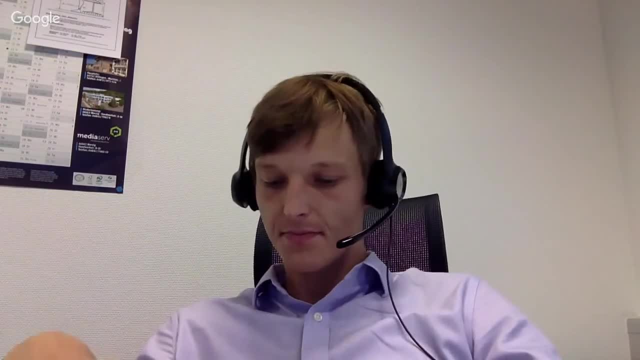 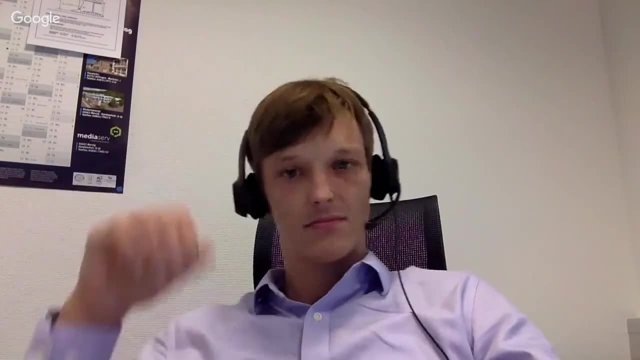 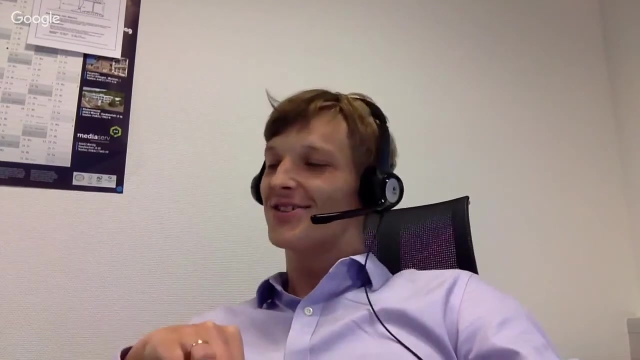 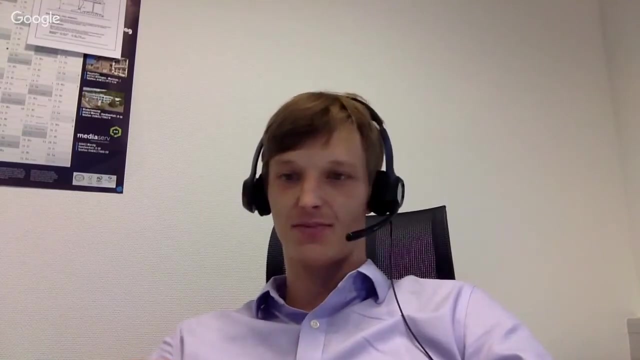 and more complex images, for example, in your work on one of our agents. response: use artificial stimuli. yes, do you think that the image content is important? oh, yes, it is. so that's what we observe. like doing it for, for simple stimuli, as I said also before, it's easy. yes, because you have really know the, the parameters. 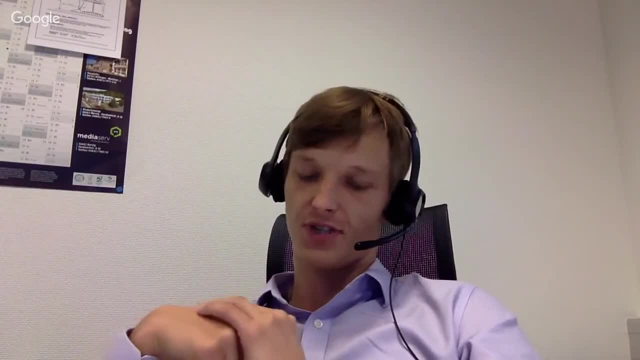 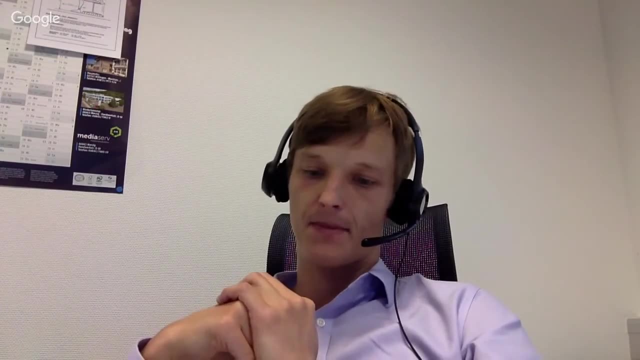 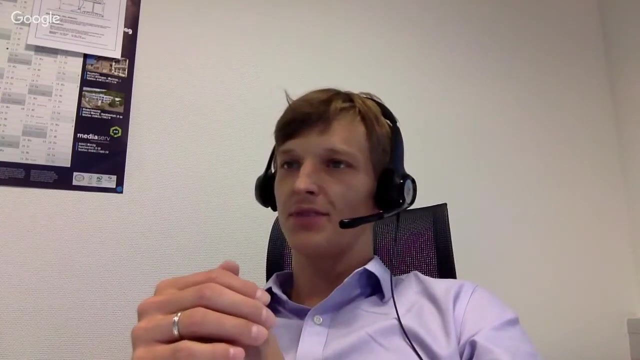 that you can vary, as for example, for the for this versions project, it was simple power with some kind of noise, and we simply vary the the, the two depth levels between which the transition happened. but I mean there is there is much more to it if you go to complex images. yes, so if you consider the video, people of. 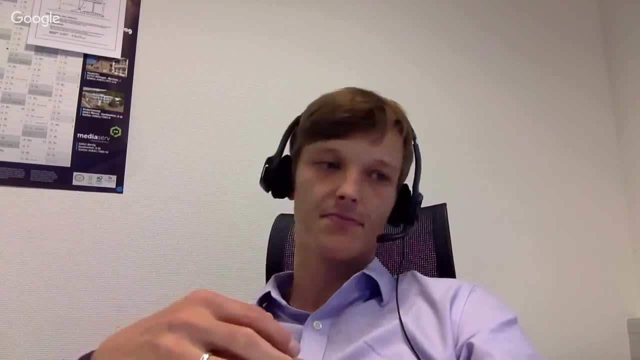 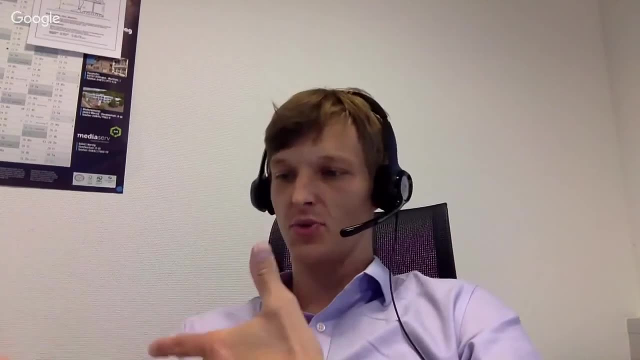 course, build some mental image of the entire scene, and you know it's not. they do also saccades or something that we didn't consider, because we have only patches that were aligned, so they were only patches that were aligned, so they were appearing at the same location on the screen, so they were not doing. 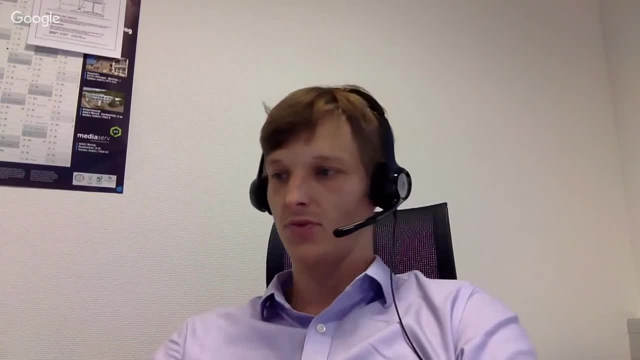 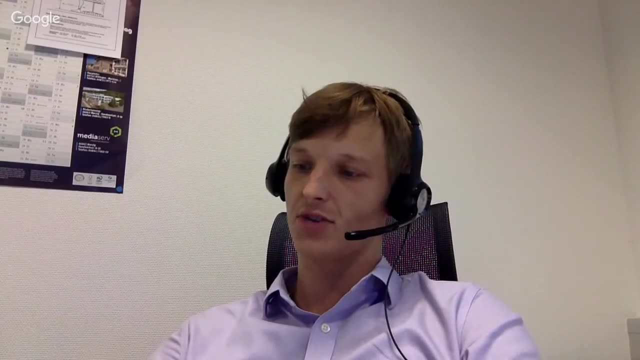 creasing gates. that would be another parameter that we could use in our stimuli, but then, of course, when you, okay. so those two simple experiments that we run, they're really nice and you know we can control it and build model and of course, I think where you're going is that you know, if you, if you try to apply. 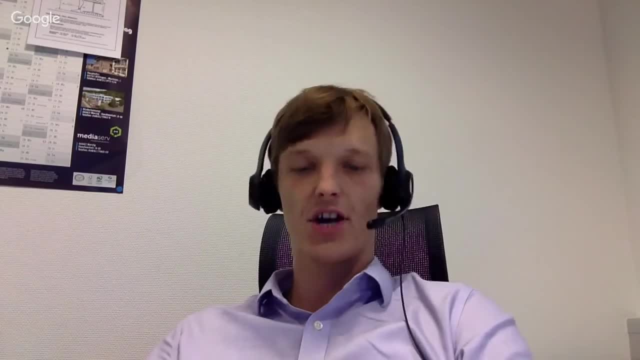 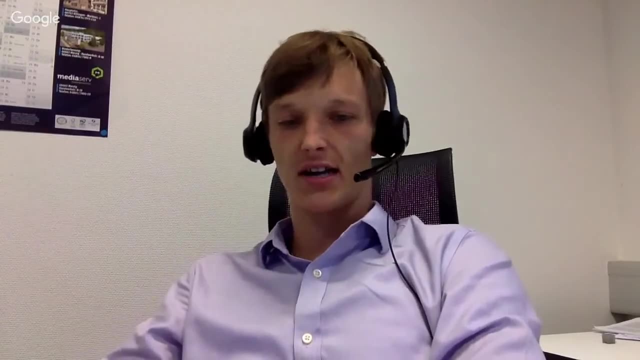 them to complex images, it's you find out that they are not accurate. yes, they are not. I mean you. they will not be accurate if you try to apply them to complex images. yes, they are not accurate if you try them to complex images. for example, if you try to apply them to total peugeot. 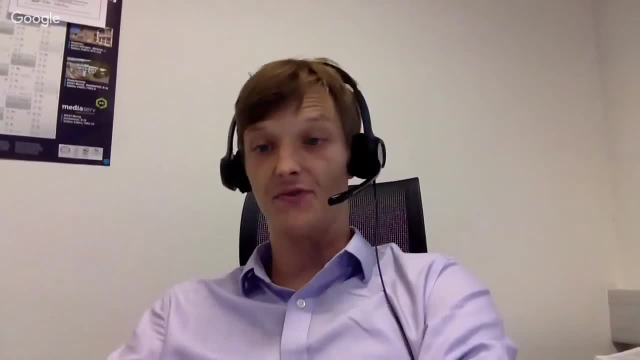 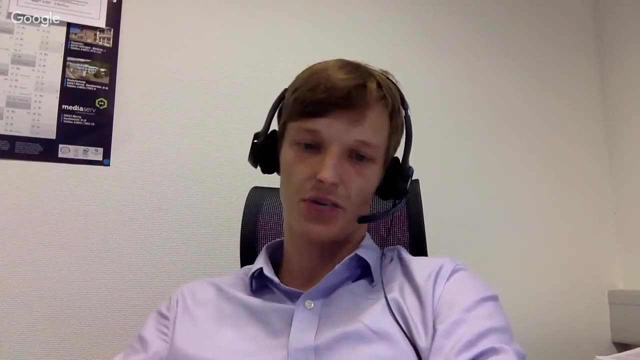 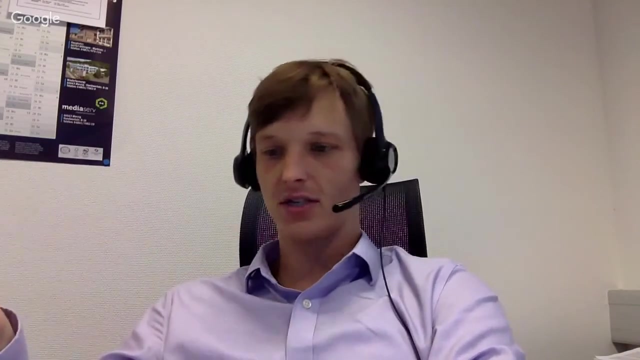 certain image, or if you try exactly what you can predict for complex stimuli. but this is something that you have to kind of, I think, live with. yes, if, if you do this kind of things, I I mean you can go ahead and do it for complex images, but those experiments become really hard. you can imagine that you 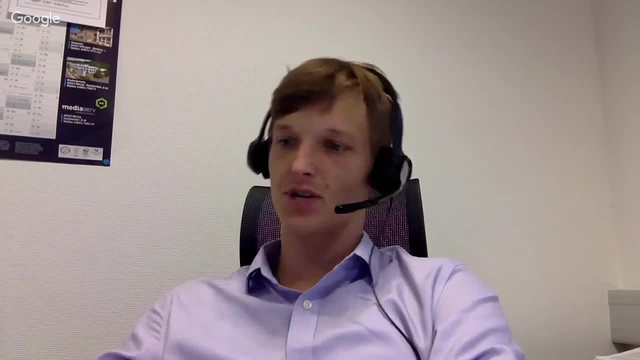 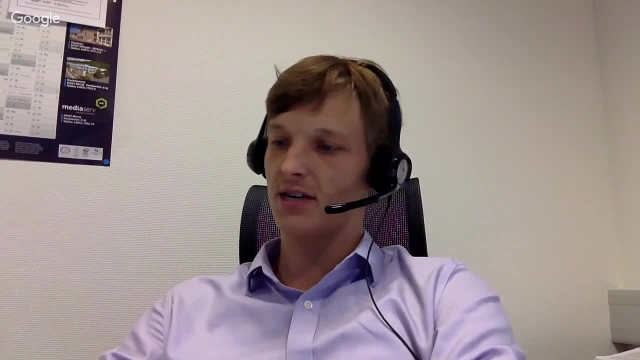 know, instead of having those patches, you play a video and you let people watch and you kind of want to even like use maybe some machining learning approach to to to build such models. but we tried some something like that also in the past. it's difficult, yes, but it's. 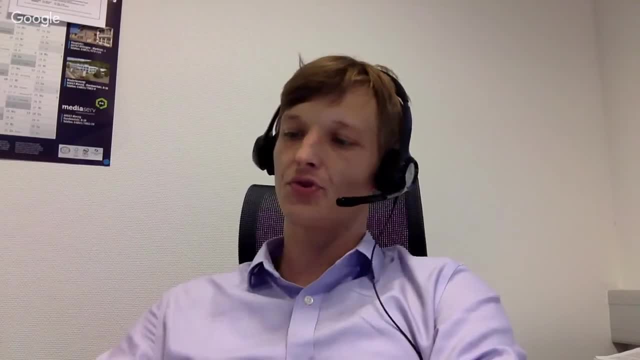 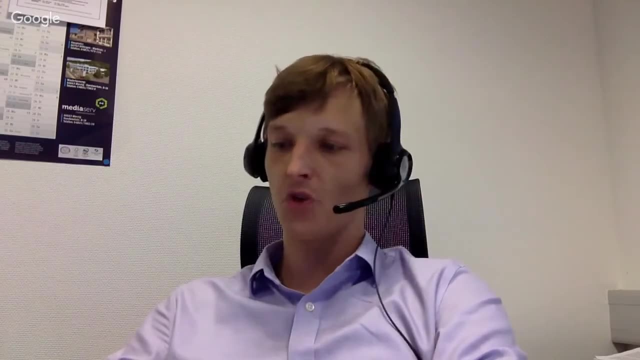 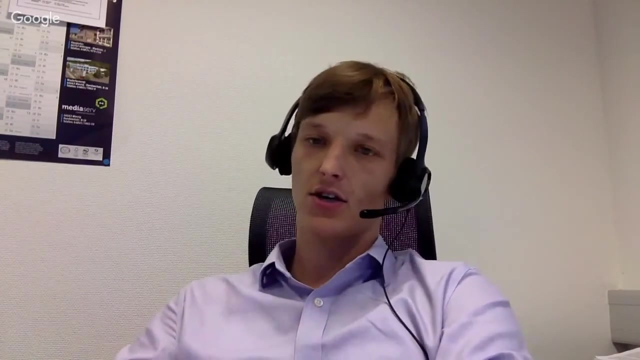 also true that that that you, if you do the modeling for a simple stimuli, you will have not the same performance of this model on the complex images. that's why i said that what is important in all those projects is that at the end you validate those models in the context of application. 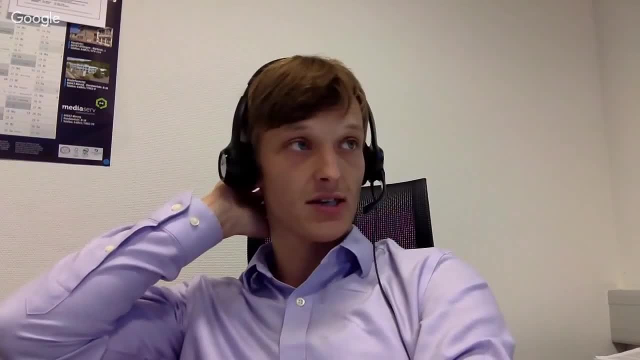 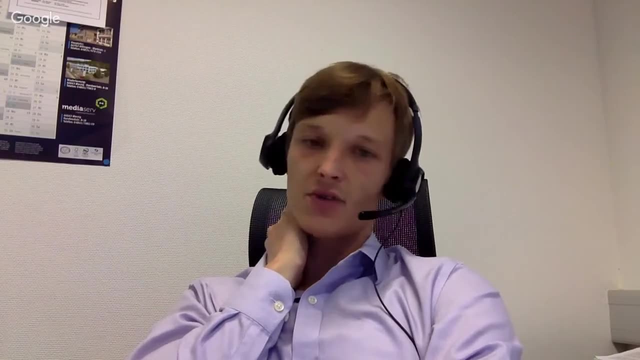 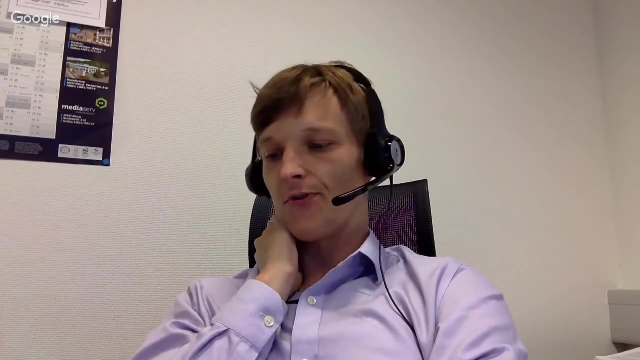 yes, so, for example, also this project on on predicting the on the disparity perception, we noticed that when we, you know, we we modeled this thing and then we were evaluating in the context of, of complex stereoscopic images, we noticed that as the number of, of of depth cues increases, so as you have more and more, 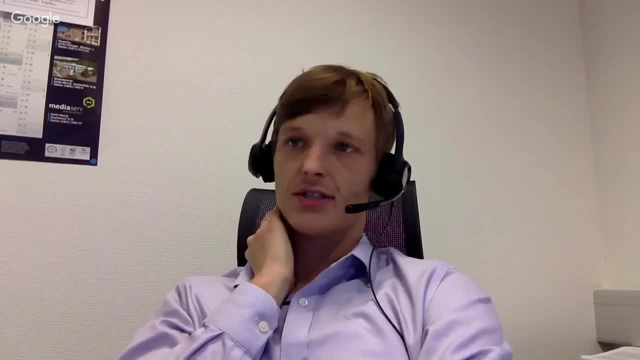 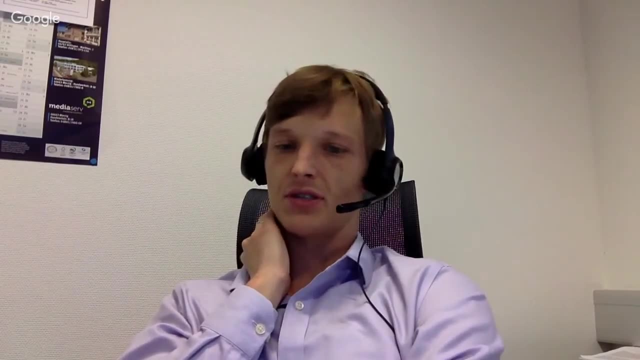 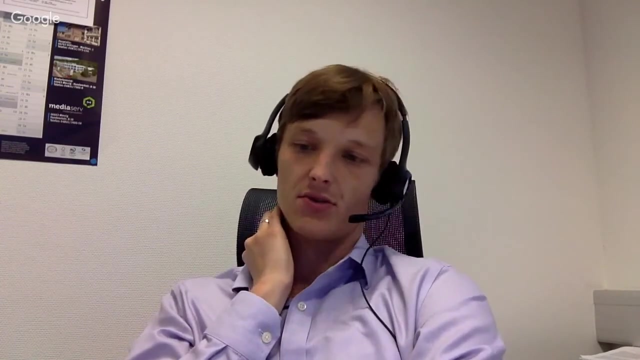 information, like shading, occlusions and things like that. the prediction of the model also deviates from the human responses. yes, but still, if you can show that your things correlate well and they're not too much of, i think this is you know. this is what we are essentially aiming for. yes, you know. 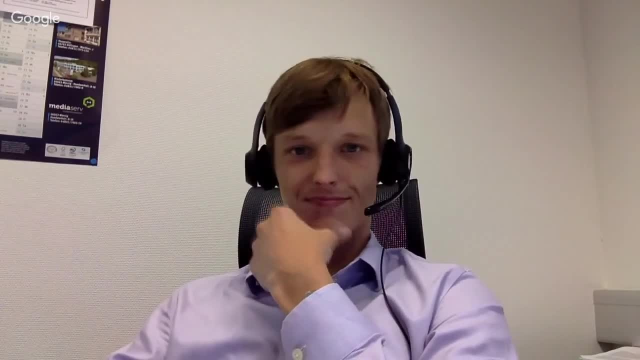 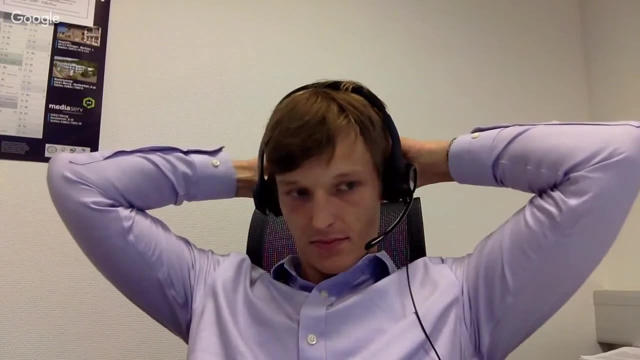 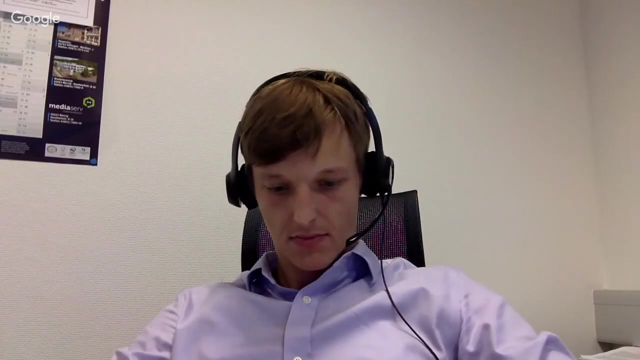 i didn't get the idea of just enough stereo. so basically reducing the disparity to support people that i'm not interested in- stereo by the model, but on the other side, with just enough parity, amount of disparity to do that perception, to have that perception, you have only a very 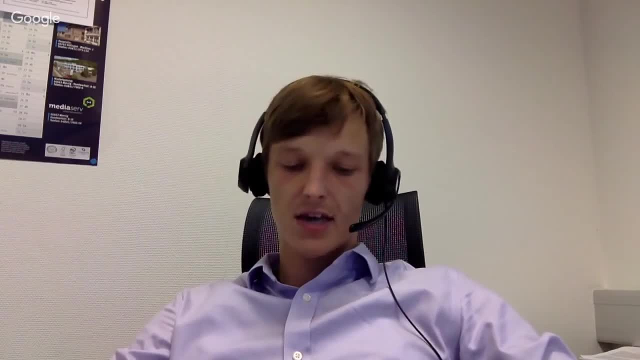 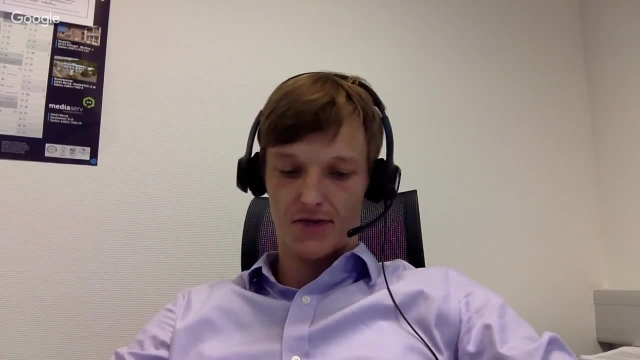 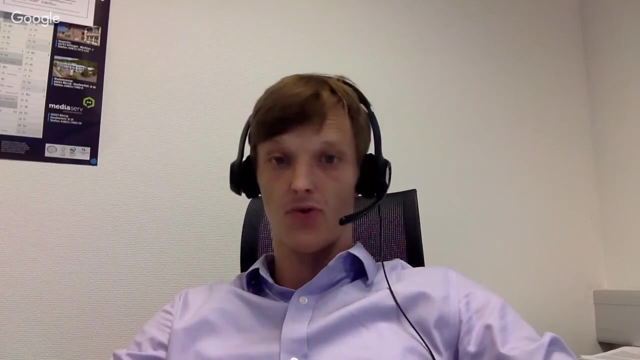 you cover only very little depth rating. yes, so so the idea was to you know, we know more or less what kind of signal people are most sensitive to in terms of depth, so we essentially were adding this information instead of some, for example, low frequency information that people are not. 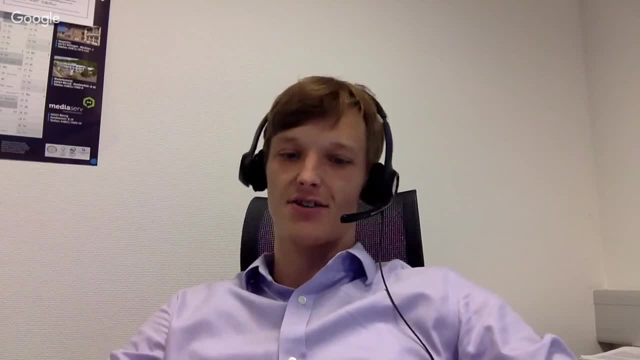 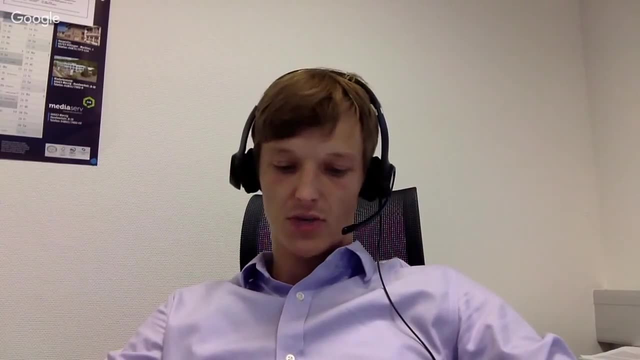 that sensitive. of course this doesn't convey the entire. you know that it doesn't give you the same impression. we did actually did some experiment where we, when we, where we ask people to, to compare our technique with the real stereo, yes, and we can show that we, you can largely reduce the overall disparity range.